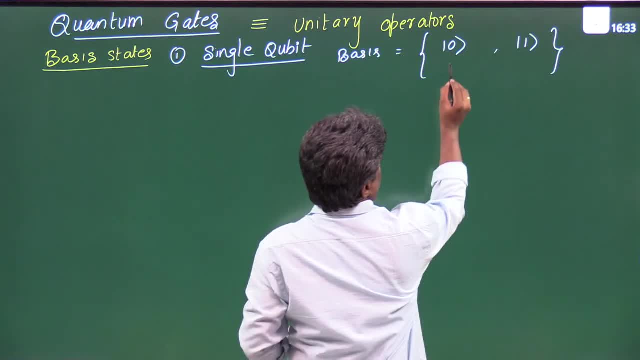 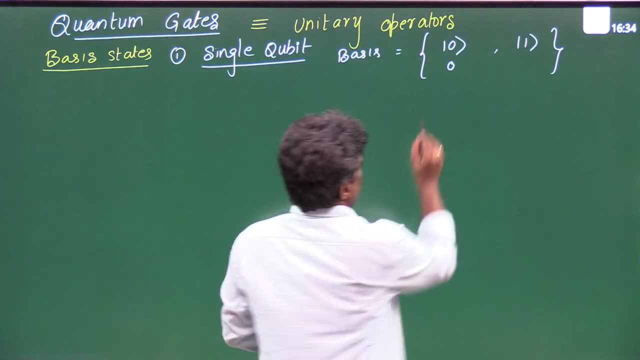 sc regarding advanced electronic technology. whenever you have this only one number, what you will take is two power zero into zero. So how much is it Zero? Please remember this value also. Okay, This is very useful. So that means binary notations. 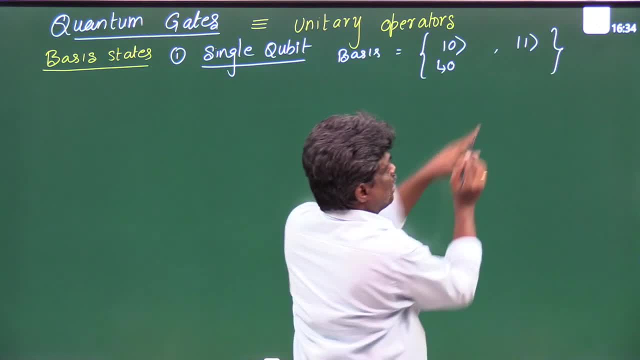 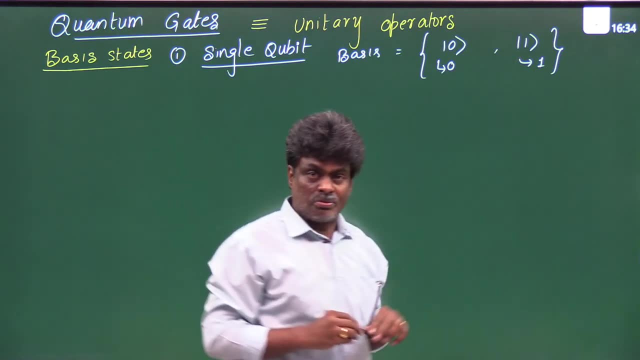 For example, here you have one. That means what? So two power zero into one. So how much is it One? So this notation is also very useful for gates. Please remember that. And after that: we have already studied about theustaities, So let's now have some to be learned about theustaities. 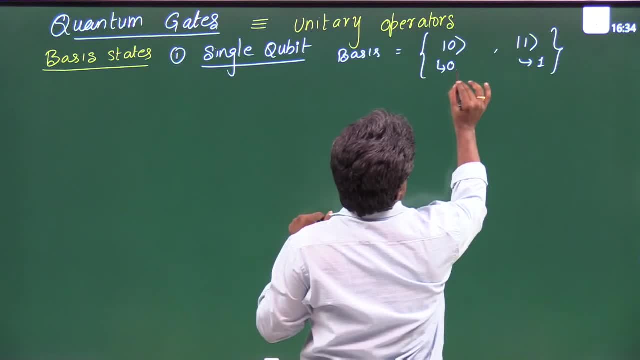 So let's have some to be learned about theustaities, And after that, we have already studied about theustaities. And after that, we have already studied about theustaities. discussed this: this is zero. state is nothing but one zero. okay, and this one. 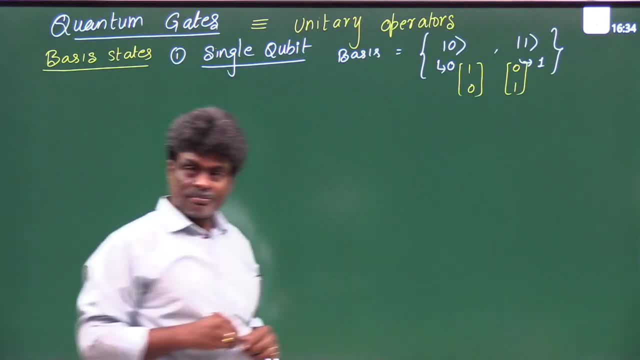 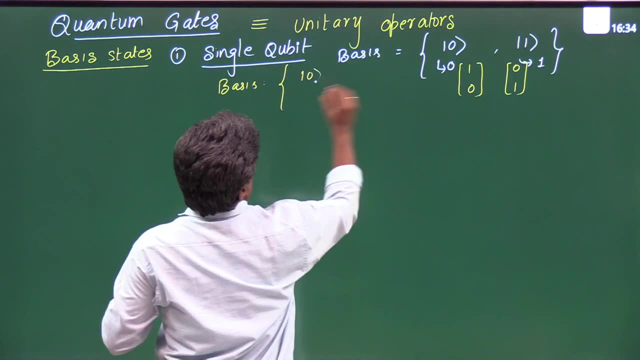 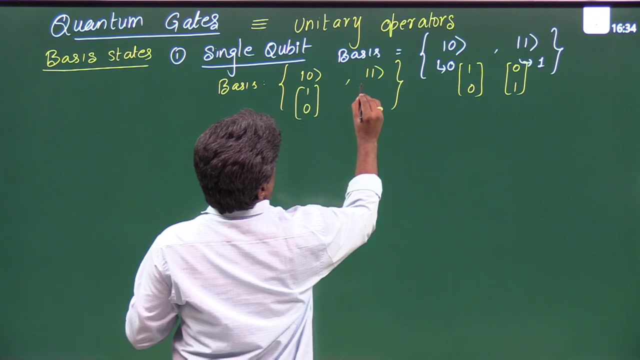 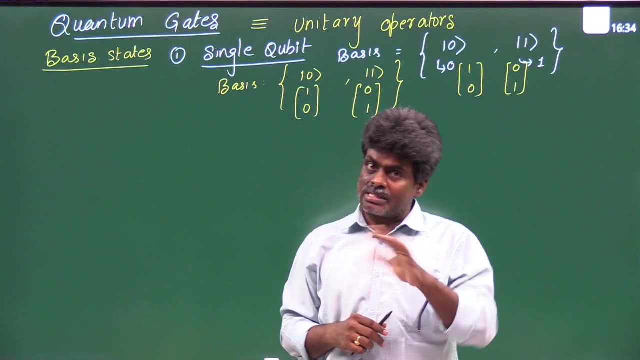 is nothing but a zero one. so here the single qubit basis states are simply zero and one one. second I am writing here, this is nothing but one zero. so, column matrix, and this is a zero one. and remember one thing: whether you are dealing with a single qubit, two qubit or three qubit, whatever may be, you just 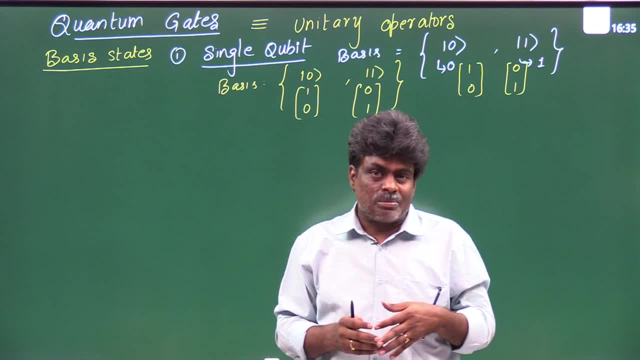 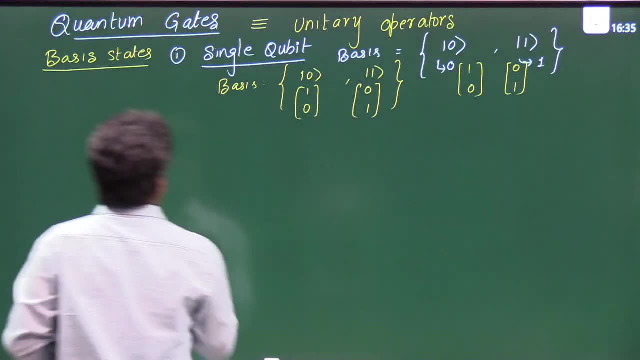 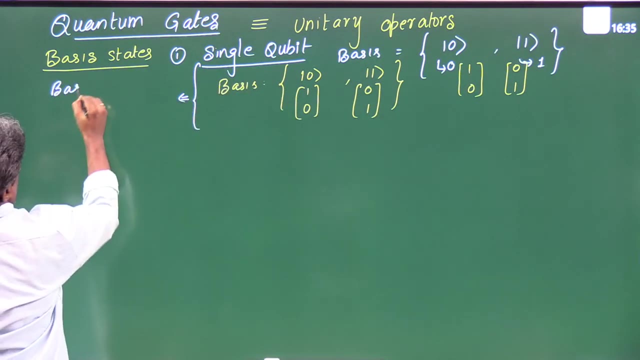 take all that basis and write as a columns, then you will get a identity matrix. so this is also most important point for the quantum gates, don't forget this. so what I am saying is, just write this basis as a columns. you, if you write basis as a column, then you will get a matrix called identity matrix. one, zero, zero one. 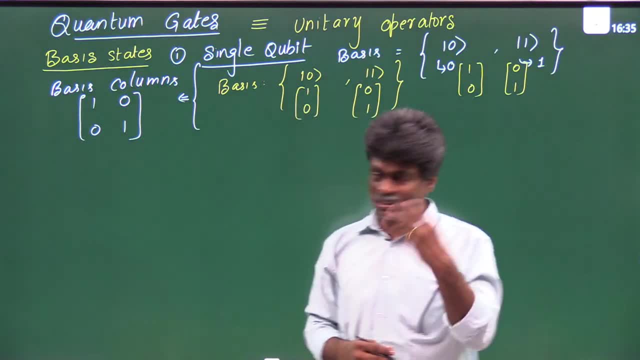 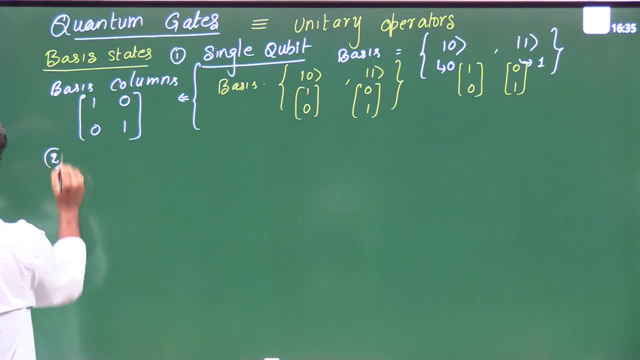 this is true for all the gates. two qubit, three qubit, whatever it may be. that's it. okay, this is about a single qubit. next let me explain here itself. two qubit, two qubit, basis states. okay, two qubit basis states here. first we are discussing basis states. 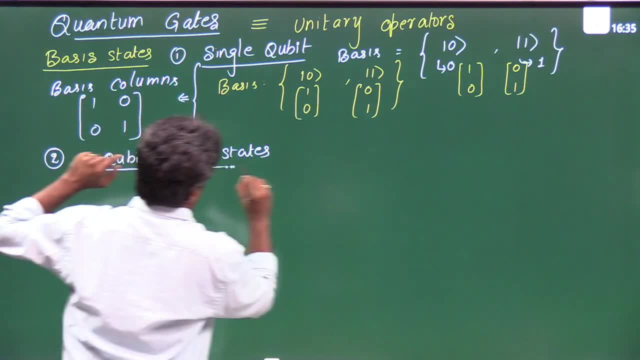 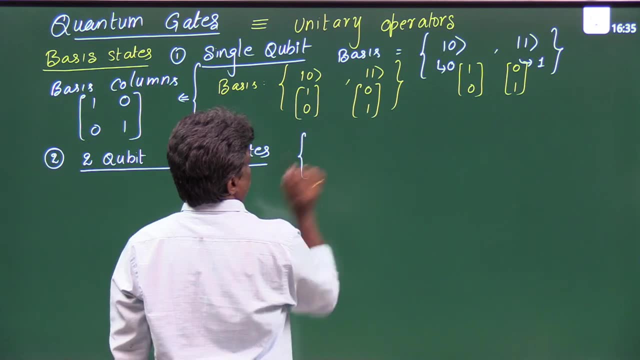 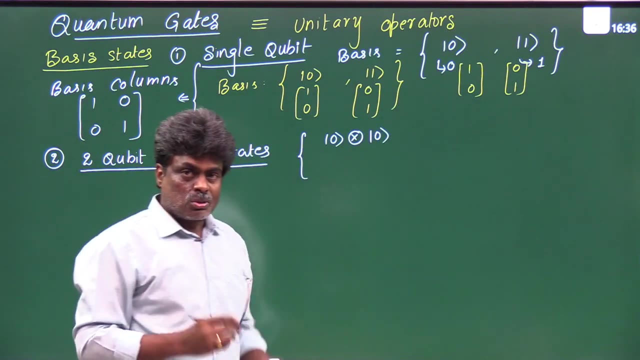 that's good. now what are two qubit basis states? don't get tension, it's very easy. so here, two qubit states are given by simply zero. single qubit, tensor, product zero. so here already you have two single qubits, zero and one. now you have two single qubits, zero and one. so here 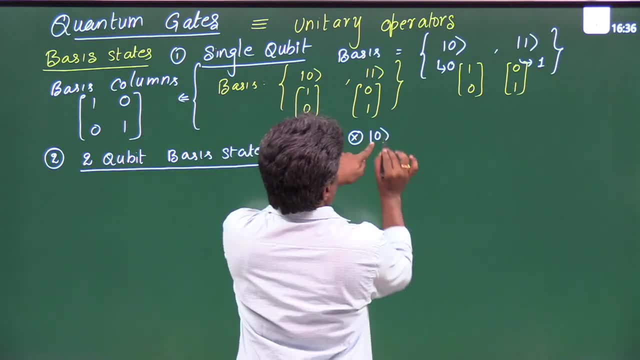 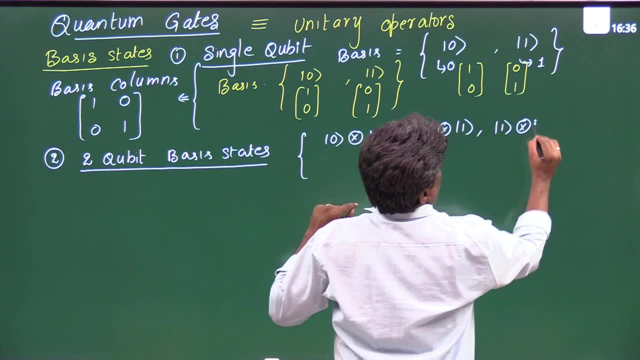 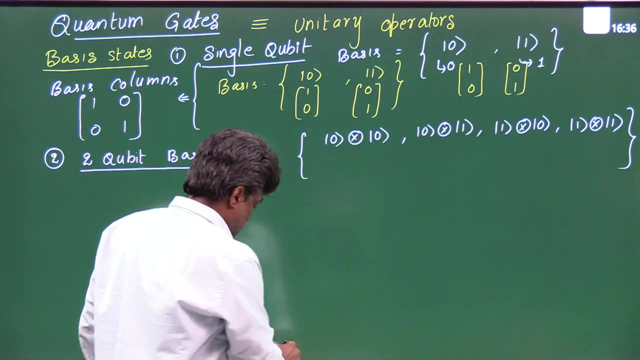 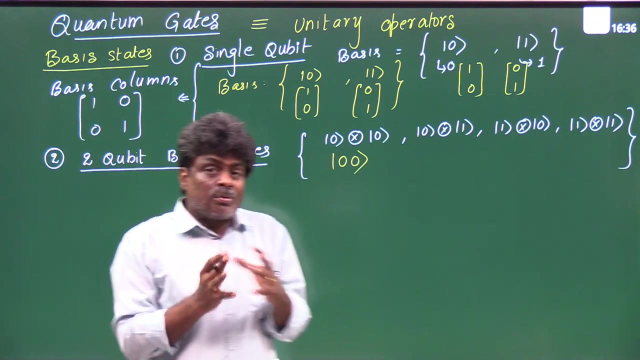 just make a combination: zero at a tensor product with zero and the next one a zero. here the tensor product one and here one tensor product zero and here one and the tensor product one. if you see this notation, we will write this tensor product as a zero. zero now onwards, whenever you. 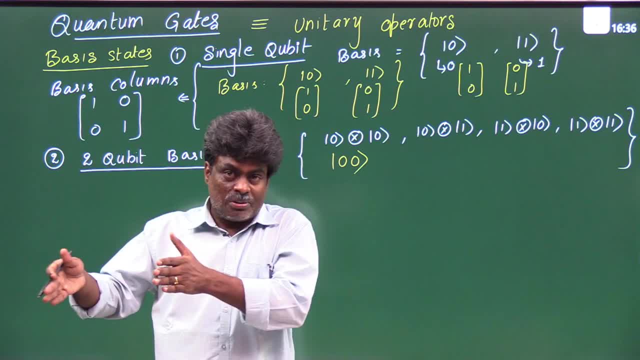 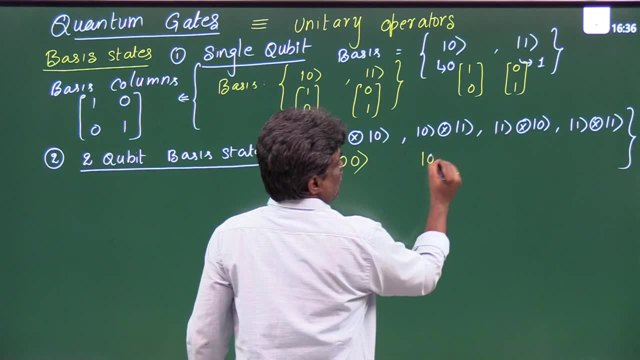 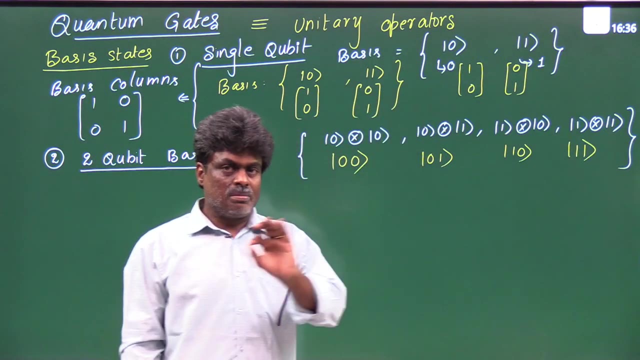 have a three tensor products: zero, zero, zero. that is nothing but a state of zero, zero, zero, 000, something like that. so you can write like this: no issue, and this is nothing but a 0, 1, and this is nothing but a 1, 0 and this is nothing but a 1, 1. so quite similar to that. 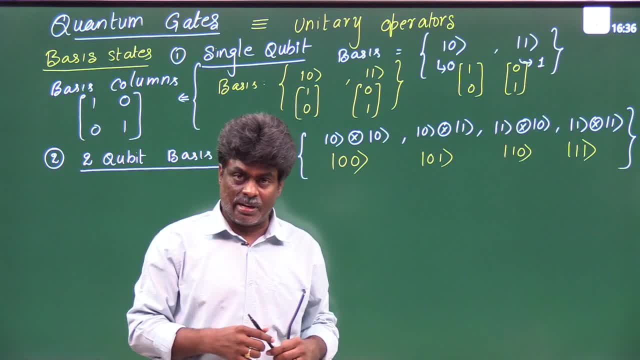 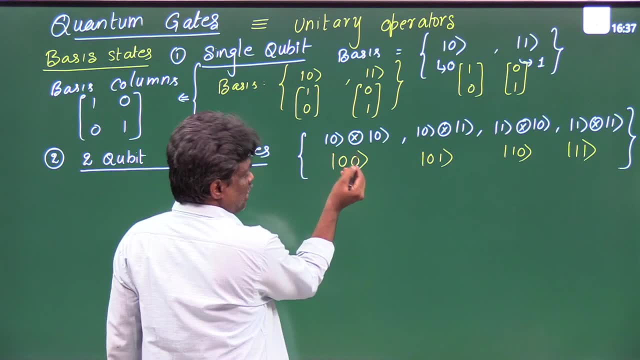 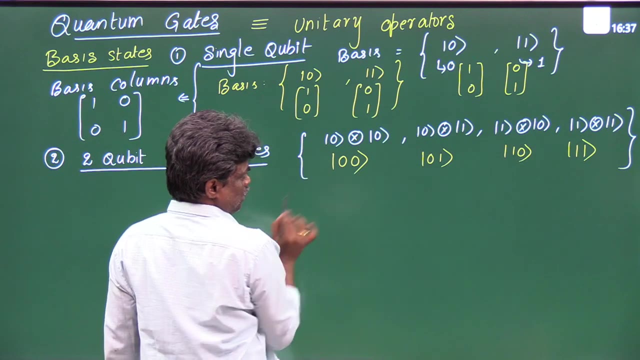 digital electronics. whatever we have done in the digital electronics. please see this one, how you will write this binary notation: 2 power 2 power. yeah, 2 power 0 into 1. i mean 2 power 0 into this and 2 power 1 into this. so how much it is? 0, all right, and this one. i hope you know this. 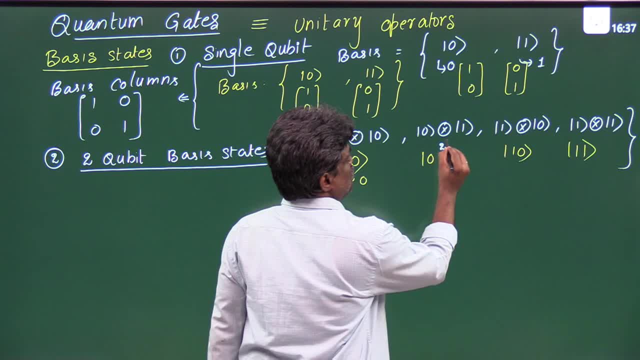 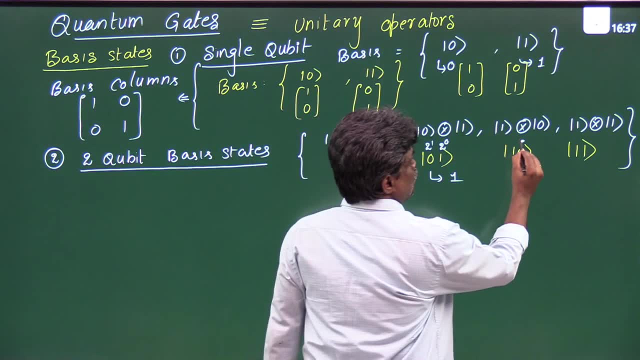 shall i write: this is a 2 power 0 and this is a 2 power 1. can you please tell me what is its value? 1? and here it is a 2 power 0 and a 2 power 1. if you see that binary notation, binary to decimal. 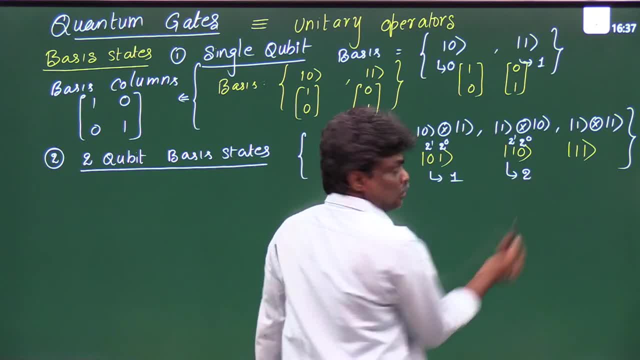 something like that. so this value is equal to how much 2. how you will write: 2 power 0 and 2 power 1, and this is a 2 power 0 and this is a 2 power 1 and this is a 2 power 1. 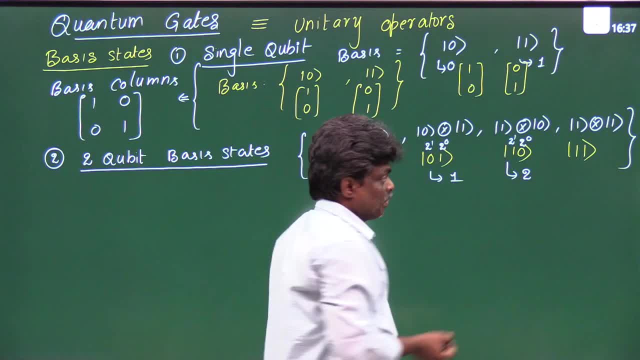 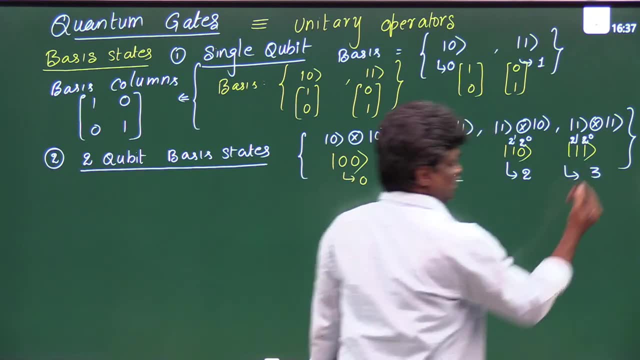 0 into 0, plus 2 power 1 into 1, and can you please tell me? this is a 2 power 0 and this is 2 power 1, so how we will convert? this is equal to 3. now carefully observe: it is a 2 qubit basis states. 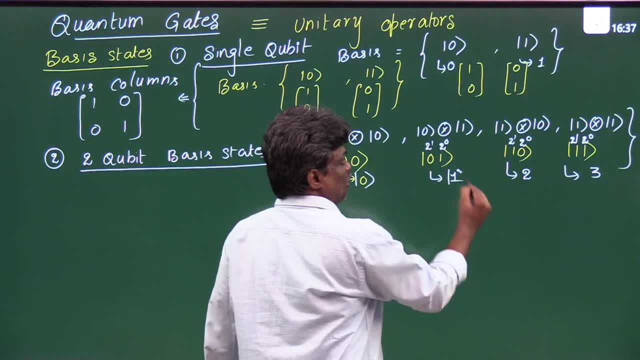 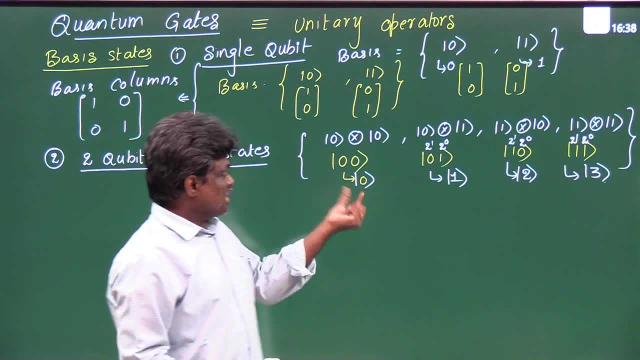 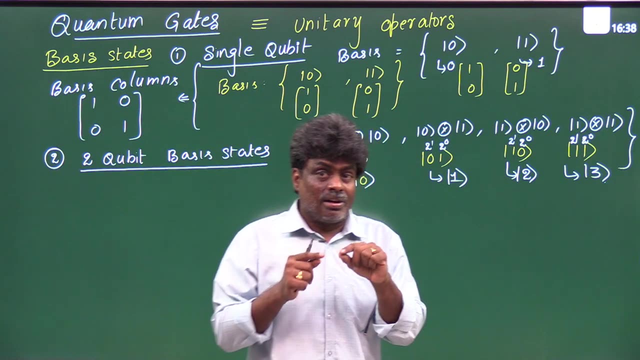 sometimes you will represent as 0, 1, 2, 3 also don't get tension. so this is: 0 is nothing but 0, 0, 1 is nothing but 0, 1, 2 is nothing but 1, 0, 3 is nothing but 1, 1. if you are writing a 2 inputs, for example, you go to digital electronics, you have 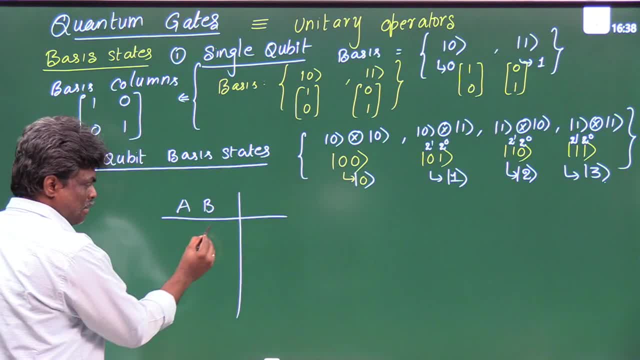 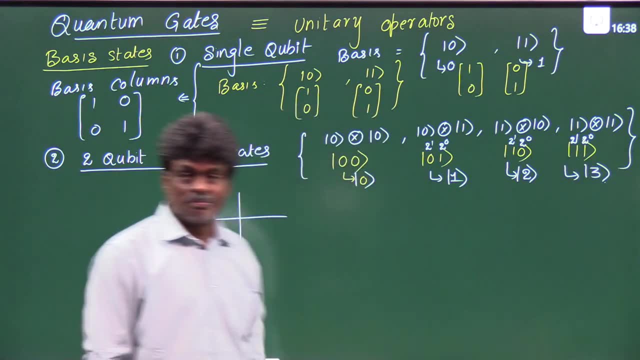 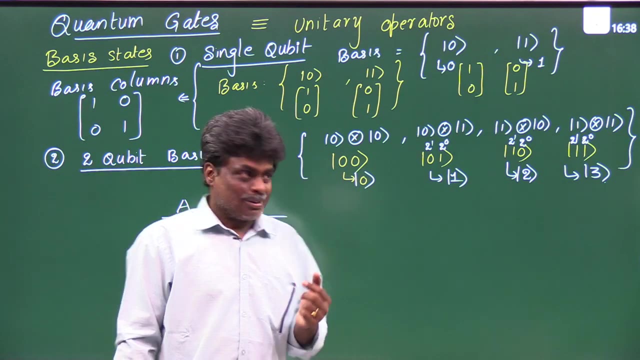 2 inputs a, b: i hope you remember this: 0, 0, 1, 0, 0, 1, 1, 1. the same thing. i hope now you can guess what will happen for a 3 qubits basis states. so 3 qubits, what you have taken, 0, 0, 0, like that. how? 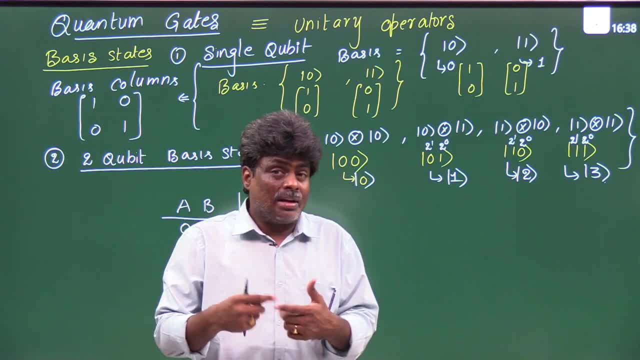 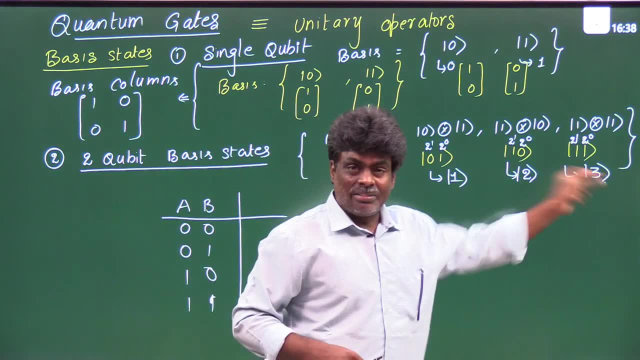 many. you will get them: total 8. but the binary value, what is that? a decimal value? what is that? 0, 2, 7. so here we have 0, 2, 3 and let us see what is that 3 qubits. also don't write, just listen, please. 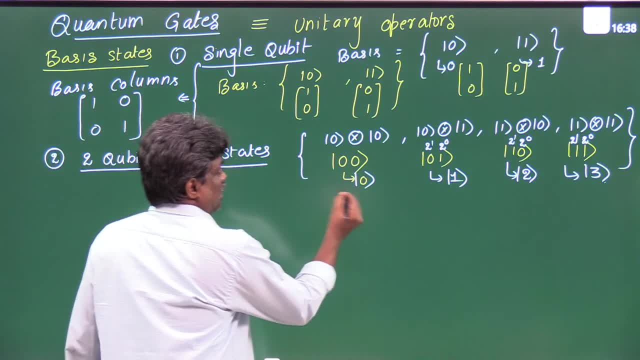 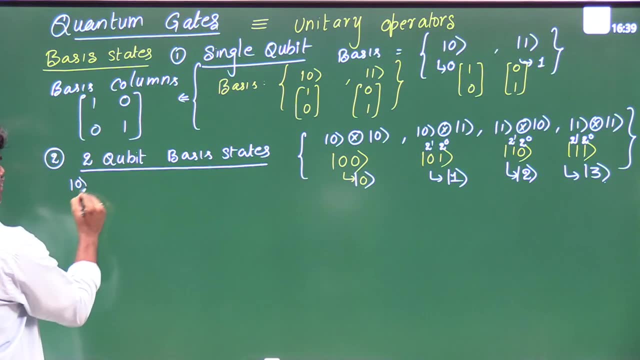 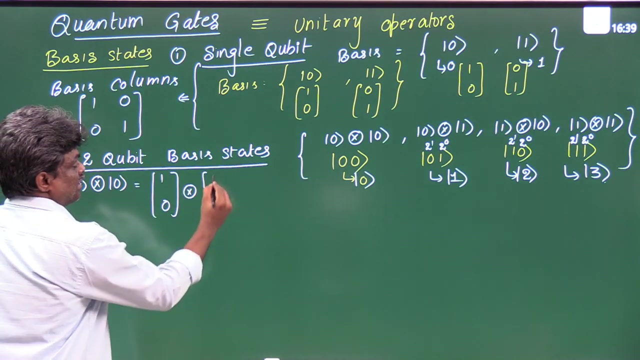 okay, so then one minute, how to find this tensor product. let me write this state. so the tensor product is given by 0. tensor product 0: here, these, these two, what is the tensor product of these two? it's very simple, right? this is 0. state 1: 0. now tensor product with a: 1: 0. are you listening? yes, please listen. now take this 1. 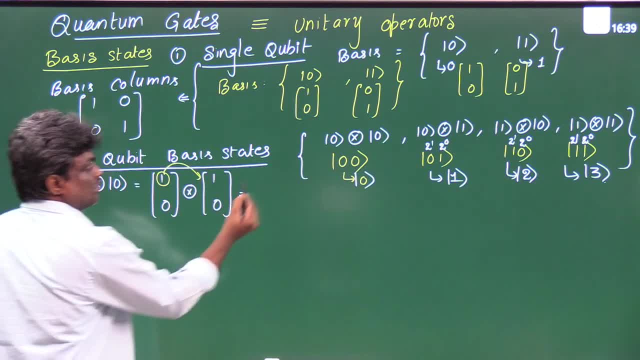 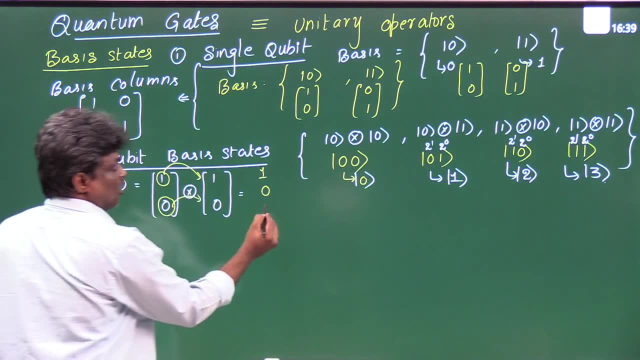 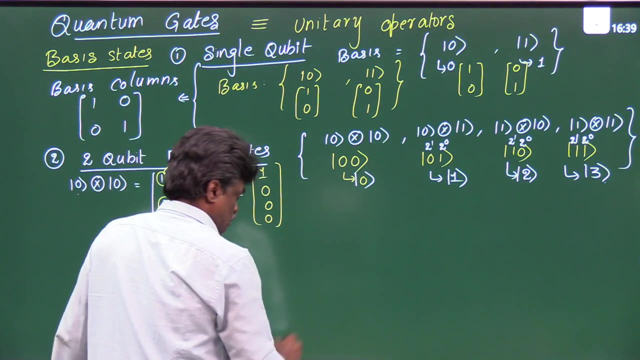 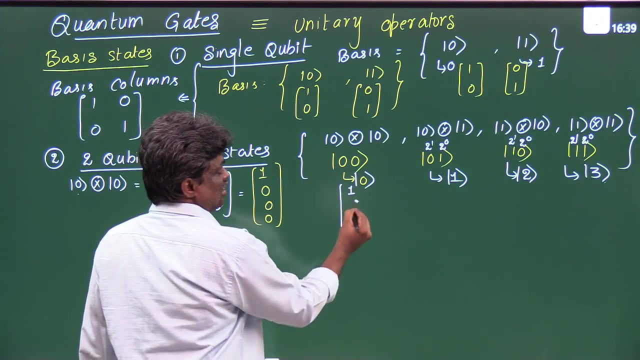 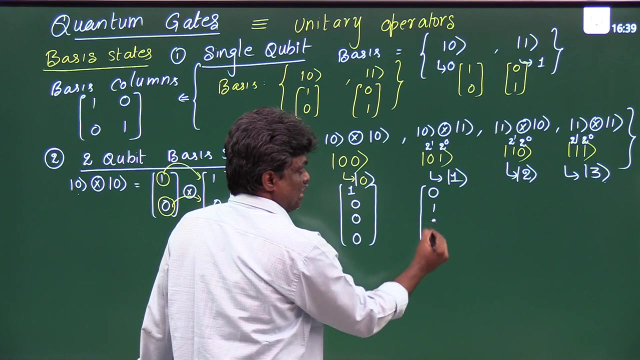 and multiply with this entire column, how much 1 0. next, take this and multiply with the entire this column, how much 0, 0? i hope you understand. so if you write the first basis state, the first basis state of a 2 qubits, that is, a 1 0 0, 0, shall i write similarly? similarly, 0 1 0, 0. can you please guess? 0 0 1 0. 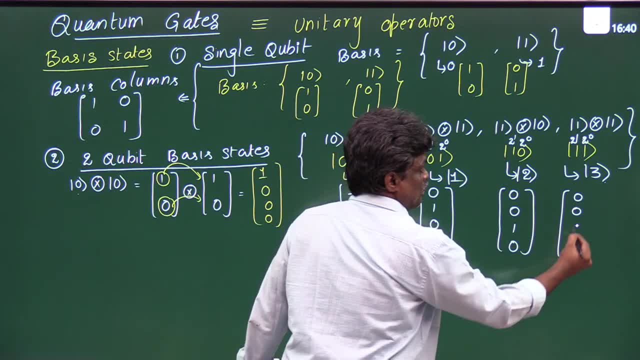 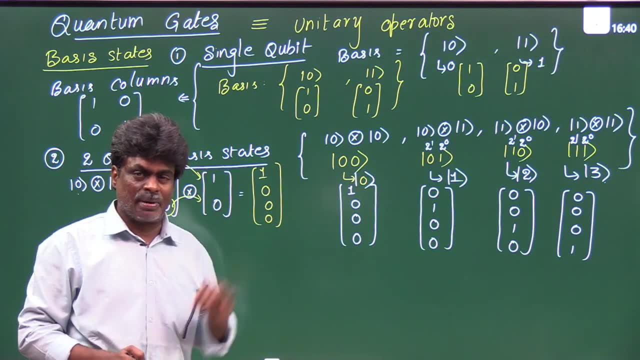 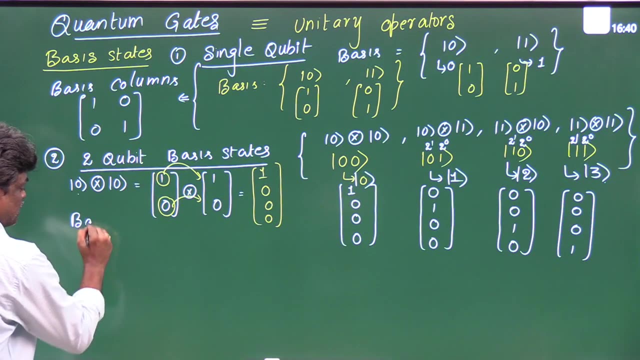 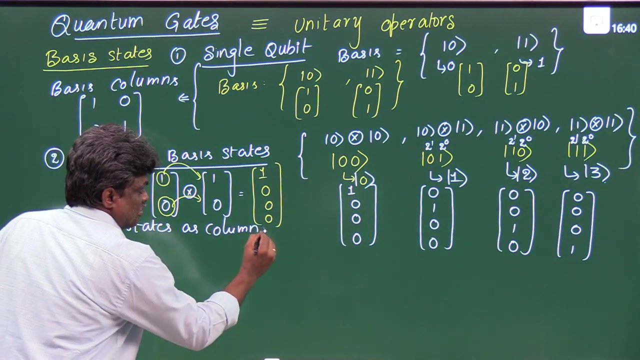 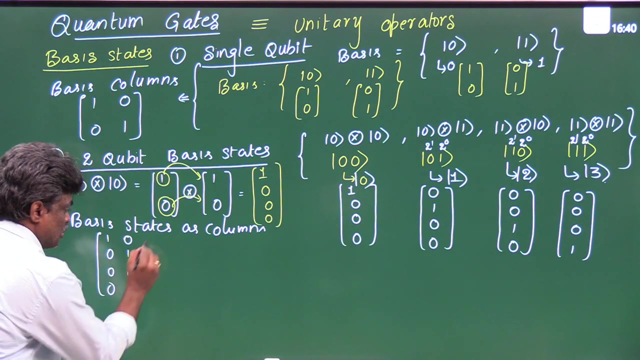 and here: 0 0, 0, 1. a few minutes back, i told you one thing. this is a very important in quantum gates: if you take all these basis states and write it as a column, that means basis states, basis states as columns- what you will get. so you will get here: 1 0, 0, 0 0, 1, 0, 0, 0 0 0, 1, 0, 0, 0 0 1. 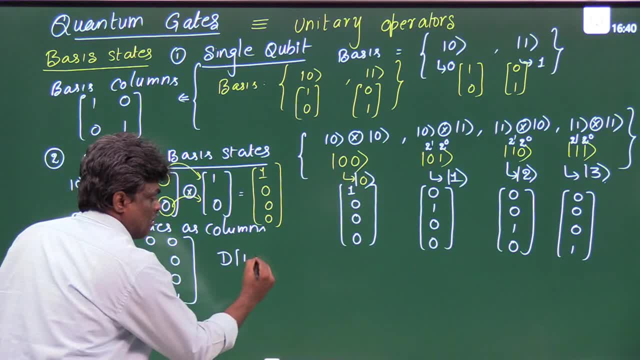 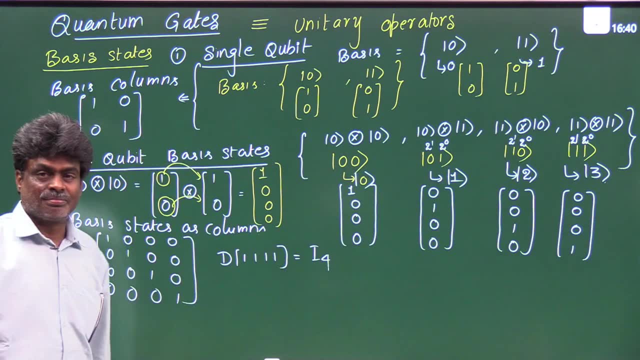 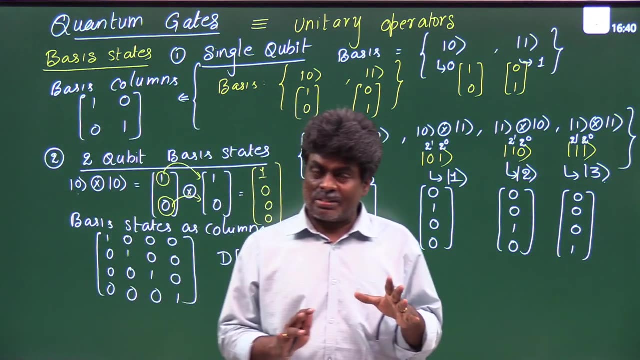 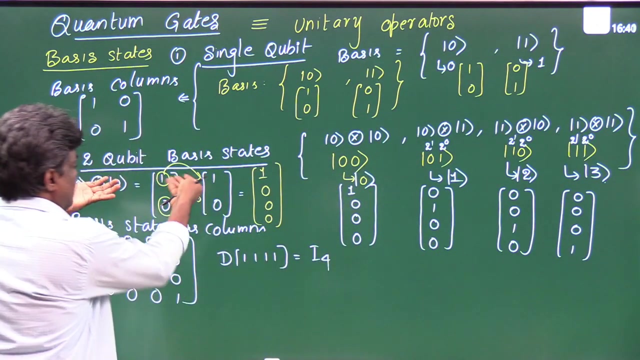 this is the diagonal matrix of diagonal elements- four ones. so this is nothing but i4. so whether it is a two qubit states or three qubit states, all the basis states: if you write as a column, you will get identity matrix. don't forget this. now can you please write similar to: 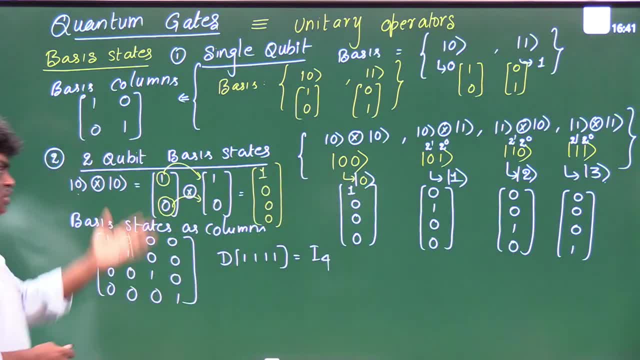 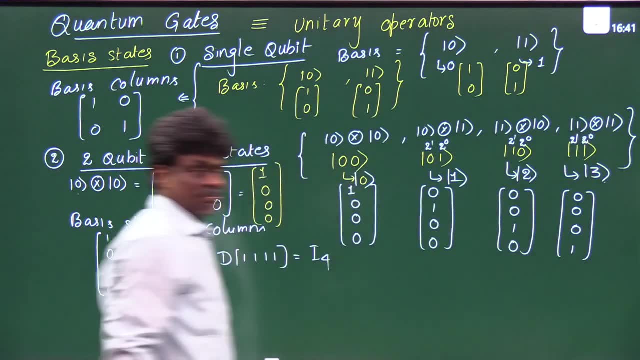 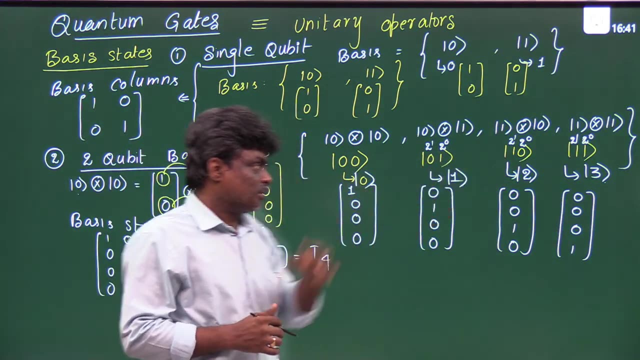 this: what are three qubit states? yeah, do it yourself. try then what you will get here: zero, one, two, three, four, five, six, seven. because already you know some knowledge about the digital electronics. that's why i'm giving this notation also, so that's why you won't. 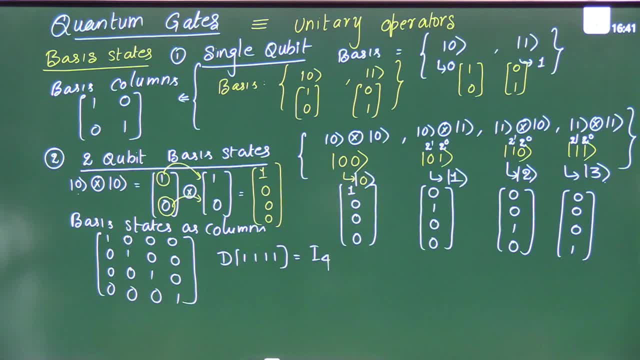 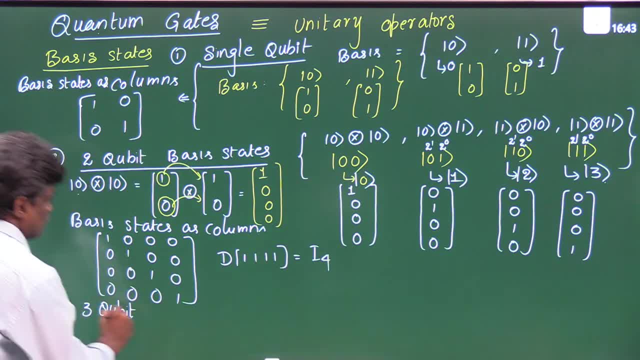 here you please try yourself. this is three qubit qubit qubit. three qubit basis states. three qubit basis states. three qubit basis states. try to write yourself, you will get interest. three qubit basis states. try to write yourself, you will get interest. three qubit basis states. try to write yourself, you will get interest. otherwise, simply copy no use because you. 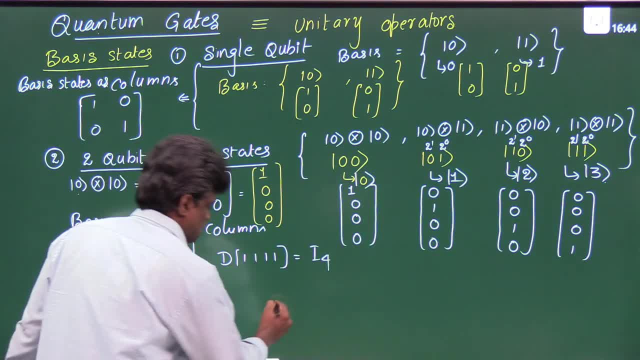 otherwise simply copy no use because you otherwise simply copy no use because you will forget easily, will forget easily, will forget easily. so because we won't practice, because we are so, because we won't practice, because we are so, because we won't practice because we are not writing for writing any exam on this. 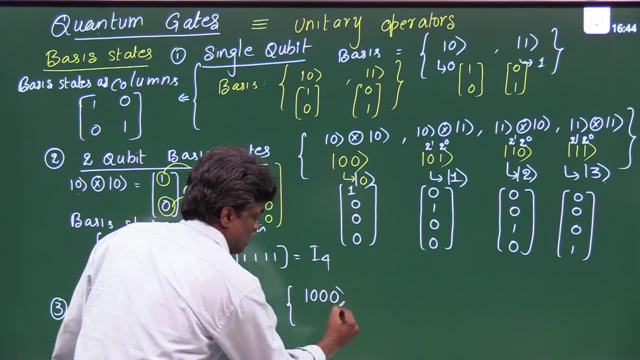 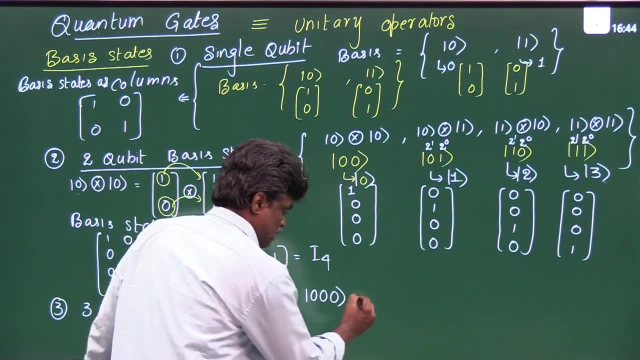 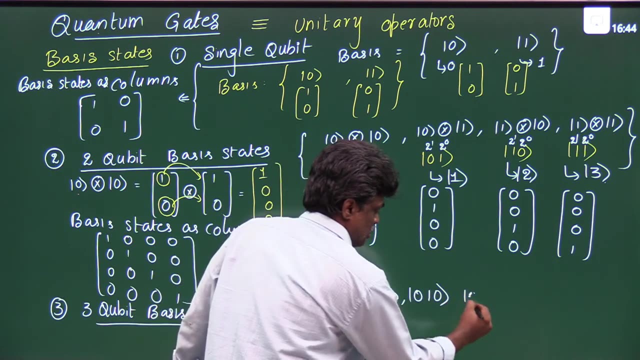 not writing for writing any exam on this. not writing for writing any exam on this. i can write directly here: 0 0, 0. i hope you know in digital electronics and binary system how you will write the same thing. you can write zero, zero, one, zero, one, zero, zero, sorry. 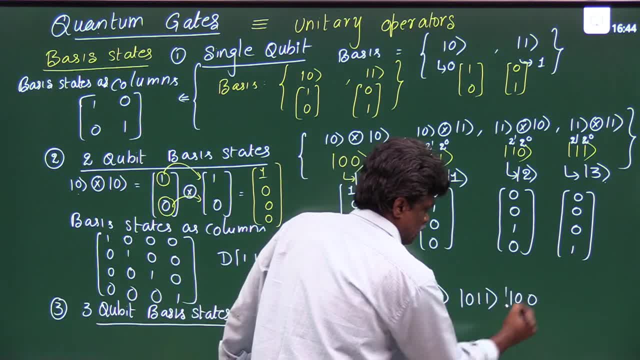 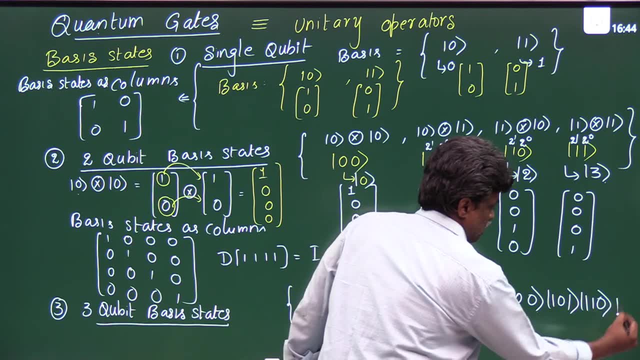 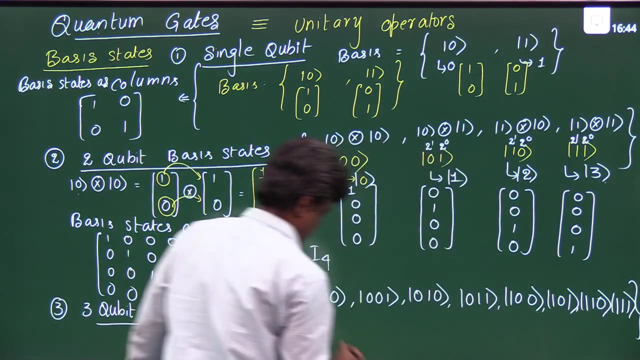 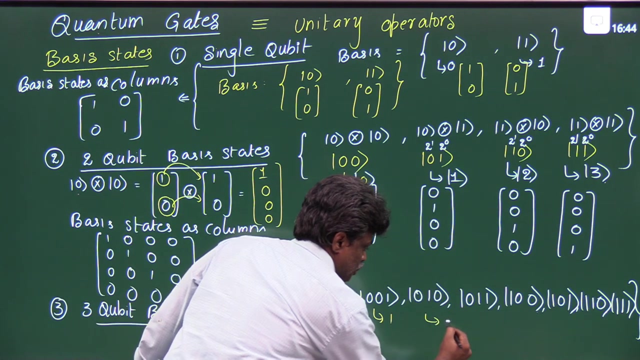 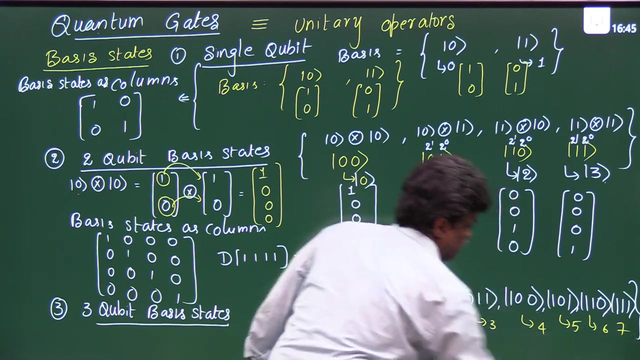 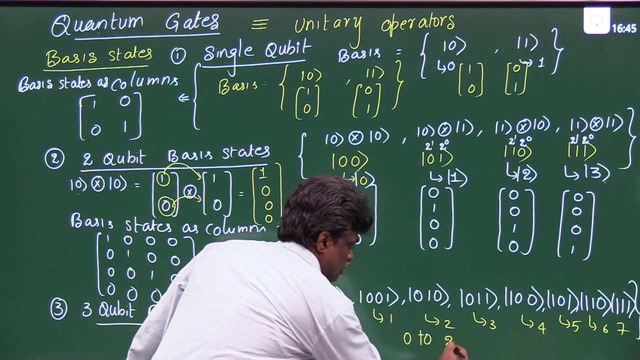 zero one, one one zero, zero one, not one one zero one one one zero and a triple one. so i hope you understand what i'm saying. this is nothing, but you please try yourself. zero value one, two, three, four, and this is five, six and seven. so your base states are from zero to two power three minus one. 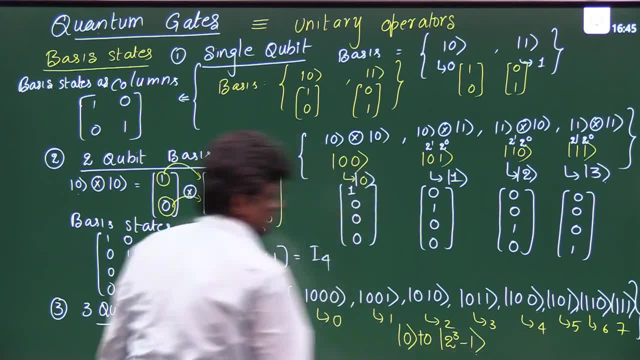 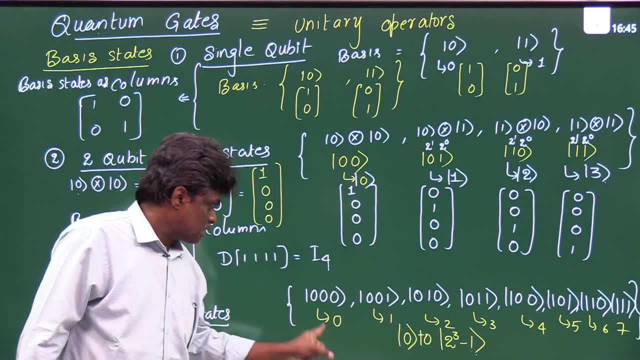 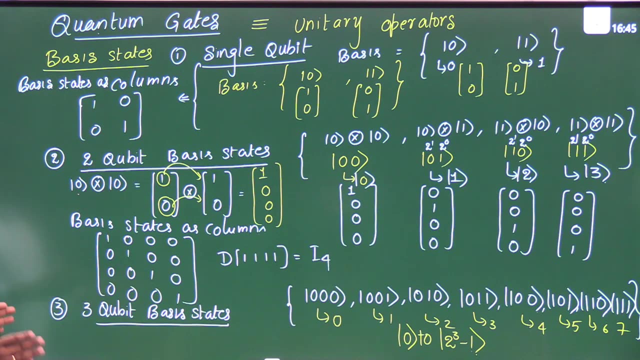 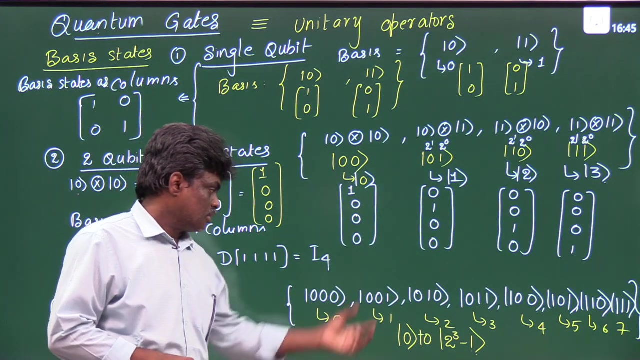 from where zero to two, power three minus one. if you are interested under this, please write this column matrix. okay, so better, because first time you are learning, the better to write a complete thing here. you will get a column matrix: 1 0, 0, 0, 0, 0, 1, 0, something like that, and if you combine all these things, 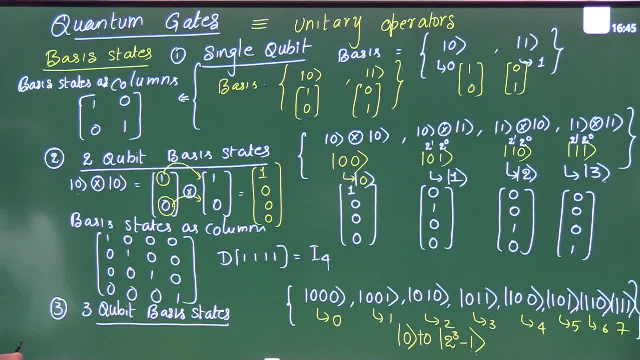 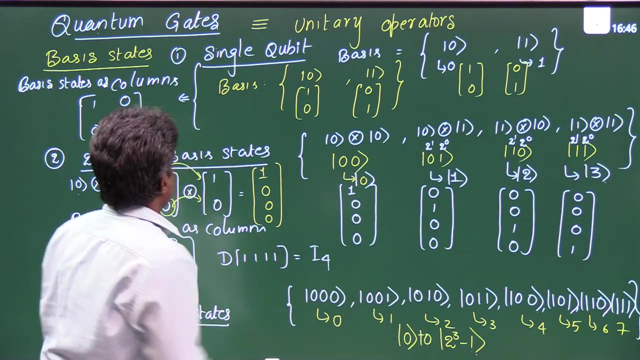 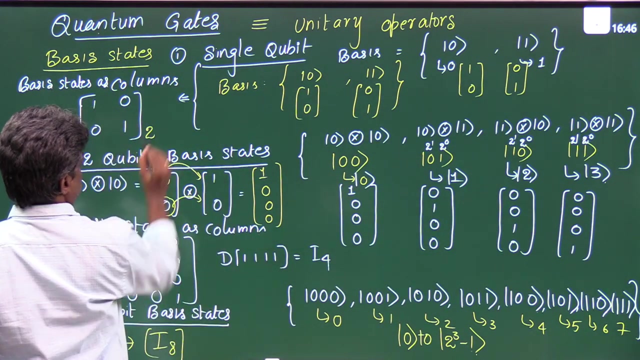 again, you will get a identity matrix of all these ones. the호�s 8, so here you will get i8. yeah, so in case of this, a single qubit, qubit basis states, we have here i2, and in case of two qubit states, we have i1, and in case of two qubit states, we have i2. and in case of 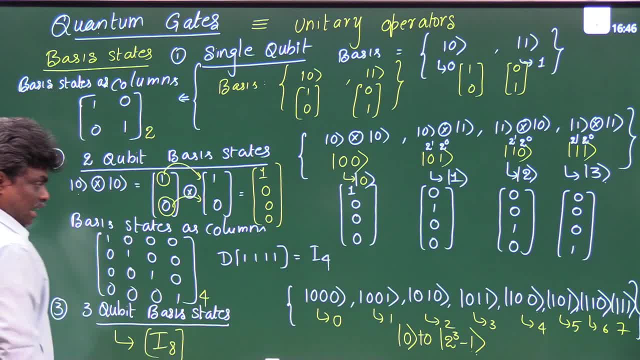 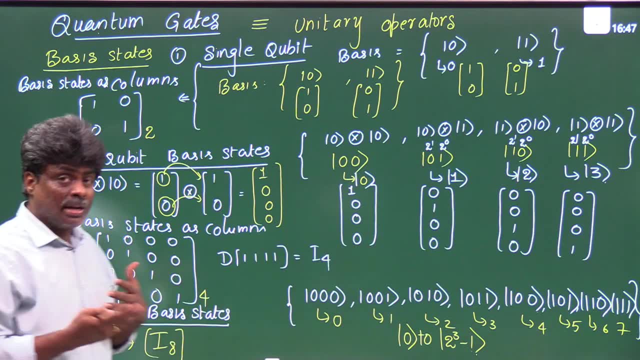 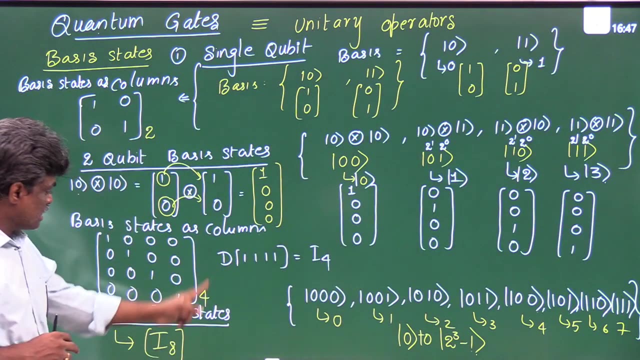 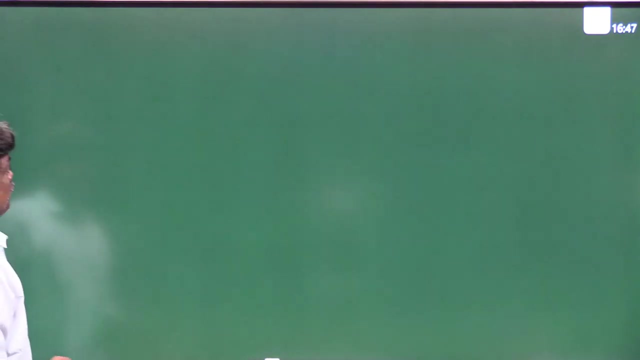 four and three qubits, we have i8. so this identity matrix is a very important and you, if you want to know the nature of that quantum gate and what is its a function, so what it will do, so that will be observable from this identity matrix. so be careful, ready, yes, now let us start this. a single. 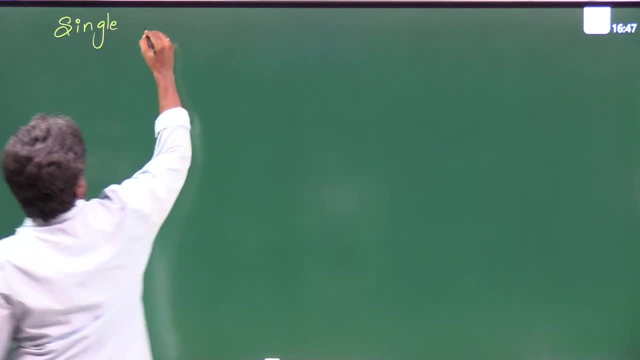 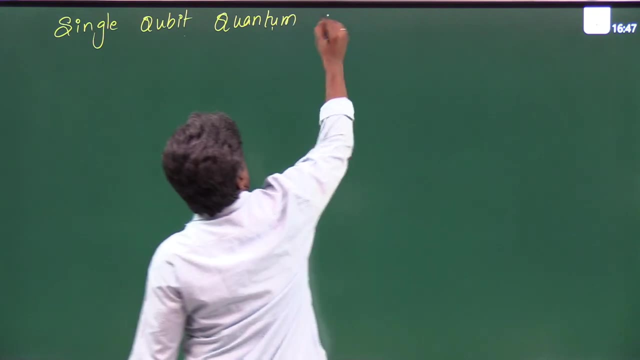 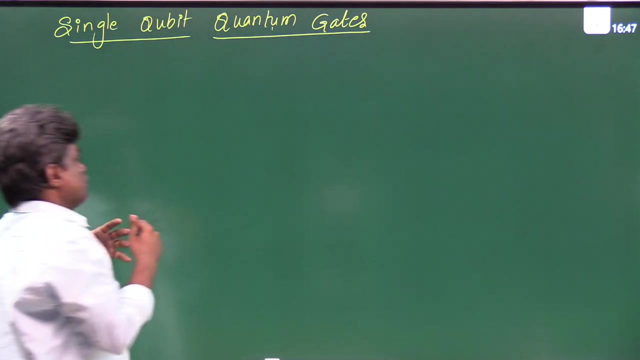 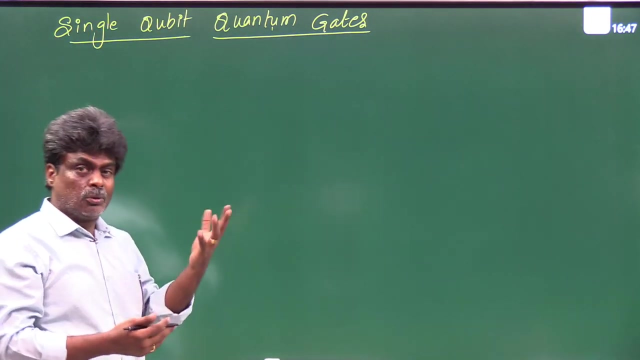 qubit state, sorry, single qubit, quantum gates, quantum gates. so already we understand what is what is meant by basis states, what is meant by basis state and how to write the basis states corresponding to single qubit and two qubits and three qubits. now let us go to quantum gates. i already inform you this: quantum gate is nothing. 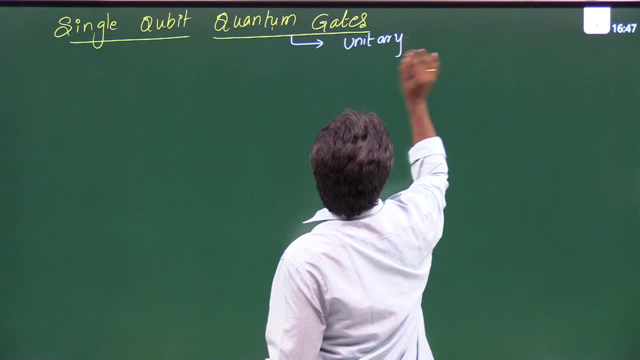 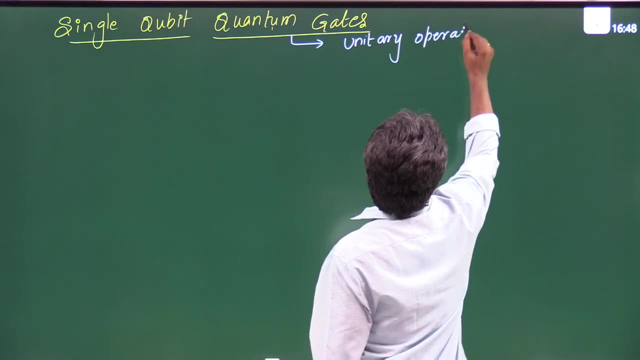 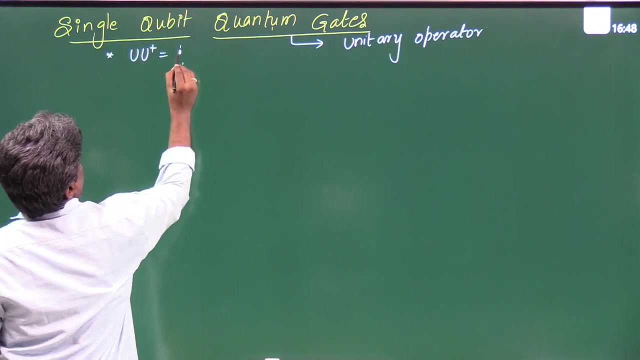 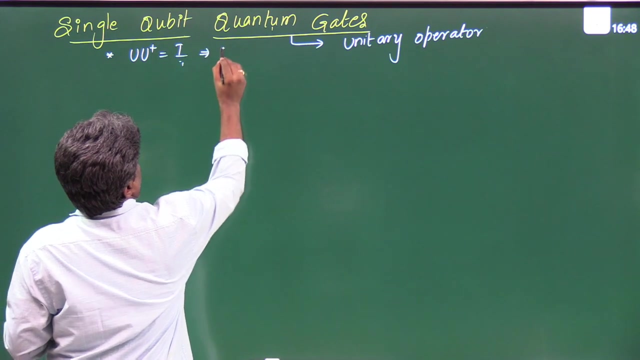 unitary operator. every quantum gate is represented by unitary operator. let us see the properties of unitary operator once. i hope you know u? u dagger is equal to i. that's a unitary operator property. that means what? now? u inverse is nothing but simply u? dagger. 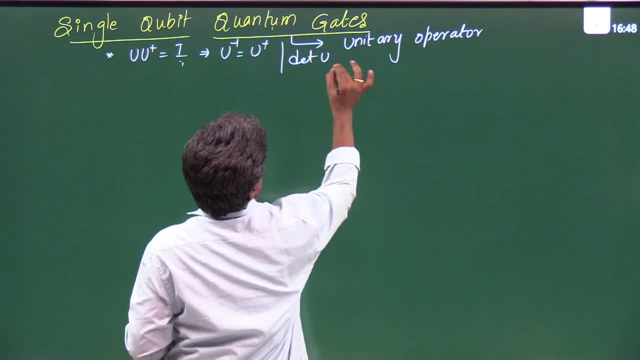 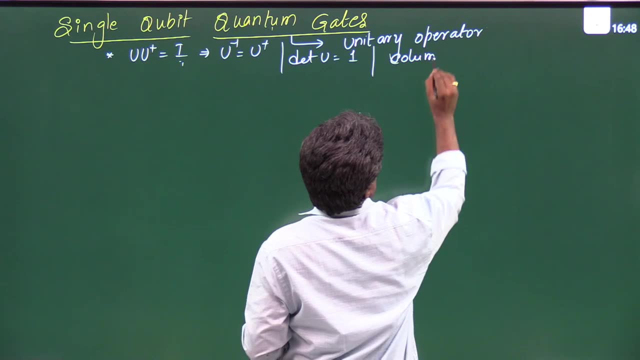 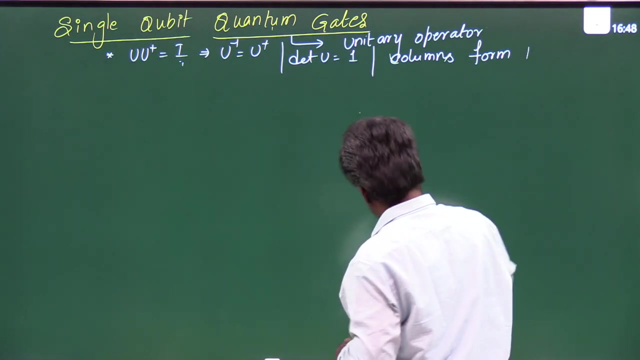 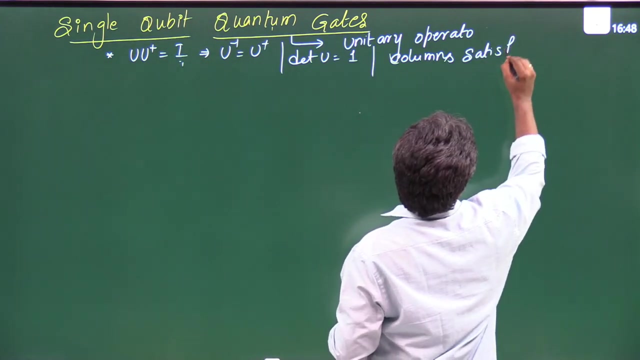 and one more: property determinant of u is equal to one in mathematics. i discussed this. and one more thing: the columns. the columns form, orthonormal basis. yes, form or not. from one minute, the columns satisfy, satisfy, orthonormal condition, orthonormal condition, orthonormal. 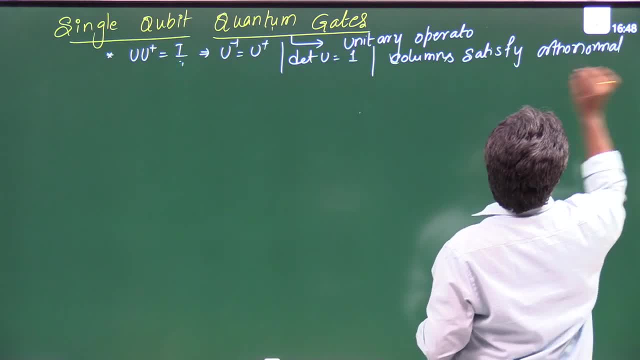 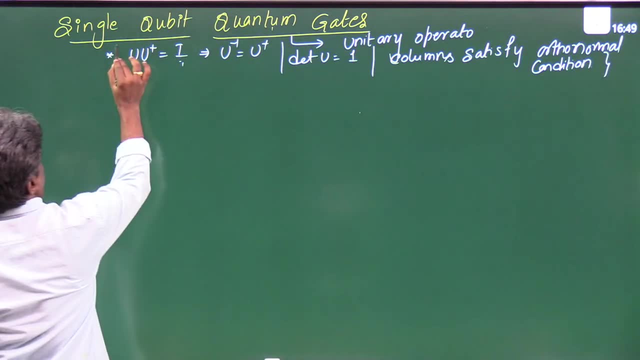 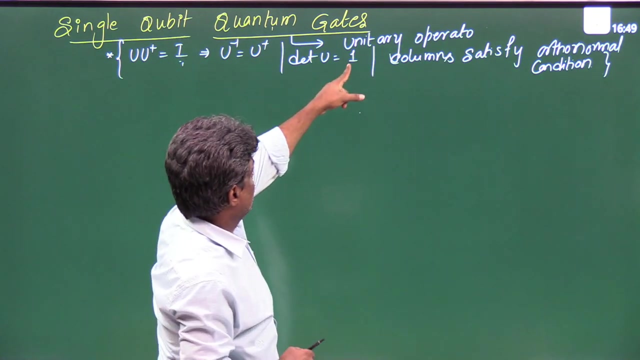 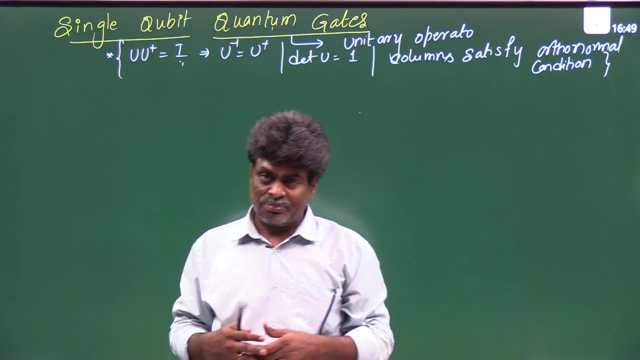 orthonormal condition. okay, that's it. so these are the few properties of a diagonal matrix: u? u dagger is equal to i and the next one determinant is u one, and this inverse is nothing but u? dagger and columns satisfies orthonormal condition. orthonormal condition means a self product is equal to one and the two different. 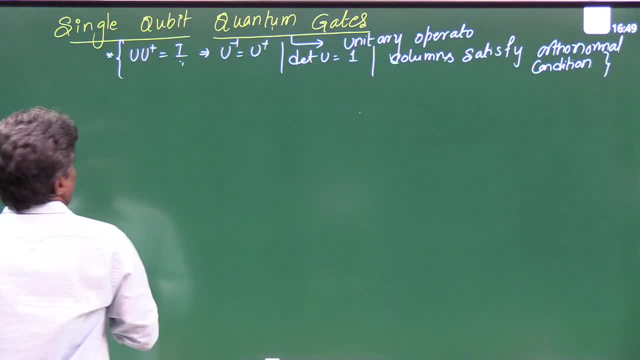 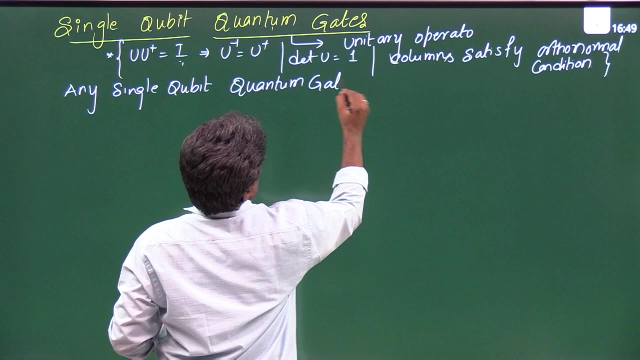 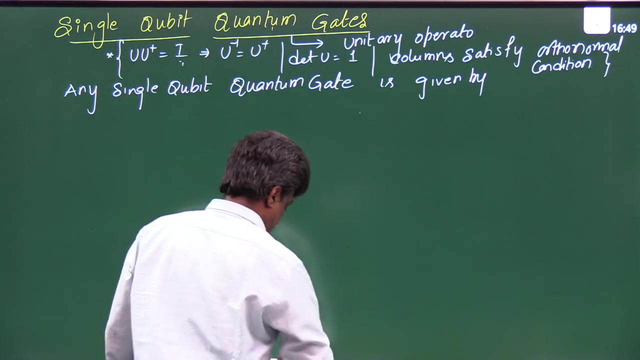 products is equal to zero. that's good. right now, here, any single qubit��을 quer d servir any single qubit. quantum gate, it's a quantum gate. so quantum gate is represented by or abandonen т Dong, given by τ v, by uncorrected. 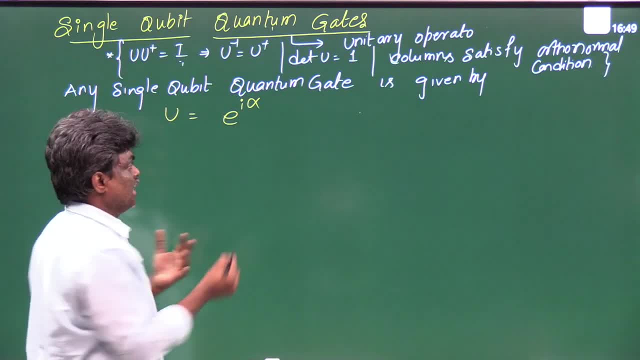 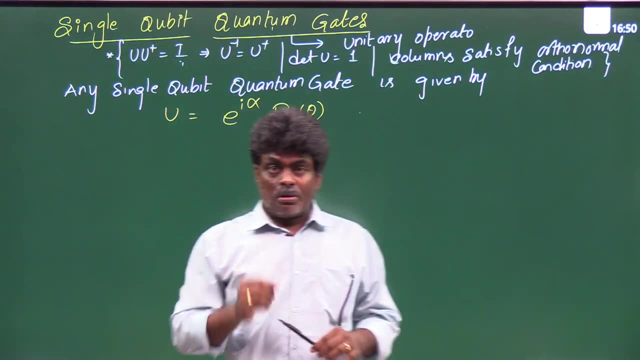 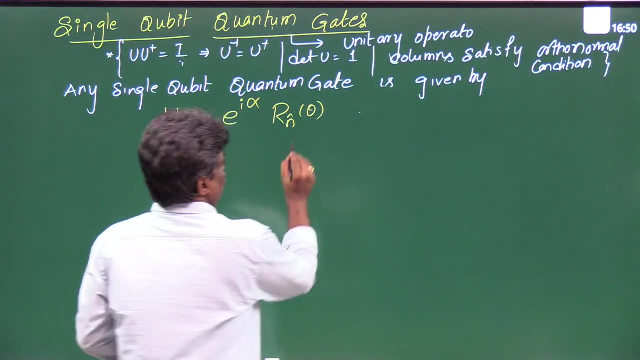 vai oli alpha and r? n cap of theta. this is what i told you yesterday. a last concept: whatever we have discussed the rotation, i told you: please, this is very important, please do this derivation. i think in the last class we have already discussed this. this is nothing but e raised to 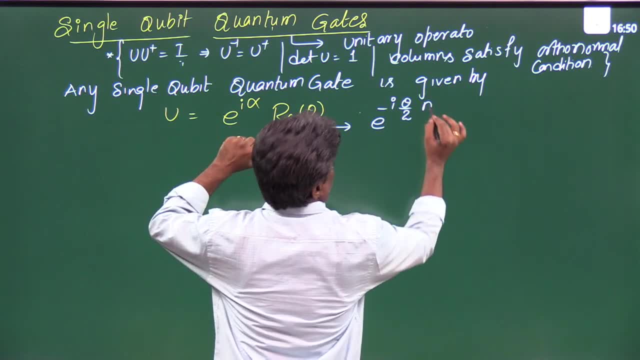 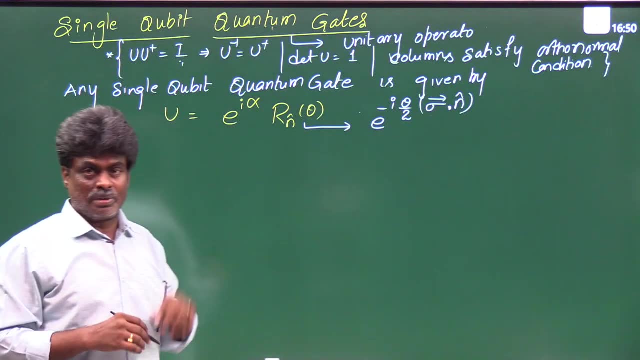 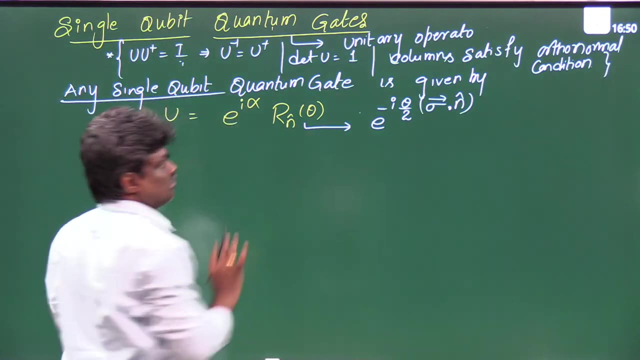 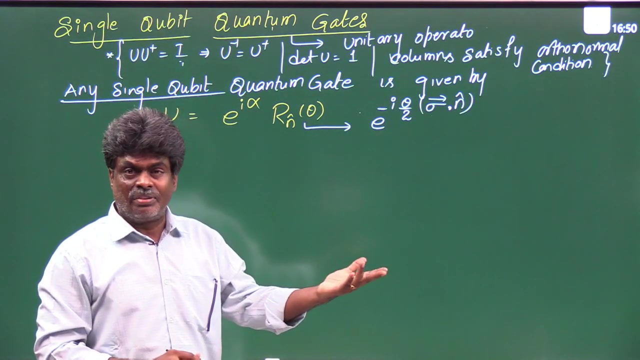 minus i theta by two sigma: sigma dot, sigma bar dot n cap. i hope you remember, okay. so then, our single qubit, any single qubit, all single qubit, quantum gates are represented by the single unitary operator, e raised to i, alpha and r n cap of theta. that means this is: 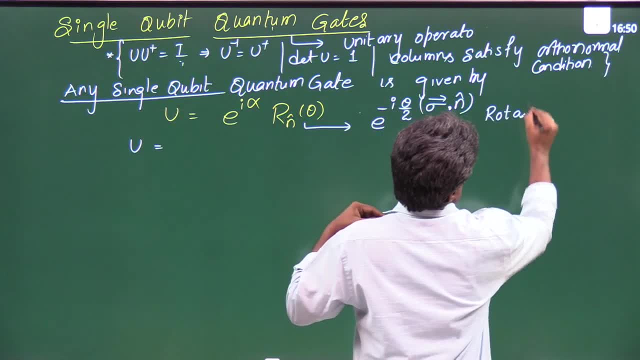 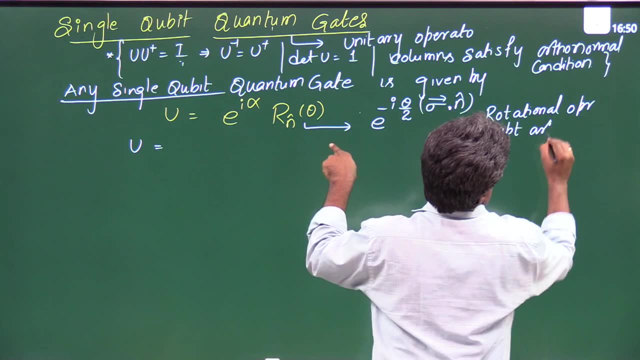 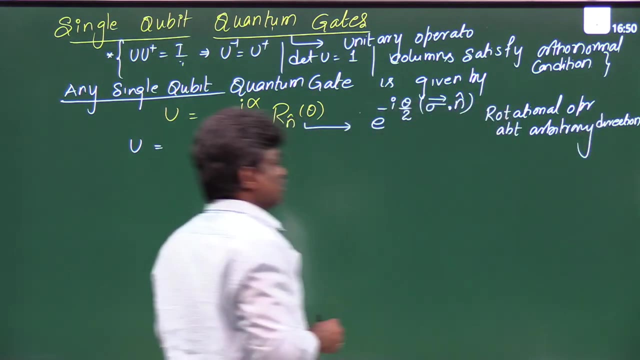 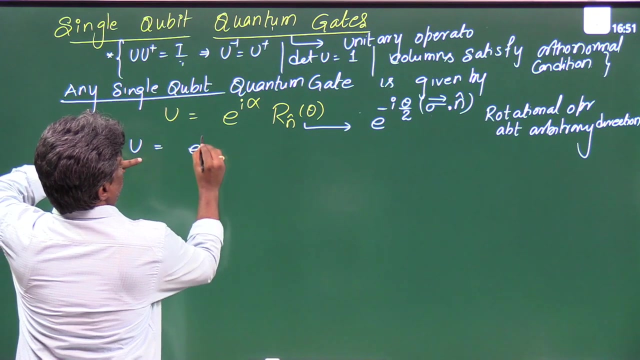 the rotation operator. this is the rotation operator. rotational operator about. about arbitrary axis or arbitrary direction. arbitrary direction, that's good. now see. okay. so this u is equal to e raised to i. alpha in the last class. i have not derived, but we already derived in the quantum mechanics. 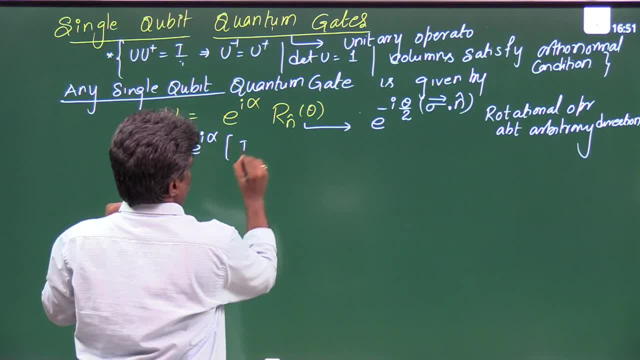 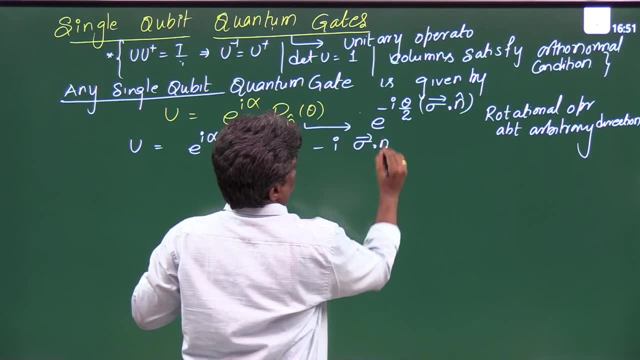 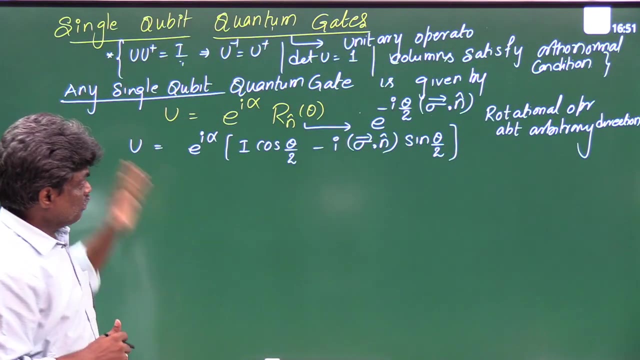 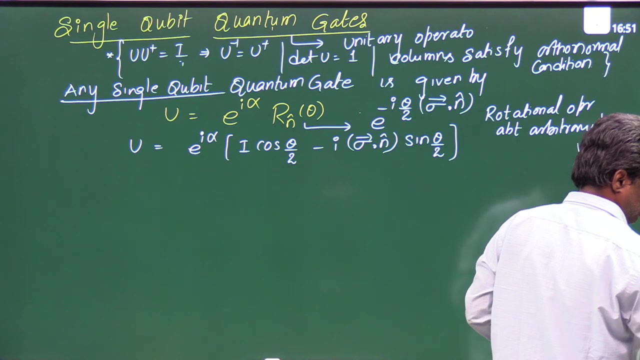 or i hope yesterday also i discussed it. this is the rotational operator: capital i cos theta by two minus i sigma bar dot n cap sine theta by two. see each and everything. we know nothing is unknown. we know everything. okay, that's good. now see, so here we have this expression. are you ready? 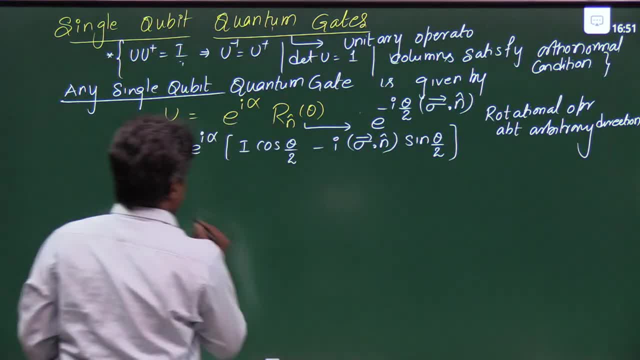 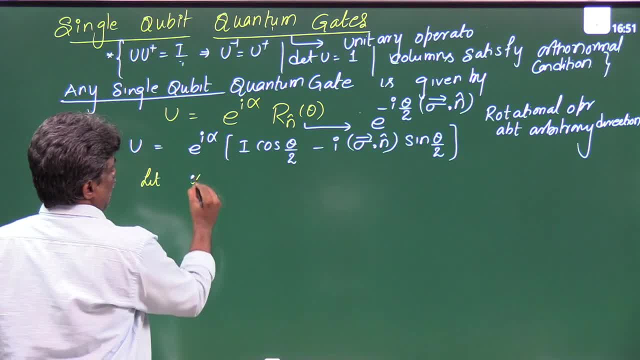 few things. this is some arbitrary angle. and this few things. this is some arbitrary angle. and this is also some is also some is also some uh angle. so now i am assuming alpha is equal uh angle. so now i am assuming alpha is equal uh angle. so now i am assuming alpha is equal to pi by two. 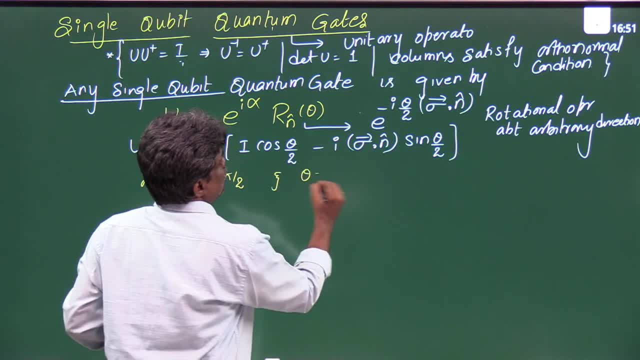 to pi by two. to pi by two: okay, and theta is equal to pi. i'm assuming, okay, and theta is equal to pi. i'm assuming, okay, and theta is equal to pi. i'm assuming, let us start. so if you take these values, let us start. so. if you take these values. 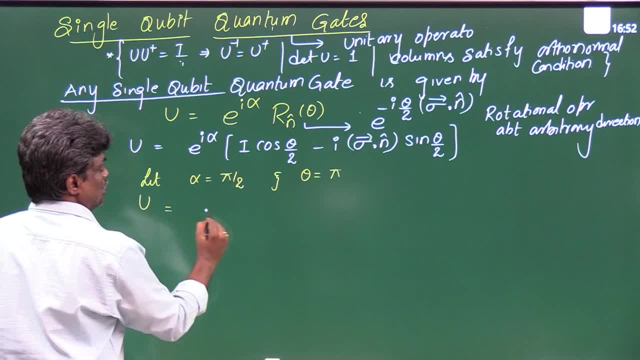 let us start. so if you take these values and a substitute there, what you will get, and a substitute there, what you will get, and a substitute there, what you will get. u is equal to e raised to i pi by 2. u is equal to e raised to i pi by 2. 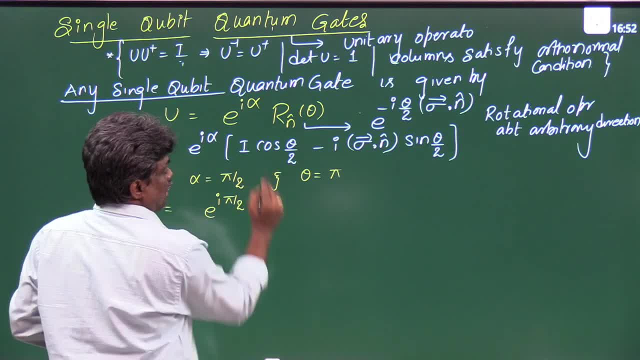 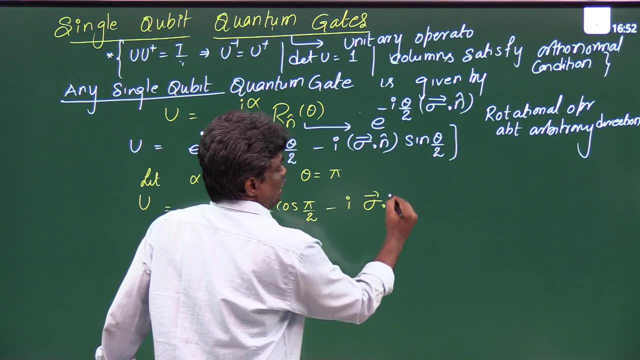 u is equal to e. raised to i pi by 2. are you observing into? are you observing into? are you observing into? i cos pi by 2. i cos pi by 2. i cos pi by 2 minus iota sigma bar dot n cap minus iota sigma bar dot n cap. 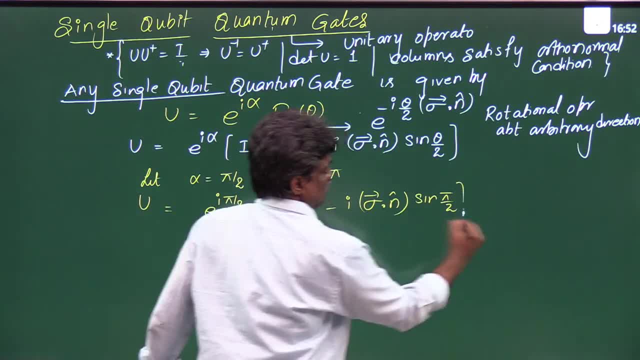 minus iota sigma bar dot n cap, and this is a sine pi by 2 and this is a sine pi by 2, and this is a sine pi by 2, that's good. and cos pi by 2 is a zero, that's good. and cos pi by 2 is a zero. 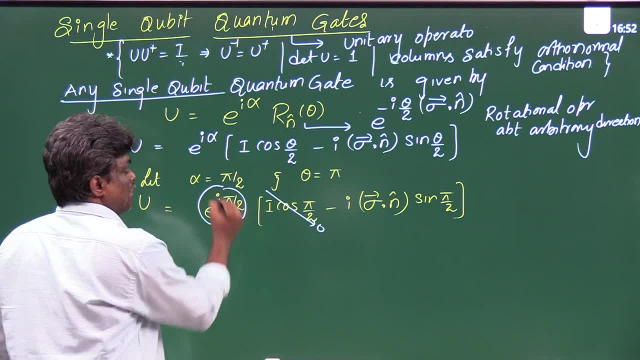 that's good and cos pi by 2 is a zero. that's why this is a zero, that's why this is a zero, that's why this is a zero. and e raised to i pi by 2 is iota and e raised to i pi by 2 is iota. 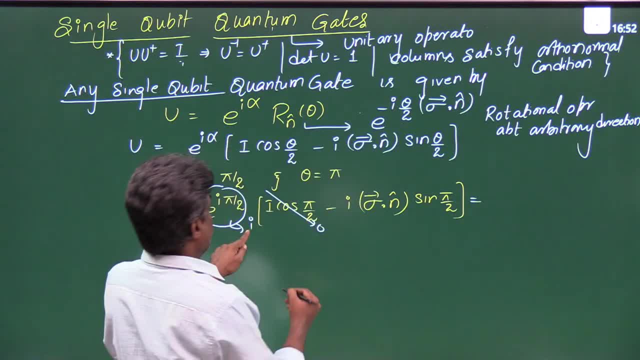 and e, raised to i pi by 2, is iota. so this is a zero, so which is nothing. so this is a zero, so which is nothing. so this is a zero, so which is nothing but but but here iota and minus iota one. here iota and minus iota one. 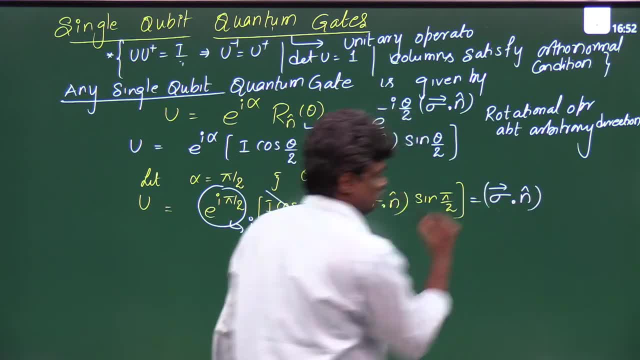 here iota and minus iota, one, and which is a simply sigma bar dot n and which is a simply sigma bar dot n and which is a simply sigma bar dot n, cap, cap, cap, because the sine pi by 2 is 1. because the sine pi by 2 is 1. 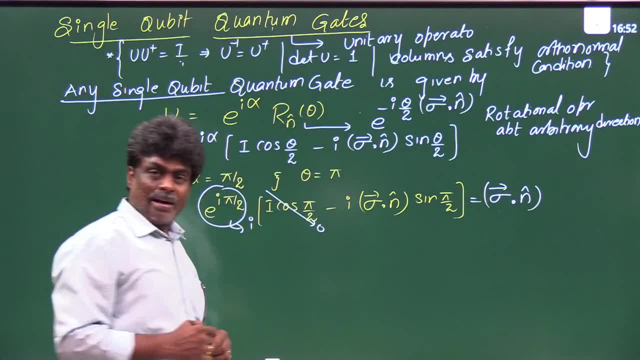 because the sine pi by 2 is 1. so, finally, here you got. u is equal to. so. finally, here you got, u is equal to. so, finally here you got. u is equal to sigma bar dot n cap. sigma bar dot n cap. sigma bar dot n cap. that's good. so u is equal to sigma bar. 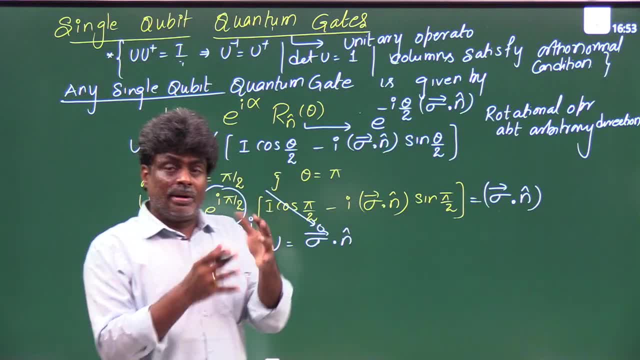 that's good. so u is equal to sigma bar dot n cap dot n cap dot n cap directly. they will write sigma x, sigma y directly. they will write sigma x, sigma y directly. they will write sigma x, sigma y, sigma z. but here what i'm saying is: 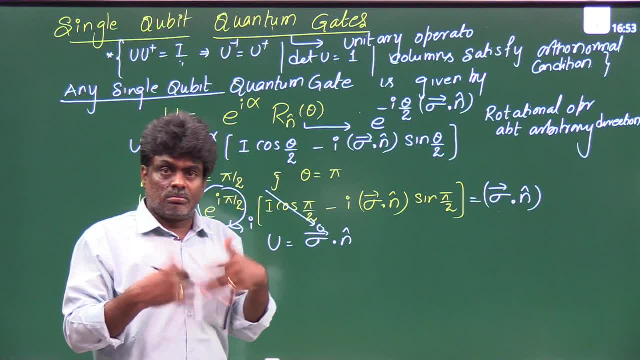 sigma z, but here what i'm saying is sigma z, but here what i'm saying is i i'm explaining more general. maybe i i'm explaining more general. maybe i i'm explaining more general. maybe tomorrow, tomorrow, tomorrow, in future, maybe some other gate is in future, maybe some other gate is. 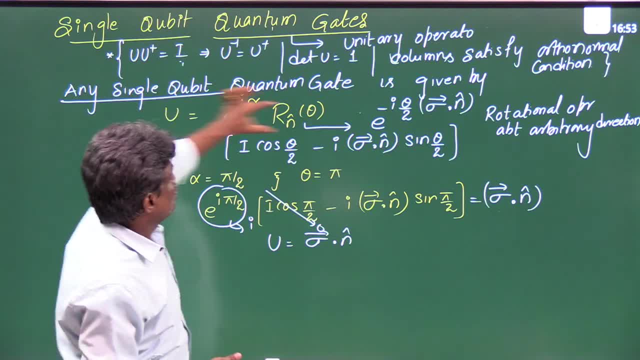 in future, maybe some other gate is introduced, introduced, introduced, then also it must be in this form. only then also it must be in this form. only then also it must be in this form. only that's good, that's good, that's good. and now see the beauty. 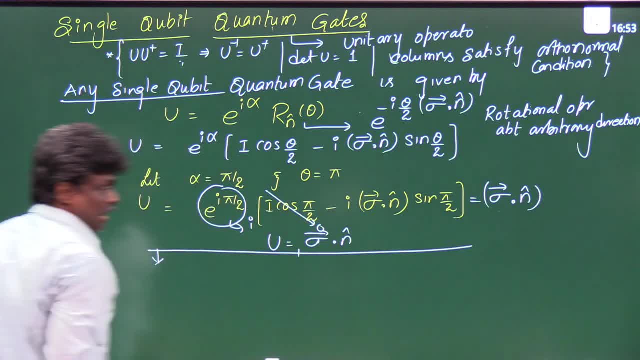 and now see the beauty. and now see the beauty if i consider the different values for, if i consider the different values for, if i consider the different values for this n cap, this n cap, this n cap- that means i'm taking n cap is equal to. that means i'm taking n cap is equal to. 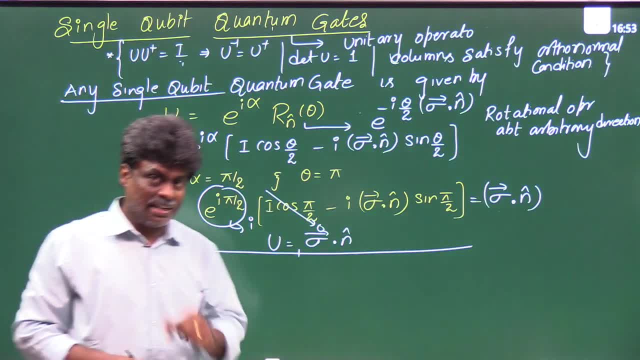 that means i'm taking n cap is equal to one comma zero comma zero. one comma zero, comma zero. one comma zero, comma zero. i hope you are understanding this is. i hope you are understanding. this is. i hope you are understanding. this is nothing but nothing but nothing but sigma x, n, x plus sigma y. 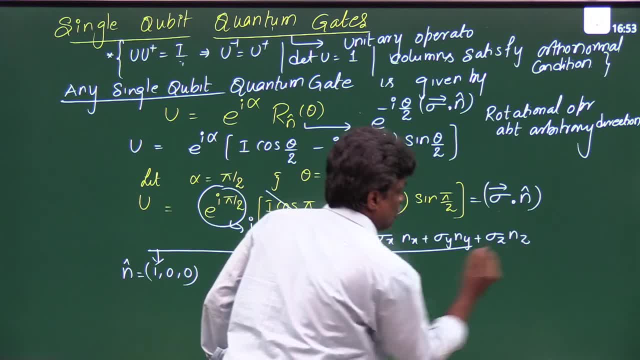 sigma x, n, x plus sigma y, sigma x, n, x plus sigma y, ny plus sigma z, ny plus sigma z, ny plus sigma z and z. i'm not using any unknown things. and z. i'm not using any unknown things and z. i'm not using any unknown things. whatever we know i'm. i'm explaining in. 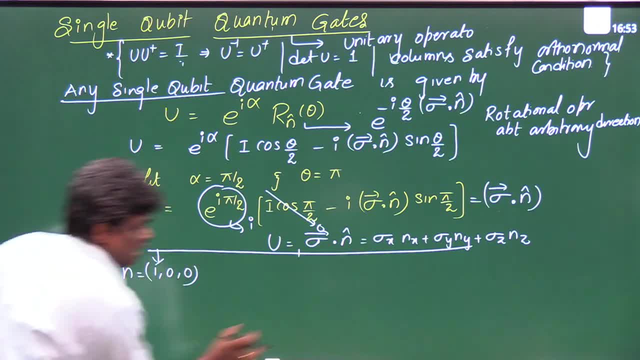 whatever we know i'm, i'm explaining in whatever we know i'm, i'm explaining in that base level only. so take this n cap, that base level only. so take this n cap, that base level only. so take this n cap and substitute here and substitute here. 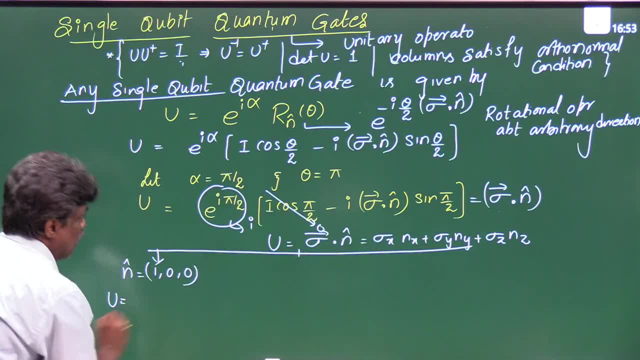 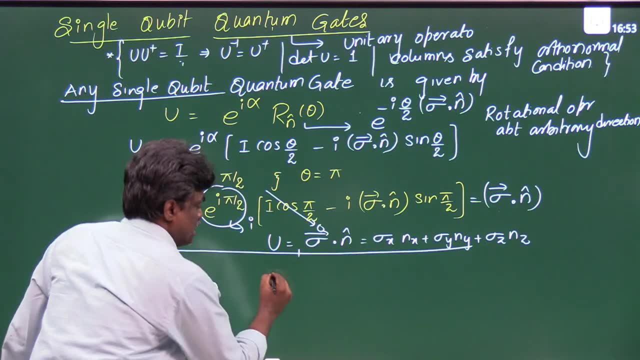 and substitute here, then your u is nothing but what, then your u is nothing but what, then your u is nothing but what. sigma x. sigma x. sigma x: 0, 1, 1, 0, 0, 1, 1 0 0, 1 1 0. if i change n cap. 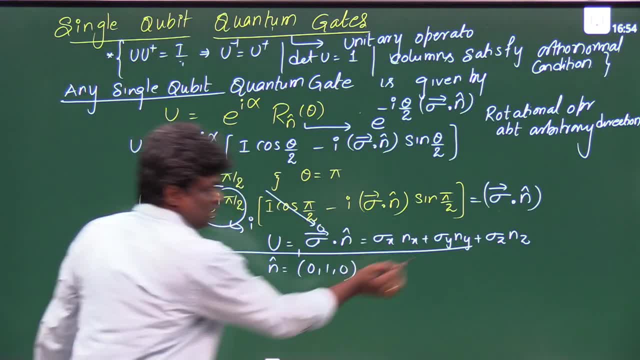 if i change n cap, if i change n cap as 0, 1, 0, as 0, 1, 0, as 0, 1, 0, so then, here you are having this. only so then, here you are having this. only so, then, here you are having this. only that's why your unitary operator is uh. 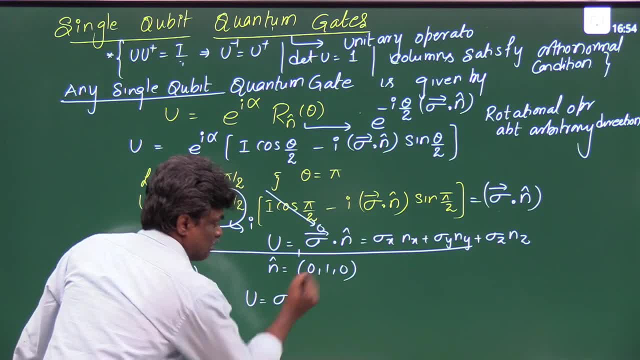 that's why your unitary operator is uh. that's why your unitary operator is uh. and what sorry, and what sorry, and what sorry. sigma y, sigma y, sigma y. into 1, which is 0 minus i i. into 1, which is 0 minus i i. 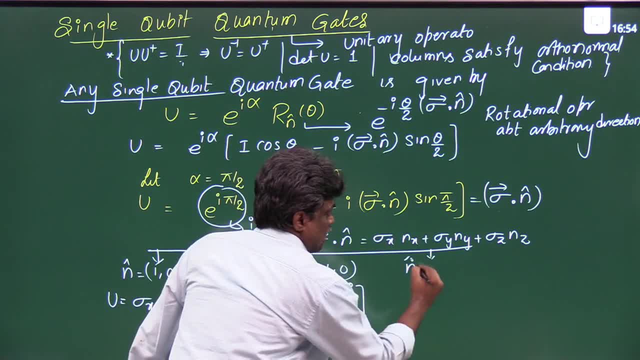 into 1, which is 0 minus i i 0. and if i take the n cap as 0 and if i take the n cap as 0 and if i take the n cap as 0, 0, 1, 0, 0, 1. 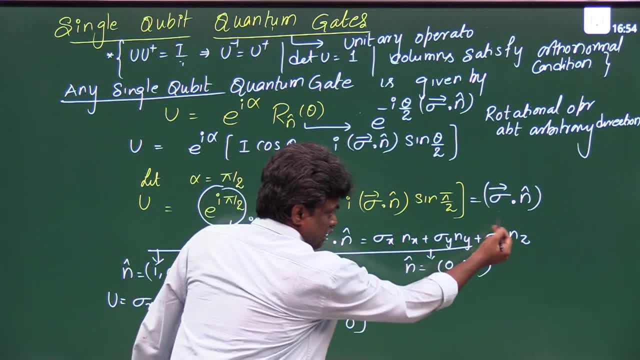 0 0 1. some arbitrary: i have taken 0 0 1. then some arbitrary: i have taken 0 0 1, then some arbitrary: i have taken 0 0 1. then this will be the value u is equal to. 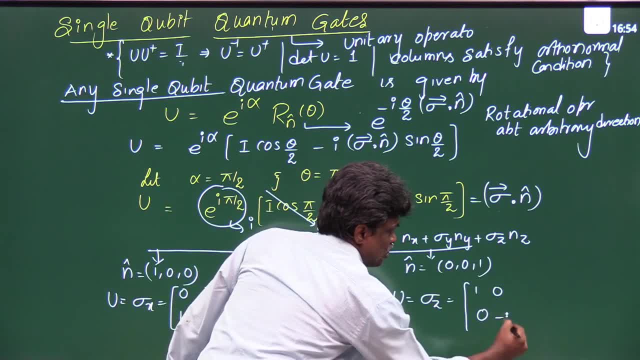 this will be the value u is equal to. this will be the value u is equal to: sigma j, sigma j, sigma j, which is 1 0 0 minus 1, which is 1 0 0 minus 1, which is 1 0 0 minus 1. so, 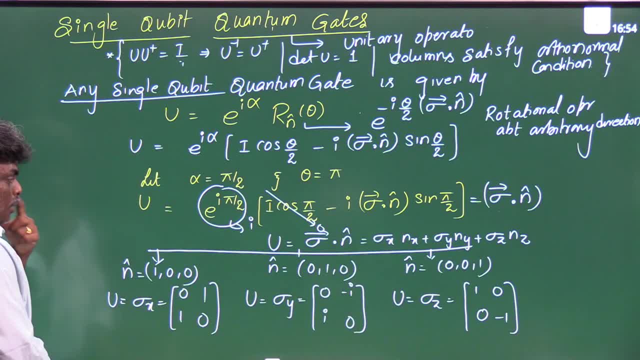 so. so this is another thing, but one of the this is another thing, but one of the this is another thing, but one of the single qubit quantum gate, which is single qubit quantum gate, which is single qubit quantum gate, which is represented by, represented by. 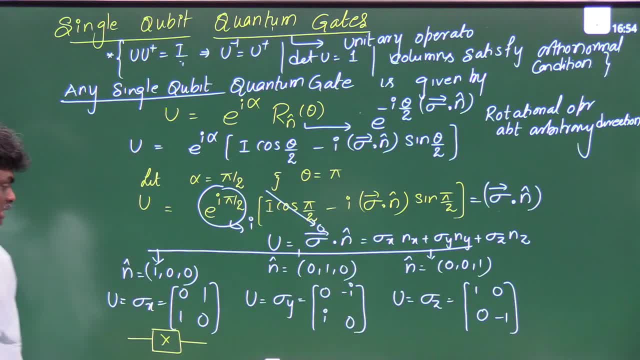 represented by x. this is a representation x. this is a representation x. this is a representation. and this is another single qubit state and this is another single qubit state and this is another single qubit state: qubit quantum gate, which is represented. qubit quantum gate, which is represented. 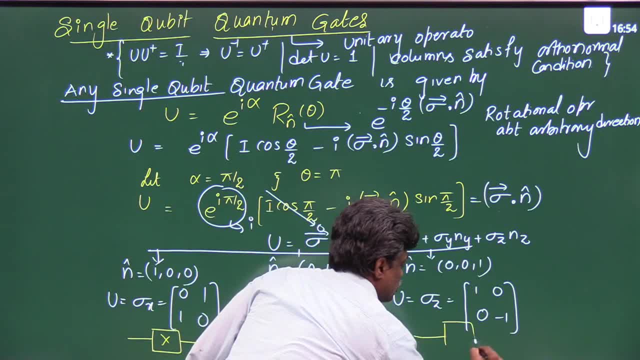 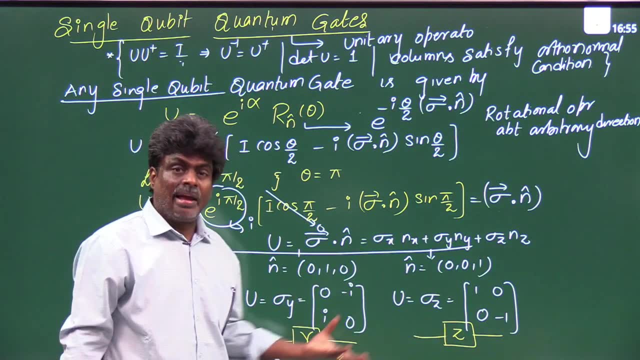 qubit, quantum gate, which is represented by y, by y, by y, and this is another single qubit and this is another single qubit, and this is another single qubit, quantum gate, represented by quantum gate, represented by quantum gate, represented by j simply, j, simply, j simply. poly x, poly y and poly z. 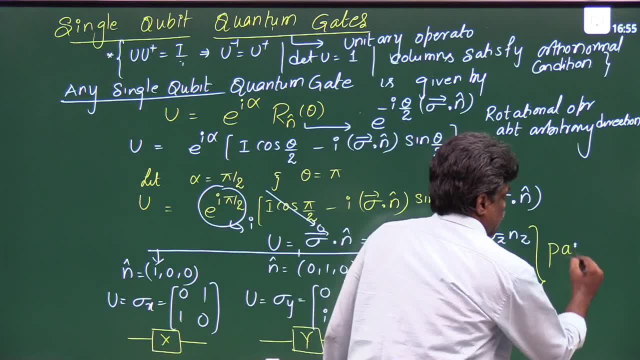 poly x, poly y and poly z. poly x, poly y and poly z. so these are three gates. we call it as a. so these are three gates. we call it as a. so these are three gates. we call it as a poly gates. poly gates x, y, z. 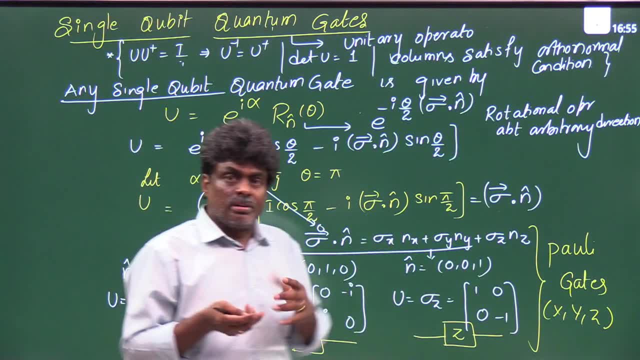 x, y, z, x, y z. i hope you understand the more general. i hope you understand the more general. i hope you understand the more general form of a single qubit quantum gate. form of a single qubit quantum gate. form of a single qubit quantum gate. single qubit quantum gate e raise to i. 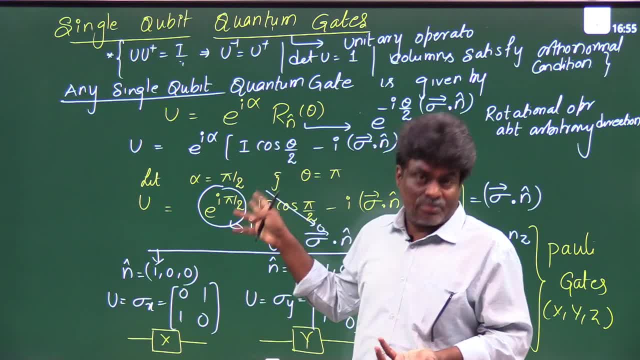 single qubit quantum gate. e raise to i single qubit quantum gate. e raise to i alpha into rotational operator alpha into rotational operator alpha into rotational operator rn cap of theta. because you know this rn cap of theta, because you know this rn cap of theta, because you know this, and whatever it may be, this is a. 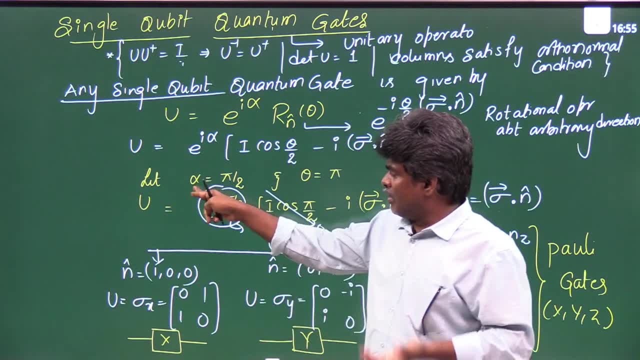 and whatever it may be, this is a and whatever it may be, this is a. representing some phase actually okay. representing some phase actually okay. representing some phase actually okay. so i have given a alpha value pi by two. so i have given a alpha value pi by two. 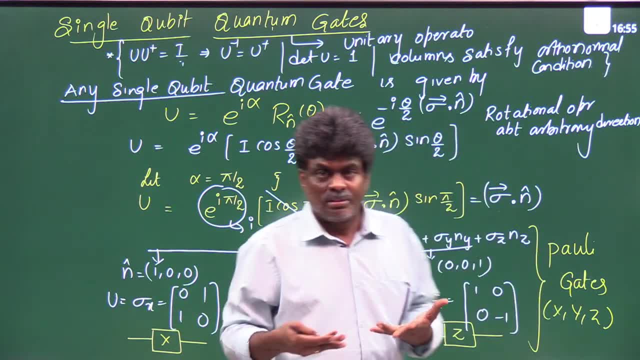 so i have given a alpha value, pi by two, and theta is pi, and i have taken and theta is pi, and i have taken and theta is pi, and i have taken different n caps, different n caps, different n caps. then i got a poly x gate, poly y gate. 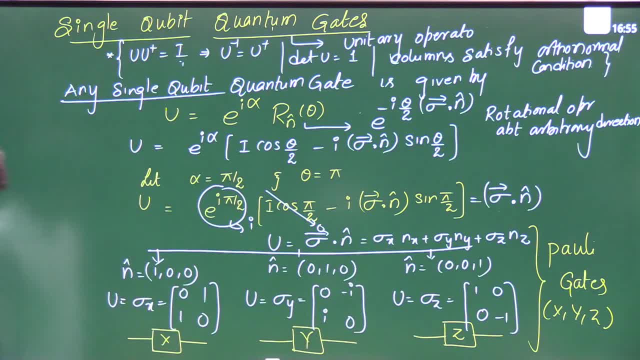 then i got a poly x gate, poly y gate. then i got a poly x gate, poly y gate and poly z gate. okay, come on right, listen. so the next one. uh right, listen. so the next one. uh right, listen. so the next one. uh, very important one. so here what we get. 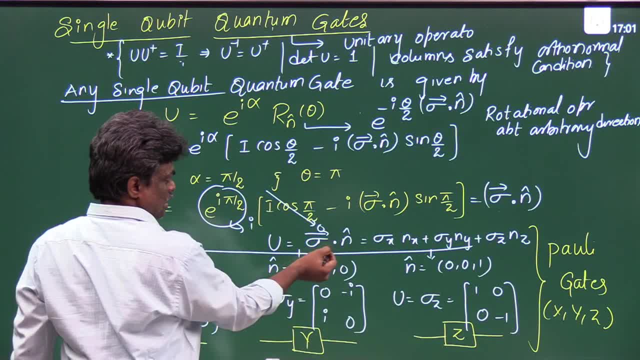 very important one. so here what we get: very important one. so here what we get. uh, this one, this is a sigma bar. uh, this one, this is a sigma bar. uh, this one, this is a sigma bar, sigma dot n cap. okay, so once again, i'm sigma dot n cap. okay, so once again i'm. 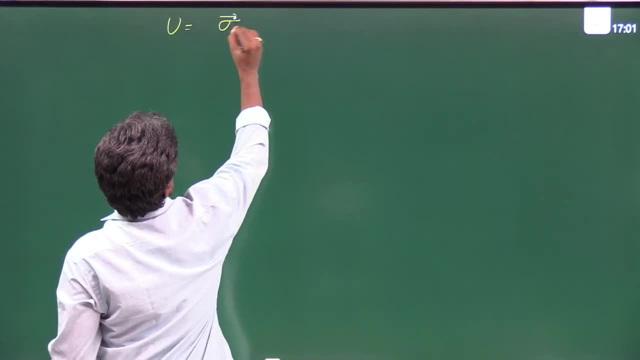 sigma dot n cap. okay, so once again, i'm taking that, taking that, taking that. you, we got a sigma dot n cap. you, we got a sigma dot n cap. you, we got a sigma dot n cap. everybody, please listen, this is a very. everybody, please listen, this is a very. 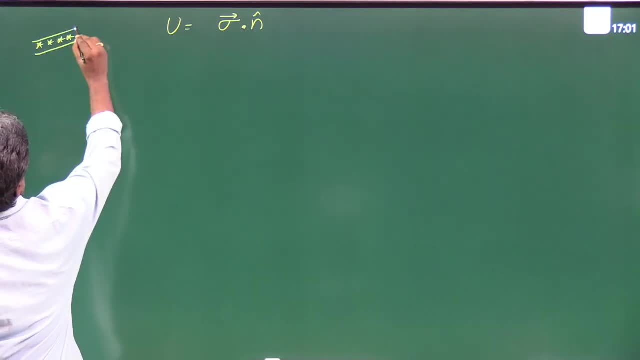 everybody, please listen, this is a very, very, very, very, very, very important, very, very, very, very, very, very, very important, very, very, very, very, very, very, very important. everyone, please, everyone, please, everyone please. so here i'm taking n cap is equal to: so here i'm taking n cap is equal to: 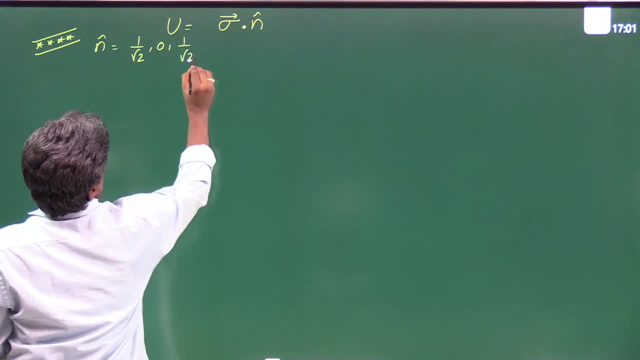 so here i'm taking n. cap is equal to 1 by root 2 0, 1 by root 2. are you 1 by root? 2 0. 1 by root 2. are you 1 by root 2 0, 1 by root 2. are you observing? 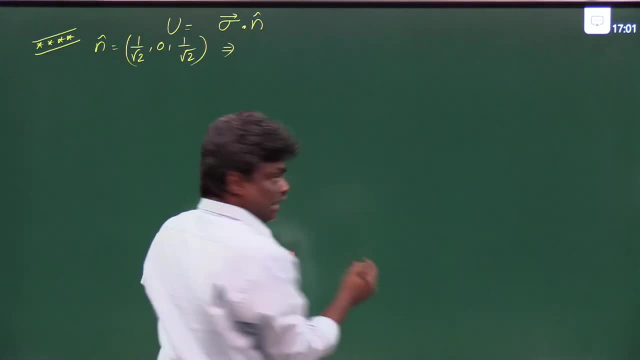 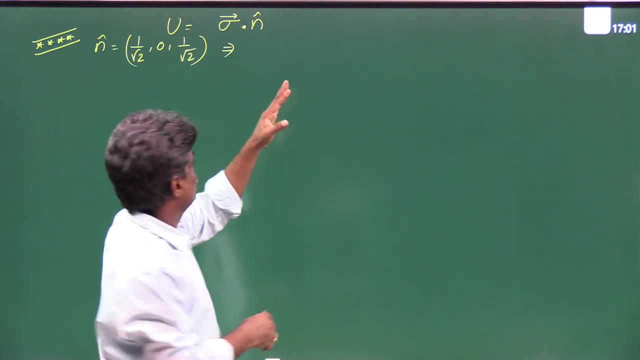 observing, observing. yes, sir, so this is uh earlier i have. yes, sir, so this is uh earlier i have. yes, sir, so this is uh earlier i have taken one zero, zero, zero, one zero, zero. taken one zero, zero, zero. one zero, zero, zero, one. taken one zero, zero, zero, zero. one zero, zero, zero, one by root 2. now come on substitute. 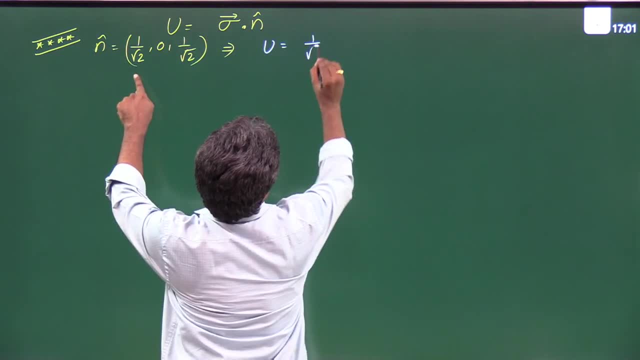 by root 2 now come on substitute by root 2 now come on substitute then. u is equal to here, we'll get 1 by then. u is equal to here, we'll get 1 by then. u is equal to here. we'll get 1 by root 2 into sigma x. 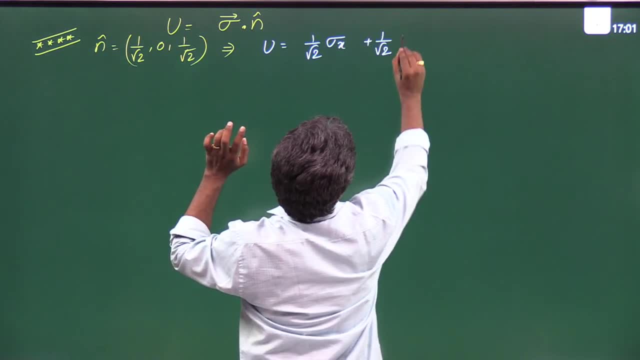 root 2 into sigma x. root 2 into sigma x. second one is a 0 and 1 by root 2. second one is a 0 and 1 by root 2. second one is a 0 and 1 by root 2 into sigma z. am i right? yes, sir. 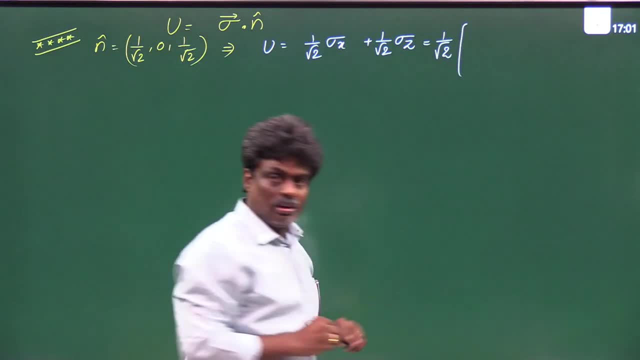 into sigma z, am i right? yes, sir, into sigma z, am i right? yes, sir, so i'm taking 1 by root, 2 common. so i'm taking 1 by root, 2 common. so i'm taking 1 by root, 2 common. just add sigma x and sigma y, if you add. 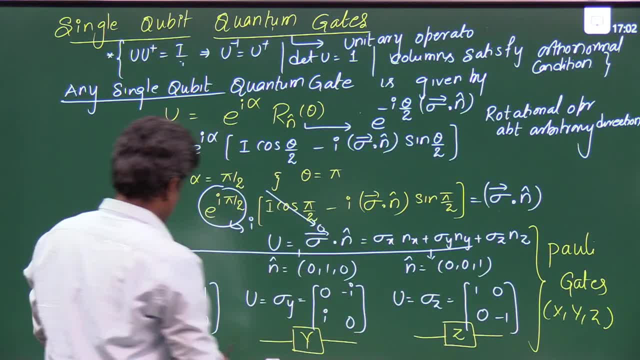 just add sigma x and sigma y. if you add, just add sigma x and sigma y. if you add sigma x and sigma y, sigma x and sigma y, sigma x and sigma y. this is your sigma x: 0 1 1 0. this is your sigma x: 0 1 1 0. 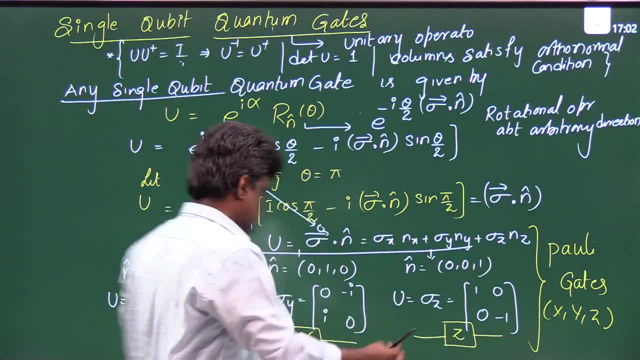 this is your sigma x 0 1 1 0 and sigma z 1 0 0 minus 1, just and sigma z 1 0 0 minus 1, just and sigma z 1 0 0 minus 1. just add these two what you will get. 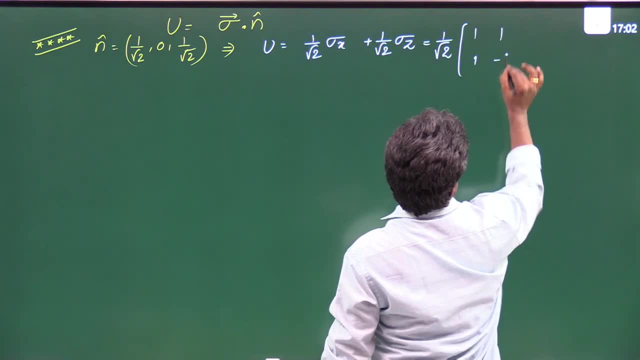 add these two. what you will get, add these two, what you will get that is, that is that is one one, one minus one. one, one, one minus one. one, one one minus one. that's good, that's good, that's good. this is the another. this is the another. 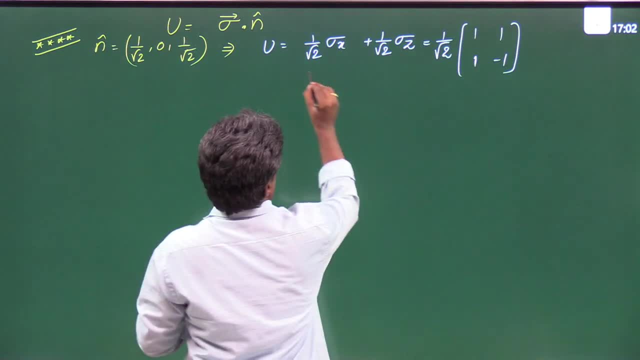 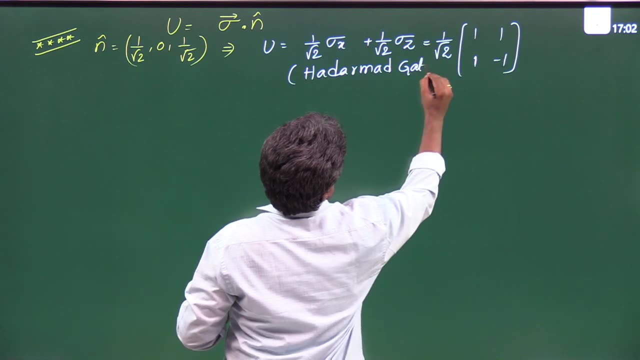 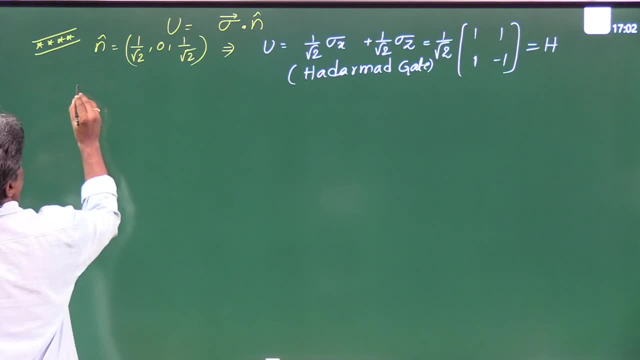 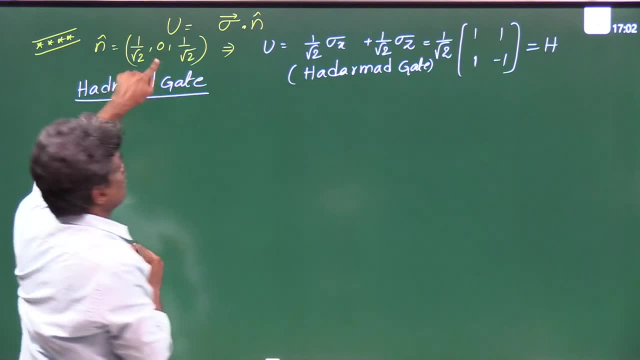 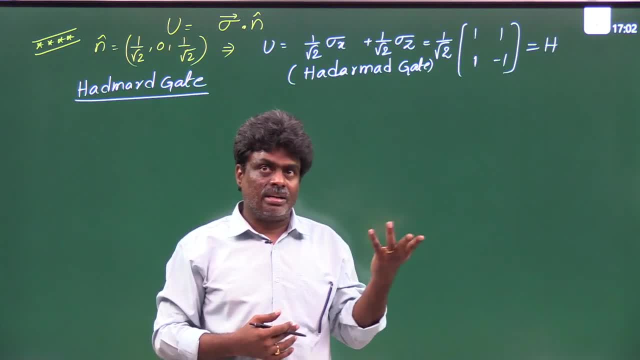 end cap rotation rotation about x z plane. end cap rotation rotation about x z plane. i hope you are understanding. if anybody, i hope you are understanding. if anybody, i hope you are understanding. if anybody, ask, ask, ask. what is the graphically, what is the head? what is the graphically? what is the head? 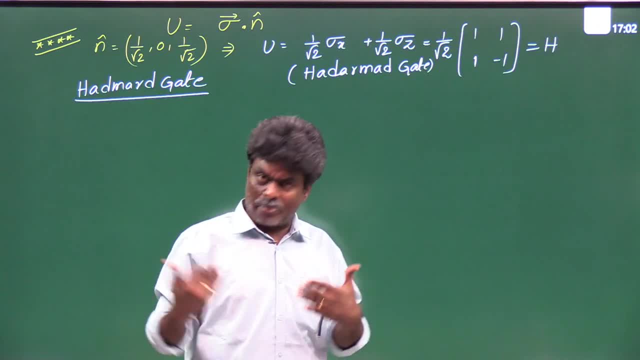 what is the graphically? what is the head? market? it's a simple rotation about market. it's a simple rotation about market. it's a simple rotation about x- z plane. that is a 1 by root 2, 1 by x z plane. that is a 1 by root 2, 1 by. 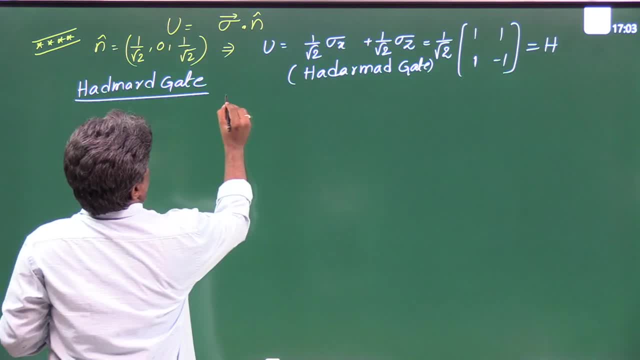 x z plane. that is a 1 by root 2. 1 by root 2, here it's a 0 root 2, here it's a 0 root 2, here it's a 0. so this head mod gate we got h is equal. 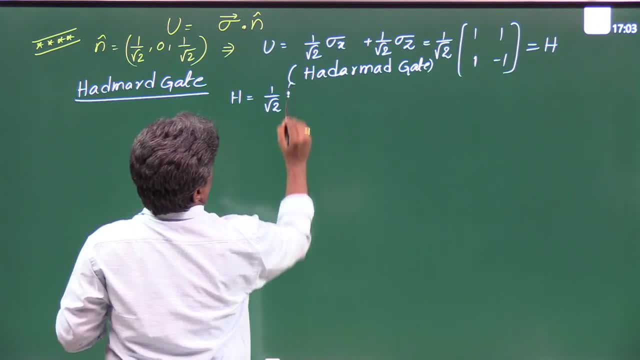 so this head mod gate we got h is equal. so this head mod gate we got h is equal to to to 1 by root 2 unitary operator a 1 1. 1 by root 2 unitary operator a 1- 1. 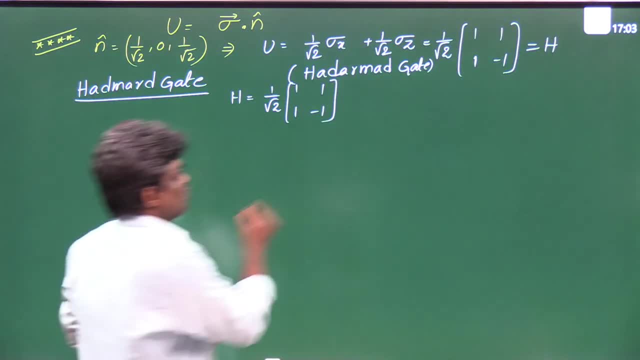 1 by root. 2, unitary operator a: 1 1 1 minus 1, 1 minus 1, 1 minus 1. and if you observe carefully, h square, if and if you observe carefully, h square, if and if you observe carefully, h square, if you square this, what you will get i 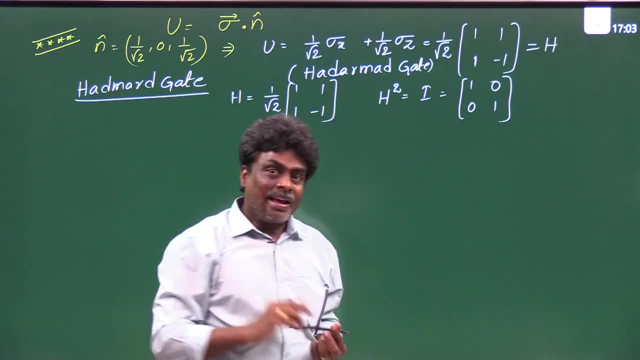 you square this what you will get, i. you square this what you will get, i. okay, okay, okay, so, so, so, if you apply head market twice, if you apply head market twice, if you apply head market twice, you'll get the same state again. i repeat. you'll get the same state again. i repeat. 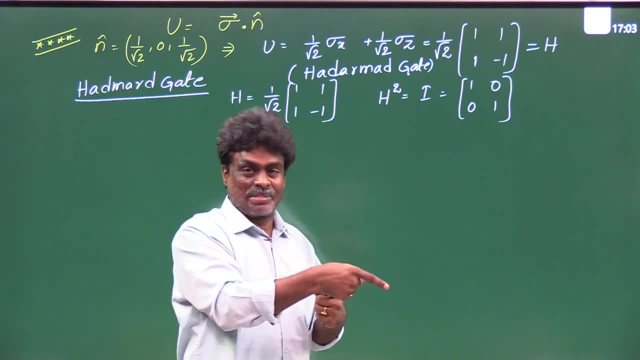 you'll get the same state again. i repeat: if you apply head mod gate twice, you'll. if you apply head mod gate twice, you'll. if you apply head mod gate twice, you'll get the same state clear good. get the same state clear, good. get the same state: clear, good. so this is about, uh, head market, fine. 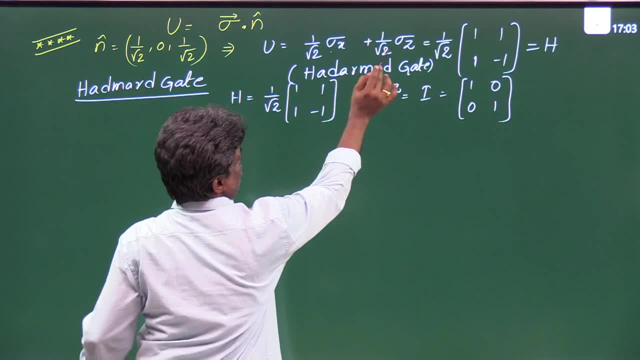 so this is about uh head market, fine. so this is about uh head market, fine. and which is a linear combination of and which is a linear combination of, and which is a linear combination of sigma x and sigma z, it's not a state. sigma x and sigma z, it's not a state. 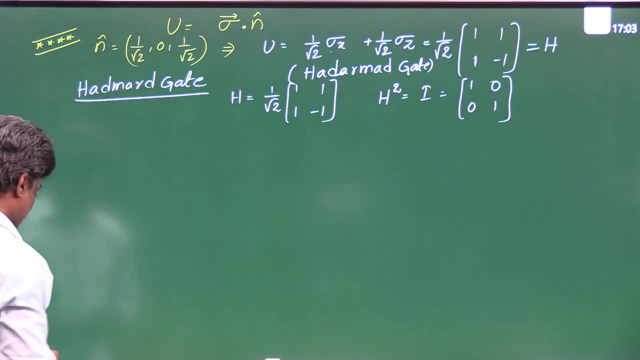 sigma x and sigma z. it's not a state. matrices, just a combination of those two matrices. just a combination of those two matrices. just a combination of those two matrices, matrices, matrices. okay, so let me discuss more detail. okay, so, let me discuss more detail. okay, so let me discuss more detail about. 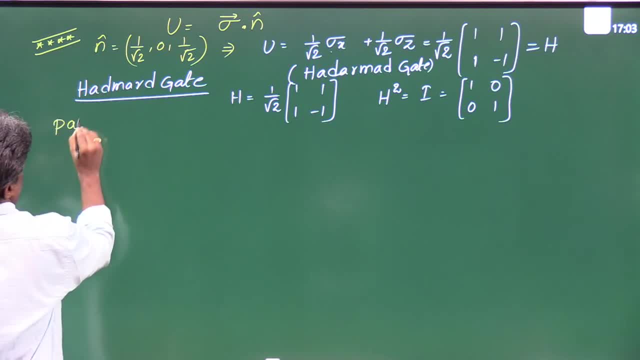 about, about these, these, these poly gates, first poly gates, first poly gates first. let me take first. let me take first, let me take first pauli gates. let us discuss more detail this head market, let us discuss more detail, this head market, let us discuss more detail. this head market also will discuss just laser. 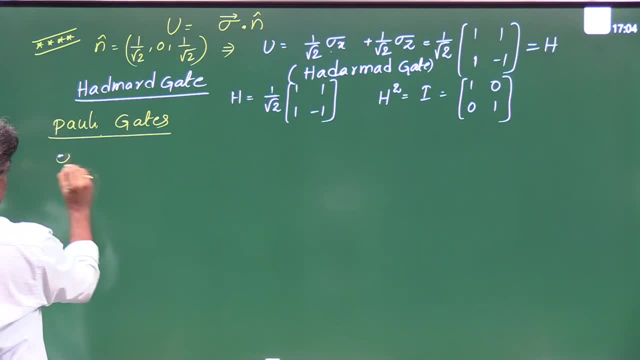 also will discuss just laser. also will discuss just laser. now here, poly gates, first one. we have now here, poly gates, first one. we have now here, poly gates, first one. we have sigma x, sigma x, sigma x. so you know everyone what is the sigma x. so you know everyone what is the sigma x. 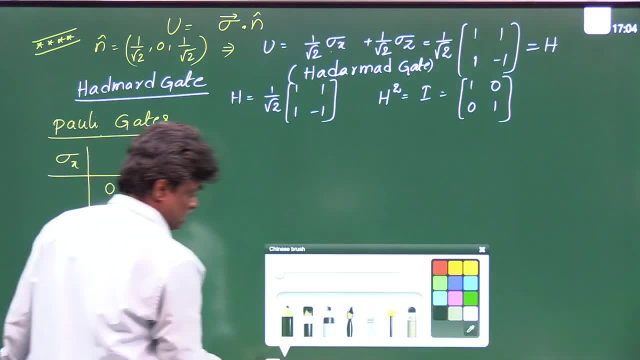 so you know everyone what is the sigma x? uh zero, one, one, zero, carefully, please. uh, zero one, one, zero, carefully, please. uh zero, one, one, zero, carefully, please listen. this is very important, listen, this is very important, listen. this is very important. i will explain. first one, next one: you. 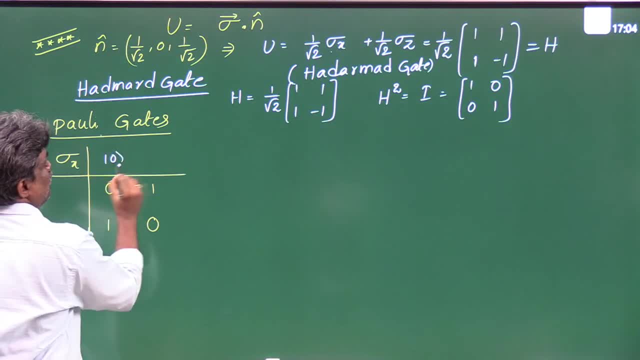 i will explain first one, next one, you. i will explain first one, next one, you, please do it, please do it, please do it. could you please tell me what are the? could you please tell me what are the? could you please tell me what are the basis states? we have zero. 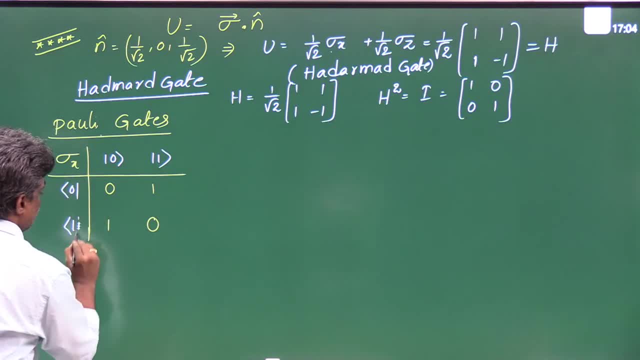 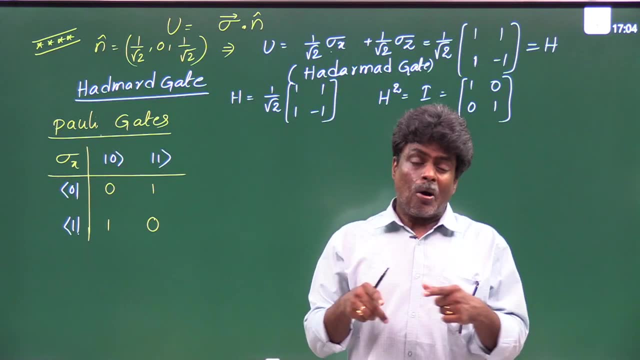 basis states. we have zero basis states. we have zero. one here the bra vector zero, and one here the bra vector zero and one here the bra vector zero. and one, one one in quantum mechanics classes. we have in quantum mechanics classes. we have in quantum mechanics classes. we have discussed how to express any operator in 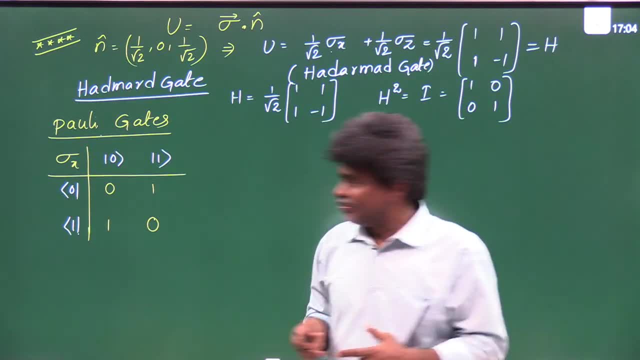 discussed how to express any operator in discussed how to express any operator in the form of outer product form. outer the form of outer product form. outer the form of outer product form. outer product form, product form, product form. so let us write that outer product form. so let us write that outer product form. 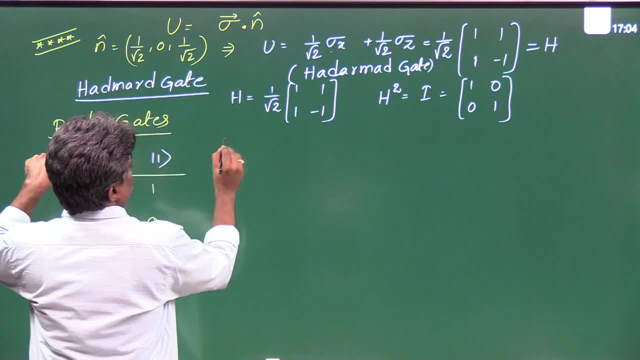 so let us write that outer product form. everyone lizard here i'm getting. i'm everyone lizard here i'm getting. i'm everyone lizard here i'm getting. i'm taking this poly x gate as a simply x, taking this poly x gate as a simply x, taking this poly x gate as a simply x, x equal to. 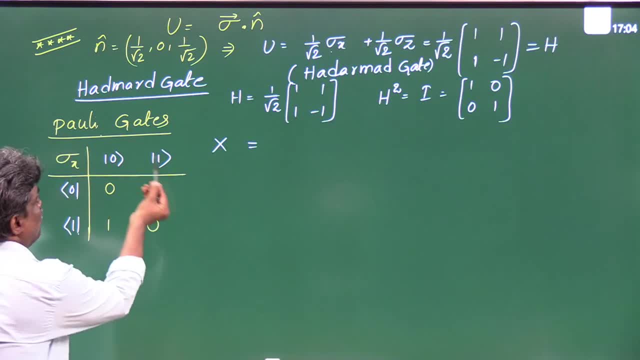 x equal to x, equal to. maybe you forgot, i'll let me explain one. maybe you forgot, i'll let me explain one. maybe you forgot, i'll let me explain one more time. more time, more time. whenever you are writing outer product. whenever you are writing outer product. 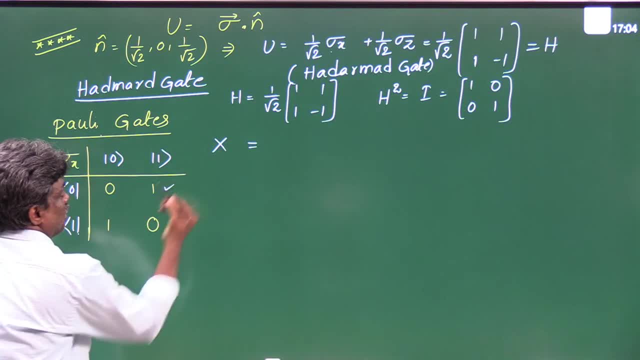 whenever you are writing outer product form. this is a zero. leave it. this is a one form. this is a zero. leave it. this is a one form. this is a zero. leave it. this is a one. you have to take this. you have to take this. you have to take this now. come to this one now. see here what. 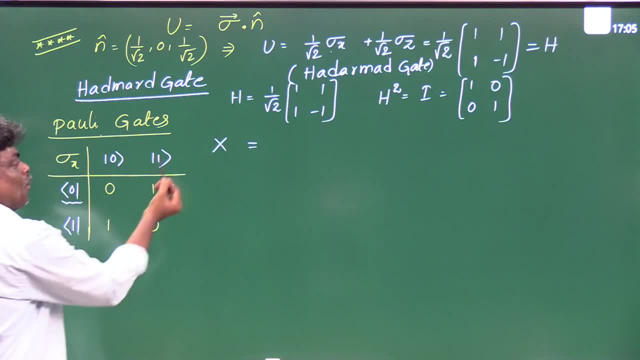 now come to this one. now see here what? now come to this one. now see here: what is the bra vector? is the bra vector? is the bra vector zero? what is the ket vector one zero? what is the ket vector one zero. what is the ket vector one? it's very simple. if you want to write, 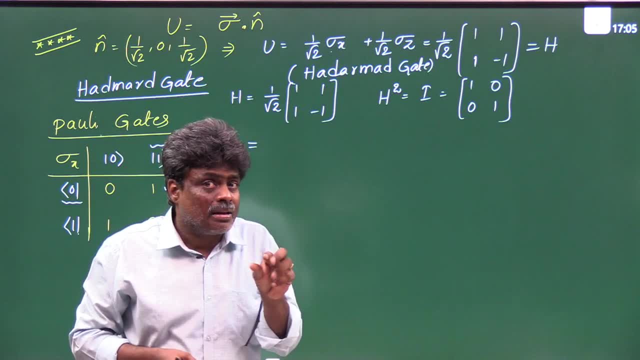 it's very simple. if you want to write, it's very simple. if you want to write: the outer product, the outer product, the outer product, whatever the bra vector is there, make it. whatever the bra vector is there, make it. whatever the bra vector is there, make it ket vector, whatever ket vector is there. 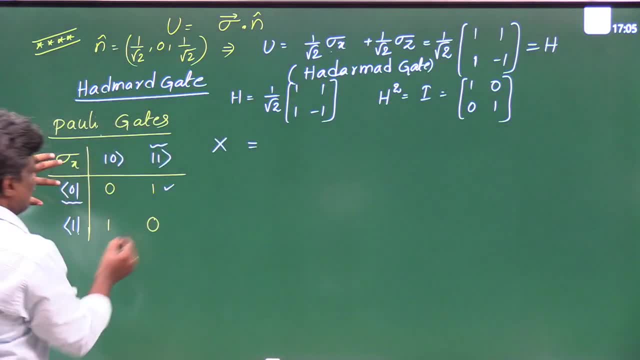 ket vector, whatever ket vector is there. ket vector, whatever ket vector is there, make it bra vector. i repeat: make it bra vector. i repeat: make it bra vector. i repeat: now i'm going to write the outer product. now i'm going to write the outer product. now i'm going to write the outer product form. 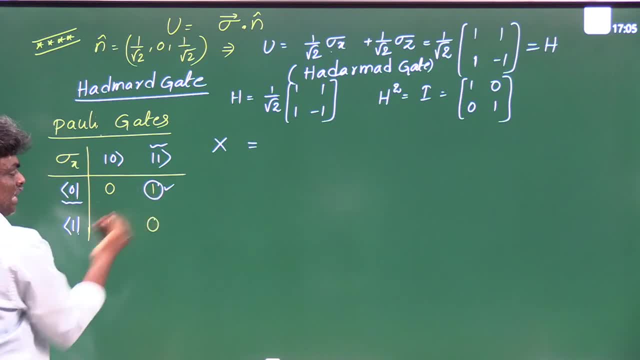 form. form. so these are the zeros. leave it wherever. so. these are the zeros. leave it wherever. so these are the zeros. leave it wherever. one is there, please go there. one is there, please go there. one is there, please go there, corresponding to this one. this is the. 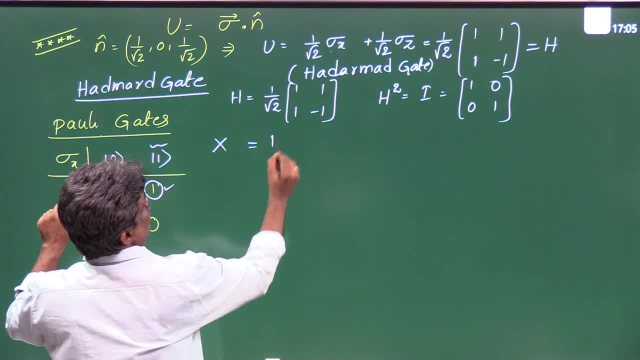 corresponding to this one. this is the corresponding to this one. this is the bra vector. bra vector. bra vector. please make this as a ket vector. please make this as a ket vector. please make this as a ket vector. actually, here it is one, one in two one. actually, here, it is one, one in two one. 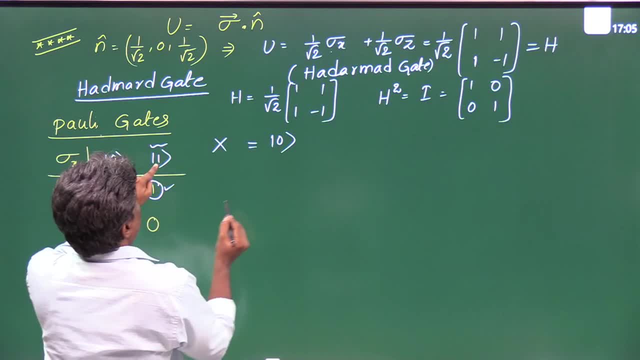 actually here it is one, one in two, one in two because i'm not taking it's in one in two, because i'm not taking it's in one in two, because i'm not taking it's in one. and whatever the ket vector just make. and whatever the ket vector just make. 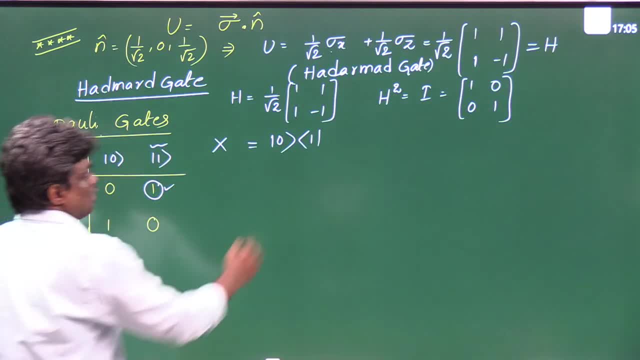 and whatever the ket vector, just make it as a bra vector, it as a bra vector, it as a bra vector. that's good plus, that's good plus, that's good plus. next one here one. next one here one. next one here one. i need not to write one. 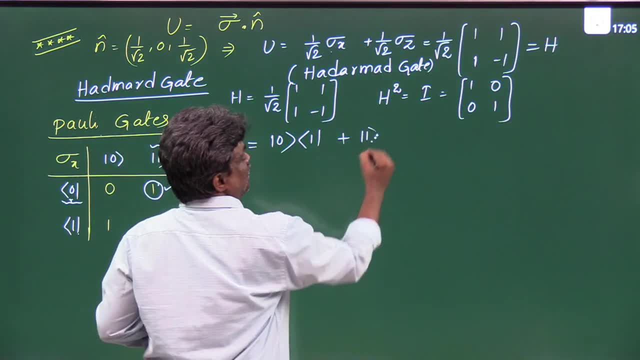 i need not to write one, i need not to write one. so again: bra vector is what one. so just so again. bra vector is what one. so just so again. bra vector is what one. so just make it a ket vector. make it a ket vector, make it a ket vector and corresponding ket vector is a zero. 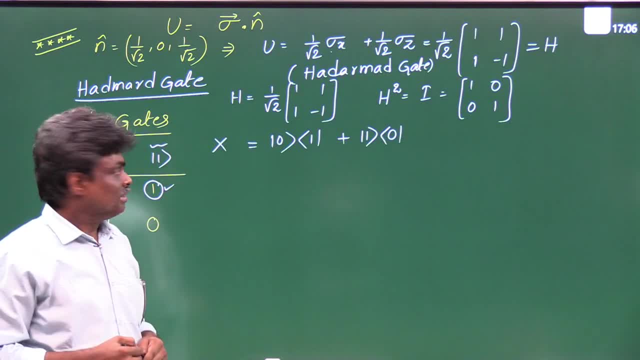 and corresponding ket vector is a zero and corresponding ket vector is a zero. make it a bra, make it a bra, make it a bra. that's it, that's it, that's it. this is the outer product form of this is the outer product form of this is the outer product form of poly x. 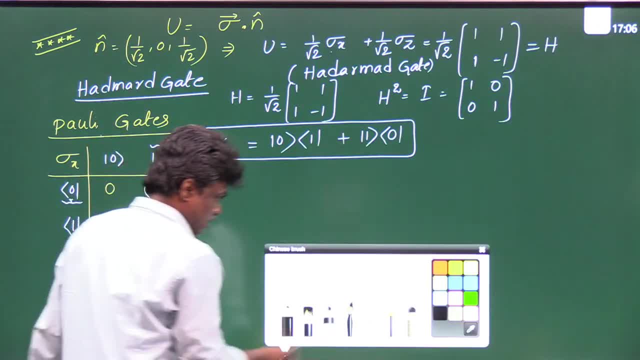 poly x, poly x gate. so what is the benefit of this yes gate? so what is the benefit of this yes gate? so what is the benefit of this yes now? this is very easy to now. this is very easy to now. this is very easy to easy for the operations. for example, 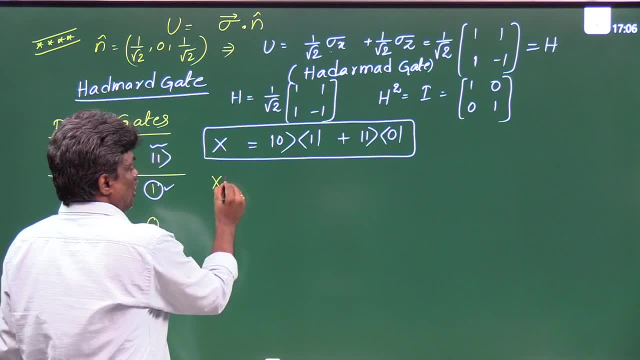 easy for the operations, for example. easy for the operations. for example, we are dealing with the single qubit. we are dealing with the single qubit. we are dealing with the single qubit. states, states, states. now poly x gate is operating on zero. now poly x gate is operating on zero. 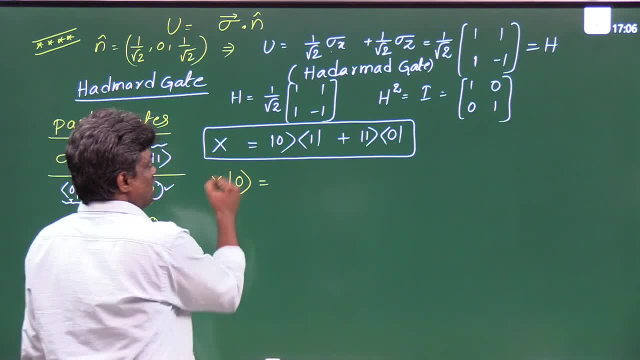 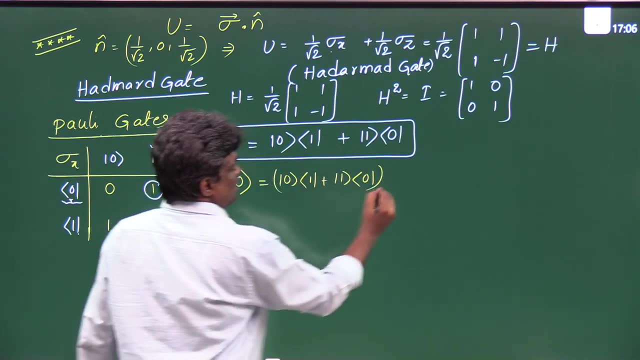 now poly x gate is operating on zero. are you observing now what is x outer? are you observing now what is x outer? are you observing now what is x outer? product, product, product, zero. one after product, plus one zero zero. one after product, plus one zero, zero. one after product, plus one zero. now this is multiplied with the zero. 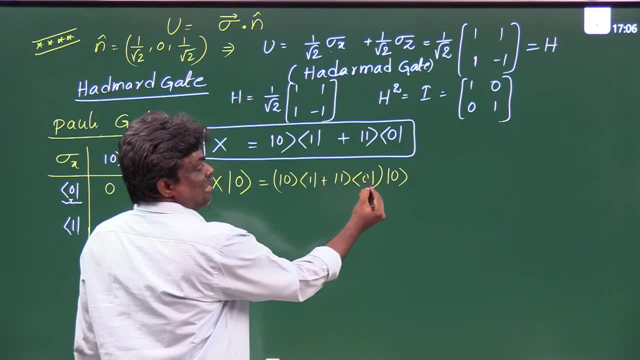 now this is multiplied with the zero. now this is multiplied with the zero. can you please tell me? can you please tell me? can you please tell me? so see here: a zero into zero is one. so see here: a zero into zero is one. so see here: a zero into zero is one. okay, just split it here. it is a bra. 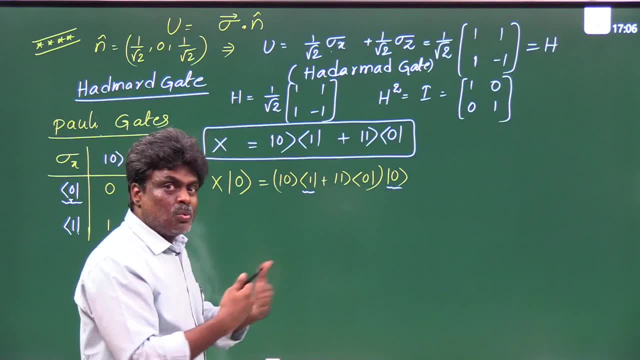 okay, just split it. here, it is a bra. okay, just split it here. it is a bra one. here it is a ket zero, one here, it is a ket zero one, here it is a ket zero. those two are abnormal basis. that's why those two are abnormal basis. that's why 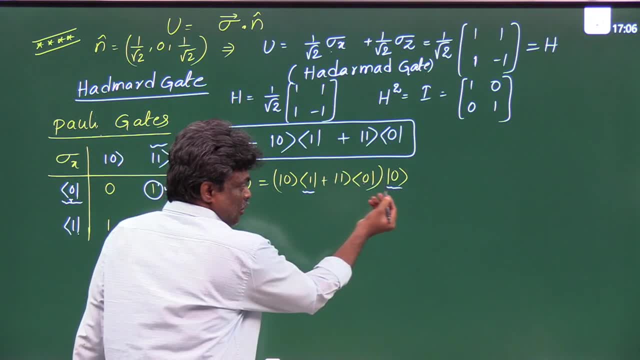 those two are abnormal basis. that's why this into this is a zero, this into this is a zero, this into this is a zero. and here: zero, zero one. so what's the? and here: zero, zero one. so what's the? and here: zero, zero one. so what's the remaining? 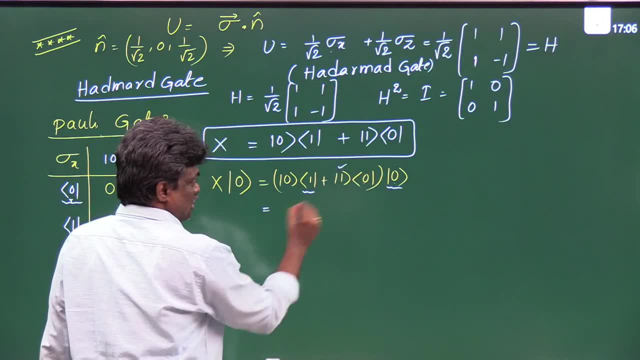 remaining, remaining one. so i hope you understand. so this is one, so i hope you understand. so this is one, so i hope you understand. so this is directly equal to one, directly equal to one, directly equal to one, because this into this is equal to one, because this into this is equal to one. 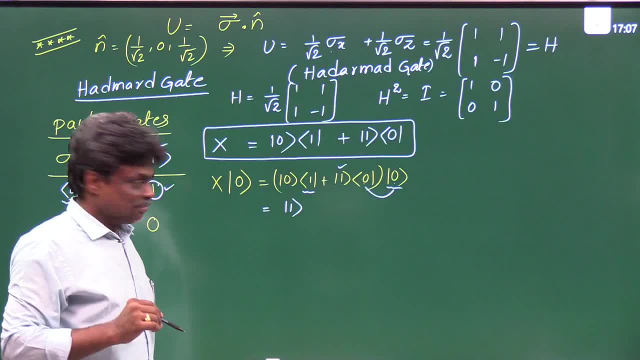 because this into this is equal to one. but this bra one and ket zero is equal. but this bra one and ket zero is equal. but this bra one and ket zero is equal to zero. to zero, to zero. so x operates on zero what you are, so x operates on zero what you are. 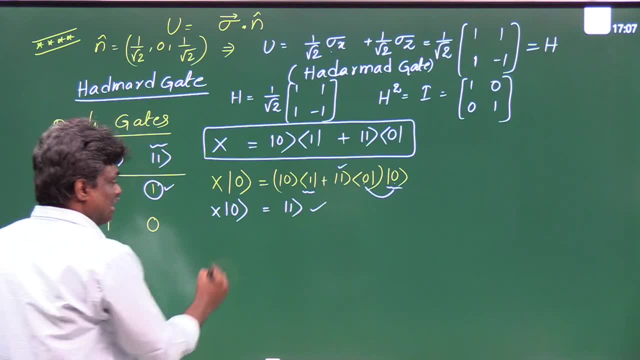 so x operates on zero. what you are getting getting getting one. wait a minute. this operation is given one. wait a minute. this operation is given one. wait a minute. this operation is given by, by, by. this is the representation of quantum. this is the representation of quantum. this is the representation of quantum. gate x: 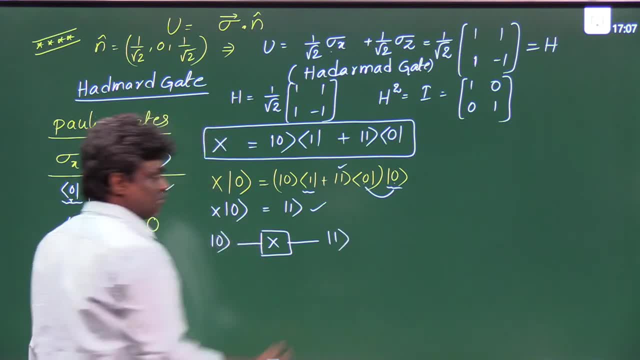 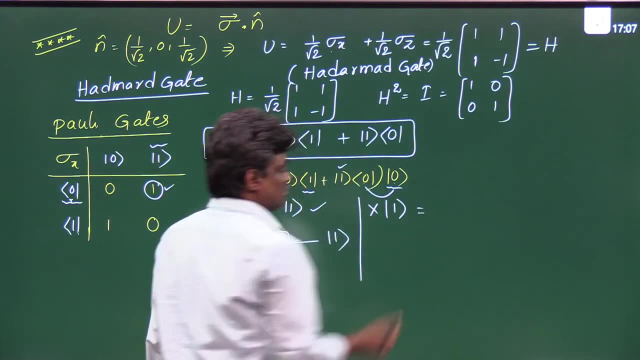 gate x, gate x: here we have zero state and we got one. here we have zero state and we got one. here we have zero state and we got one similarly. if you take similarly, if you take similarly, if you take x gate operates on ket one because we 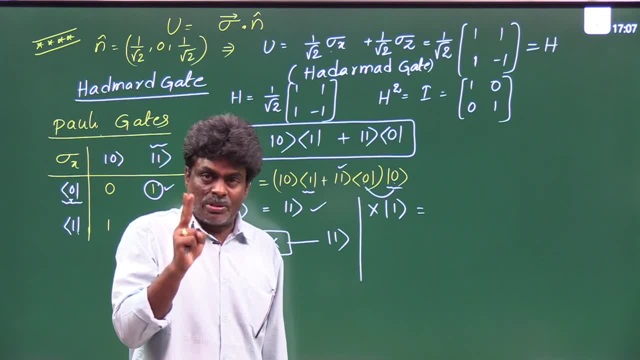 x gate operates on ket one. because we x gate operates on ket one because we have two qubit states, have two qubit states, have two qubit states, single qubits. two states are there. one is single qubits. two states are there. one is single qubits. two states are there. one is a zero, another is a one. let us operate. 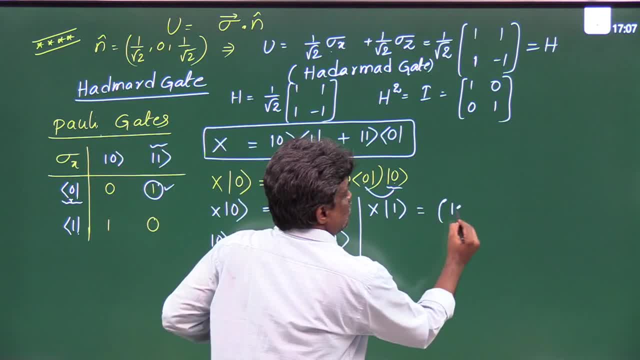 a zero, another is a one. let us operate a zero, another is a one. let us operate on that same thing. what is x on that same thing? what is x on that same thing? what is x- zero, one plus one, zero, one plus one, zero, one plus one, zero outer product. now this is going to 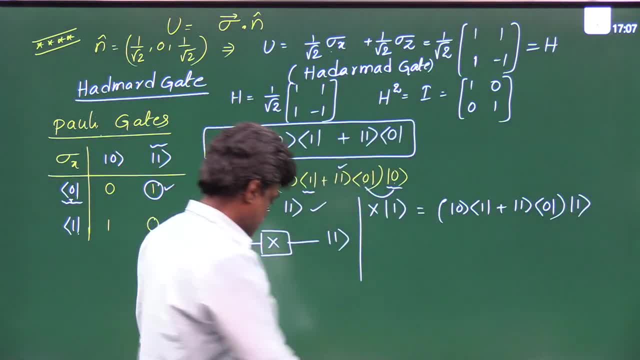 zero outer product. now this is going to zero outer product. now this is going to operate on, operate on, operate on. one so the same thing. one so the same thing. one so the same thing. so this product is equal to zero. so this product is equal to zero. 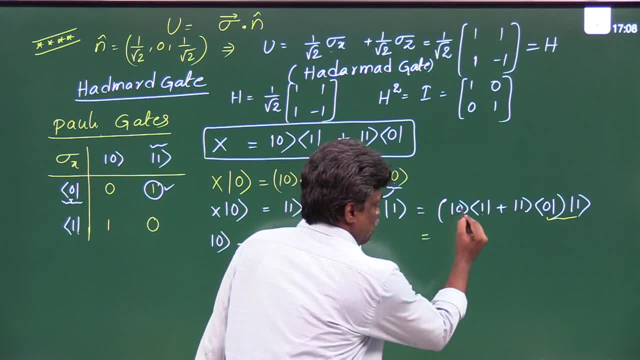 so this product is equal to zero, and one into one is one, and one into one is one, and one into one is one. so here we left with the zero. i hope you so. here we left with the zero, i hope you. so here we left with the zero. i hope you got it. 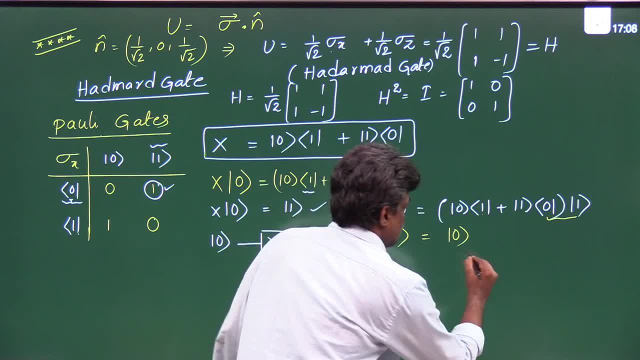 again. if you see uh the gate notation again, if you see uh the gate notation again, if you see uh the gate notation, this will be, this will be. this will be the pauli x gate. this is a quantum gate. the pauli x gate, this is a quantum gate. 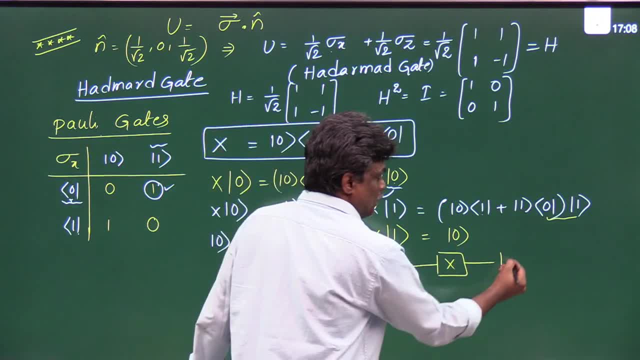 the pauli x gate. this is a quantum gate representation, representation, representation. we have one and it is a flip to zero. we have one and it is a flip to zero. we have one and it is a flip to zero which is quite similar to our classical, which is quite similar to our classical. 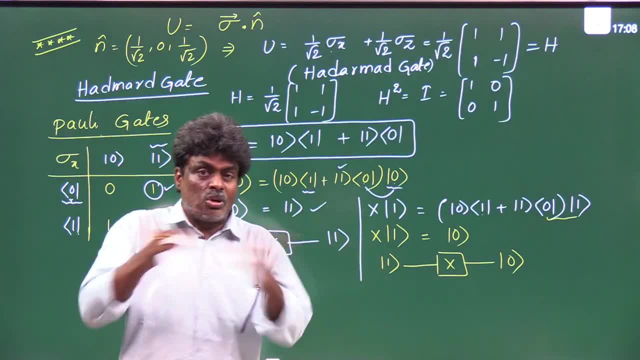 which is quite similar to our classical not gate, not gate, not gate. that also will flip zero to one, one to that also will flip zero to one. one to that also will flip zero to one. one to zero, zero, zero. so here also it is a flipping zero to. 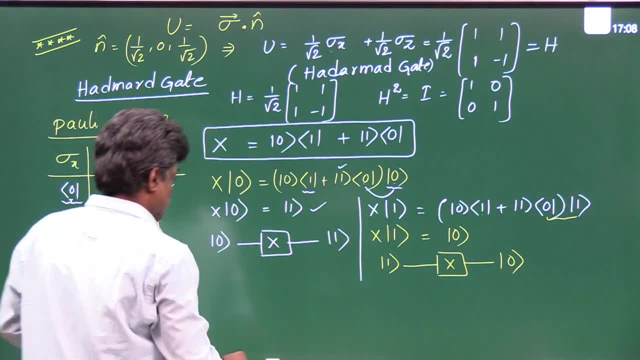 so here also it is a flipping zero to. so here also it is a flipping zero to one one to zero, one one to zero. so that means if you represent in a block, so that means if you represent in a block, so that means if you represent in a block sphere. 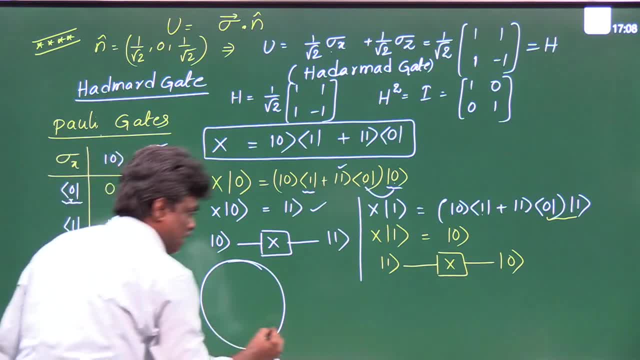 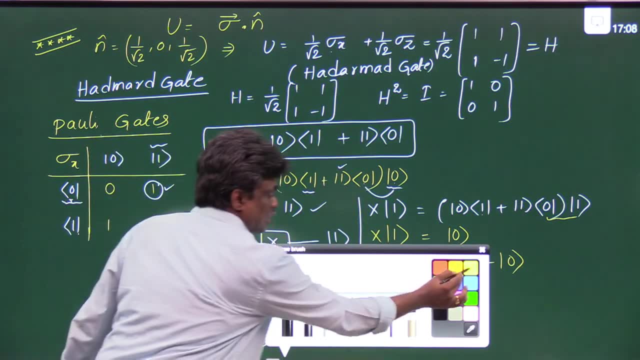 sphere sphere. so this is the block sphere. so this is the block sphere, so this is the block sphere. okay, so here i am applying x gate. okay, so here i am applying x gate. okay, so here i am applying x gate. everybody, please listen, everybody, please listen, everybody, please listen. so, for example, 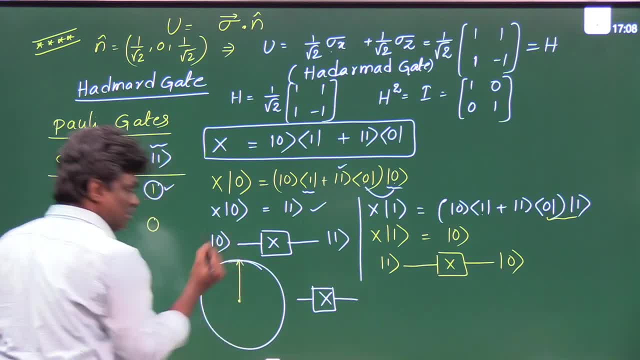 so, for example, so, for example, here initial state is zero, here initial state is zero, here initial state is zero. i told you already, the north pole is. i told you already, the north pole is. i told you already, the north pole is nothing but zero and the south pole is. 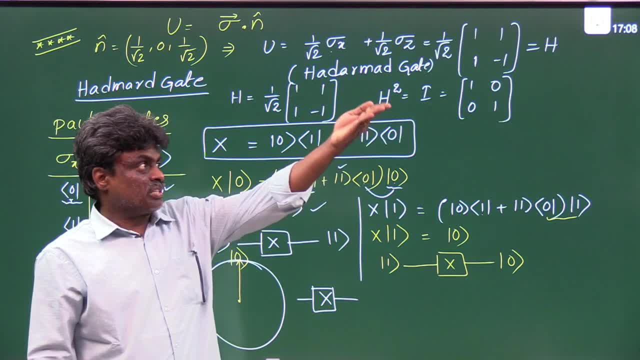 nothing but zero and the south pole is nothing but zero and the south pole is nothing but nothing but nothing but one. so north pole zero state will one. so north pole zero state will one. so north pole zero state will convert it to south. that means this: the 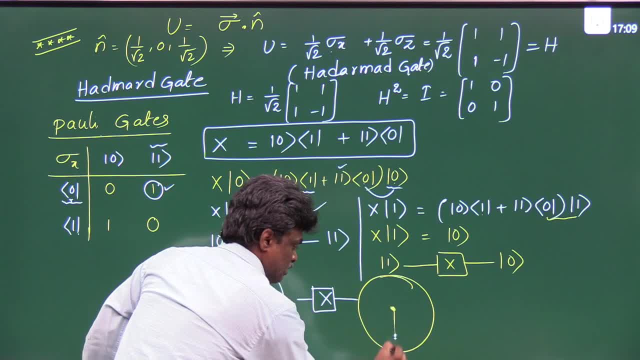 convert it to south. that means this: the convert it to south. that means this: the output will be on the block sphere. output will be on the block sphere. output will be on the block sphere like this, like this, like this. this is one. this is one. this is one, sorry. 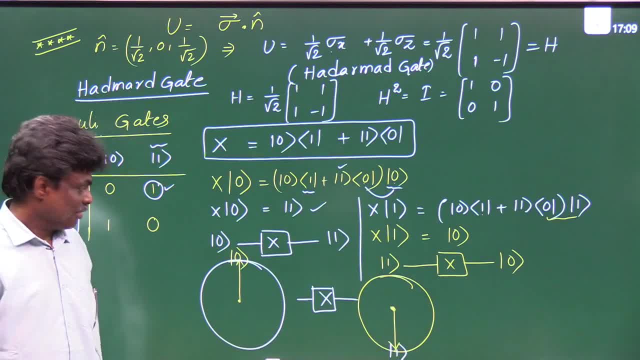 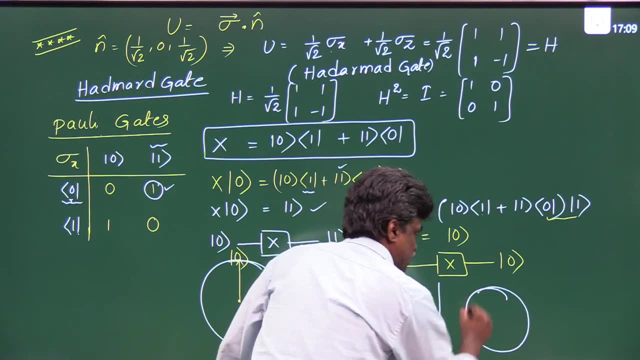 sorry, sorry, south state one. so similarly, if you take this uh this, so similarly, if you take this uh this, so similarly, if you take this uh this for this diagram, let me draw this, then for this diagram, let me draw this, then for this diagram, let me draw this, then you will get the clarity. 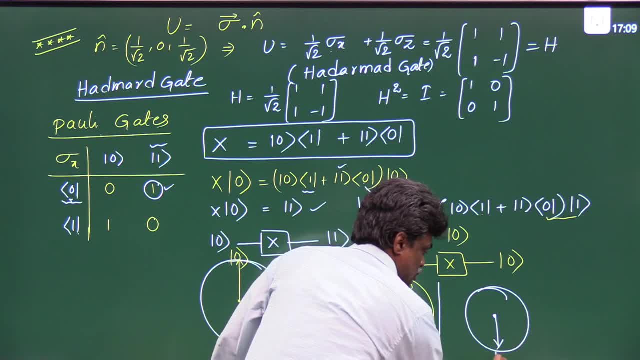 you will get the clarity. you will get the clarity: uh, this is the initial state. uh, this is the initial state. uh, this is the initial state. so, south south pole one. so south south pole one, so south south pole one. and again, here we have x gate, and again, here we have x gate. 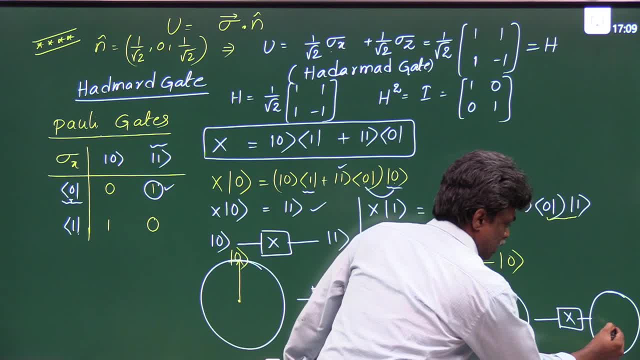 and again, here we have x gate. so what it is doing is so what it is doing? is so what it is doing is what it is performing? uh, this is what it is performing. uh, this is what it is performing. uh, this is converted to, converted to, converted to this north pole. 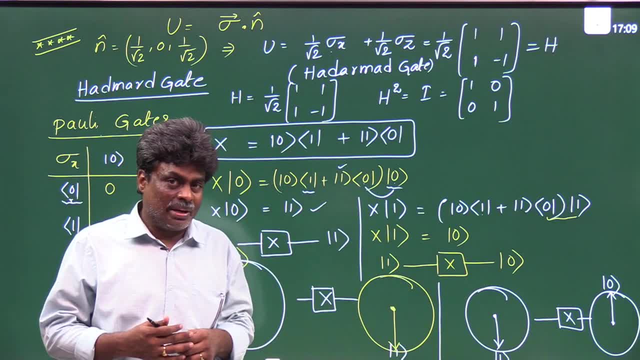 so did you observe one thing? so did you observe one thing? so did you observe one thing: what this not gate is doing, what this not gate is doing, what this not gate is doing, this is called not gate. actually this, this is called not gate. actually this, this is called not gate. actually this. this is nothing but. 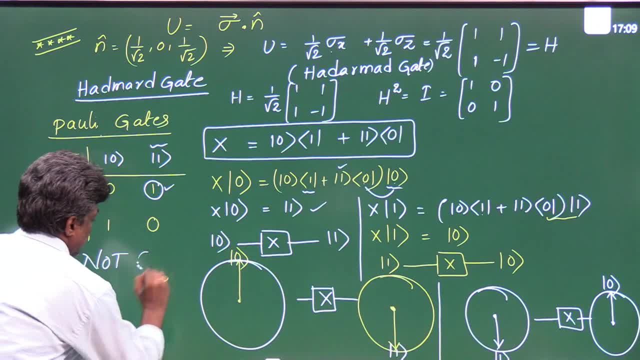 this is nothing, but this is nothing but quantum: uh, not gate. we call it as not quantum, uh, not gate. we call it as not quantum, uh, not gate. we call it as not gate, gate, gate, but quantum. so the quantum, not gate, is nothing but uh. so the quantum, not gate, is nothing but uh. 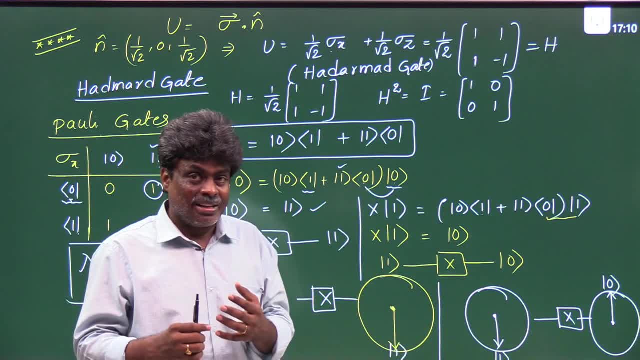 so the quantum, not gate, is nothing, but uh, probably x gate, probably x gate, probably x gate. so what it is doing, so what it is doing, so what it is doing, it is uh, flipping zero to one, one to zero. it is uh flipping zero to one, one to zero. 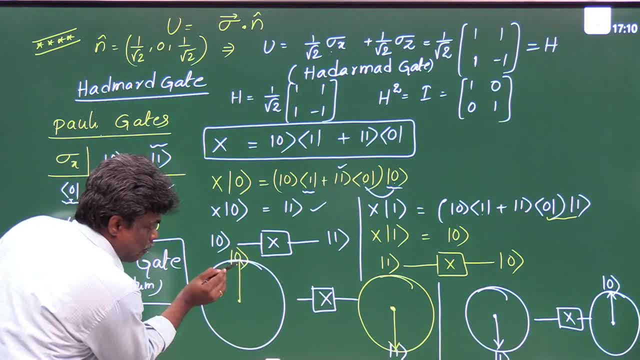 it is, uh, flipping zero to one, one to zero. so so so, and one more thing, if you observe you, and one more thing, if you observe you, and one more thing, if you observe you have taken a point here, have taken a point here, have taken a point here. after applying x gate, you got this point. 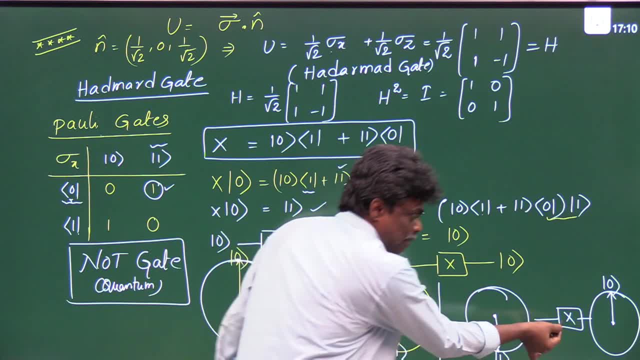 after applying x gate. you got this point. after applying x gate. you got this point and your initial state is this one. and your initial state is this one and your initial state is this one after applying x gate. you got this point. after applying x gate. you got this point. can you please tell me these two? 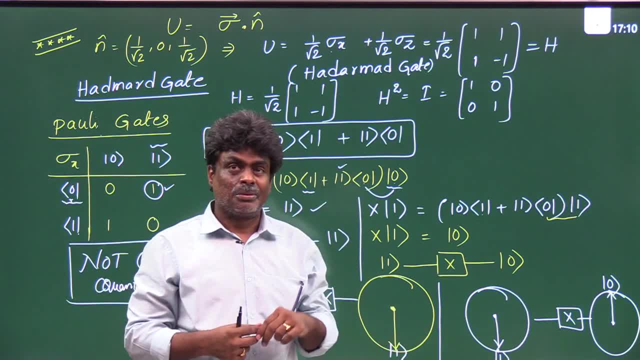 can you please tell me these two? can you please tell me these two points are opposite points or not, points are opposite points or not, points are opposite points or not. yes, yes, yes, oh, oh, oh, generally, generally, generally. quantum not gate, quantum not gate, quantum not gate. must i mean quantum not gate? operation. 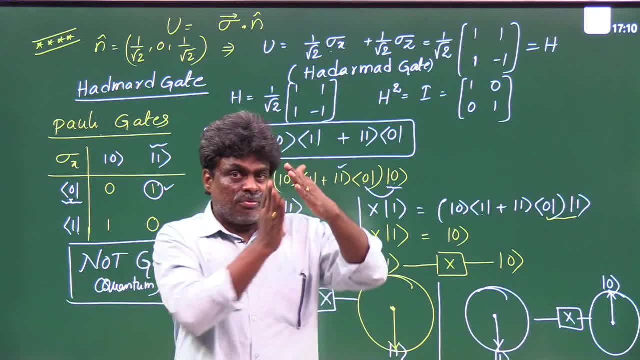 must i mean quantum, not gate operation? must i mean quantum, not gate operation? is what it has to? is what it has to? is what it has to change. uh, if you have a point on the block, change. uh, if you have a point on the block, change. uh, if you have a point on the block sphere, it will convert to the opposite. 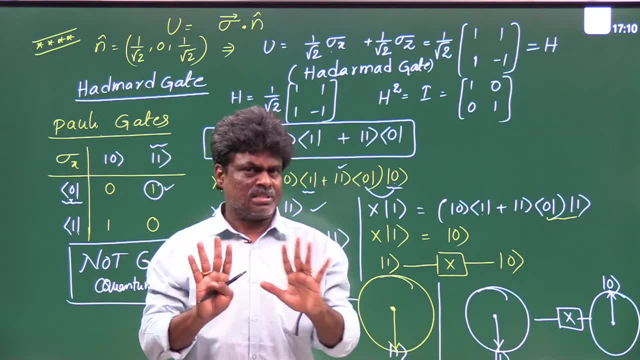 sphere. it will convert to the opposite sphere. it will convert to the opposite point, quite exactly opposite point. you point quite exactly opposite point. you point quite exactly opposite point. you have to get that is a general operation. have to get that is a general operation. have to get that is a general operation. let us discuss more. so i hope you. 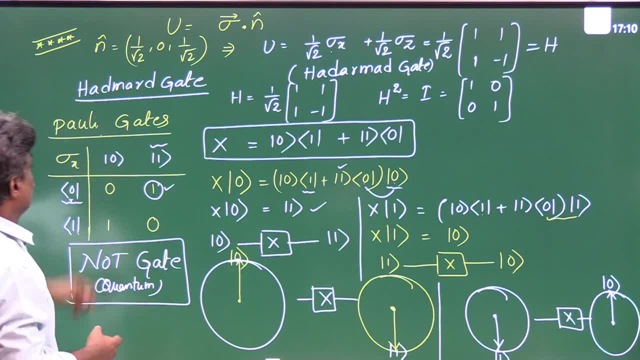 let us discuss more. so i hope you let us discuss more. so i hope you understand this. come on, understand this. come on, understand this. come on. next one: what you do, sigma y, of course. next one, what you do, sigma y, of course. next one, what you do, sigma y, of course. no need to draw the diagrams, at least. 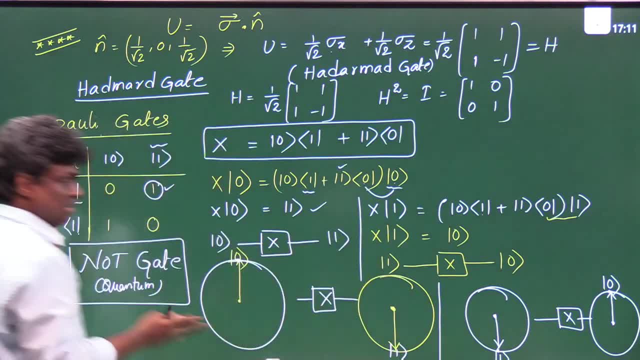 no need to draw the diagrams. at least. no need to draw the diagrams, at least write the outer product and write this. write the outer product and write this. write the outer product and write this: gates. okay, please try yourself, otherwise i will explain trouble. i will explain the second one. 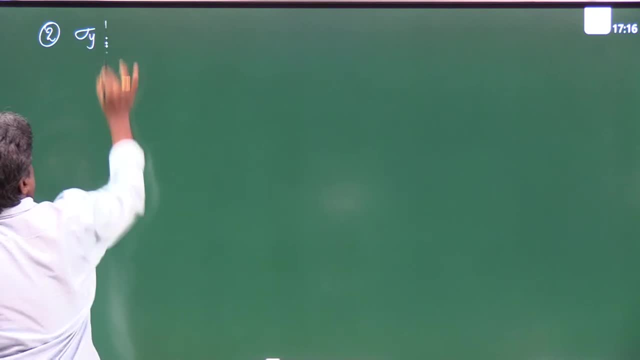 trouble. i will explain the second one trouble. i will explain the second one also. also. also sigma y. so if you take the sigma y, sigma y, so if you take the sigma y, sigma y, so if you take the sigma y, matrix zero minus i, iota zero, this is 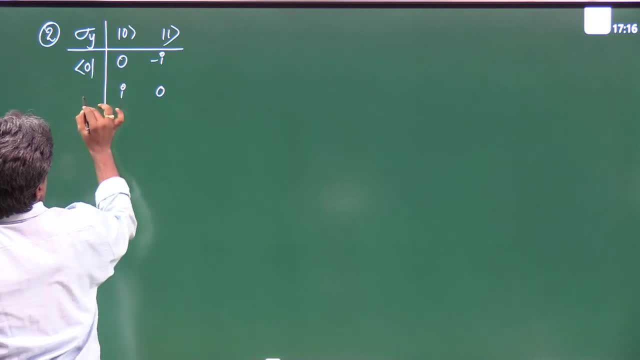 matrix zero minus i iota zero. this is matrix zero minus i iota zero. this is, these are the basis states. i told you these are the basis states. i told you, these are the basis states. i told you already what are the basis states already, what are the basis states. 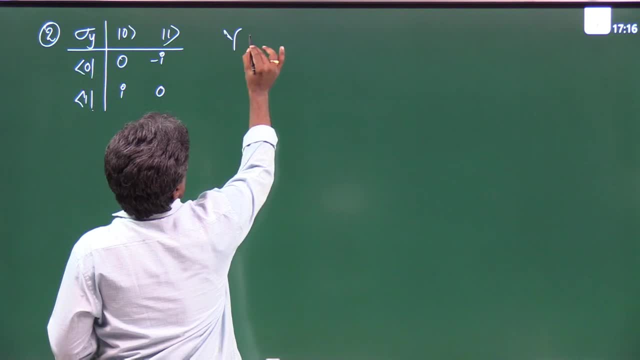 already. what are the basis states right now? here i'm writing the outer. right now, here i'm writing the outer. right now, here i'm writing the outer: product form, product form. product form. that means this is my quantum gate y. that means this is my quantum gate y. 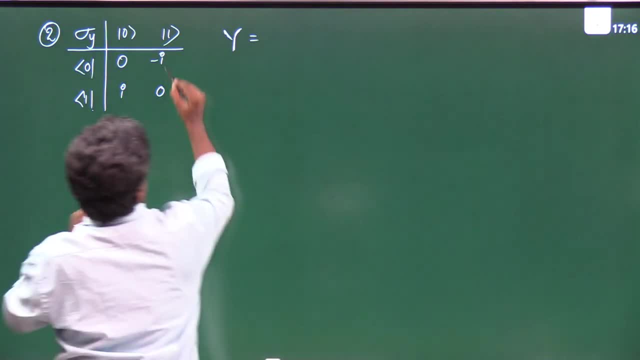 that means this is my quantum gate y. don't write sigma y, please write it as a. don't write sigma y, please write it as a. don't write sigma y, please write it as a y okay. so here we have non-zero, non-zero, y. okay, so here we have non-zero, non-zero. 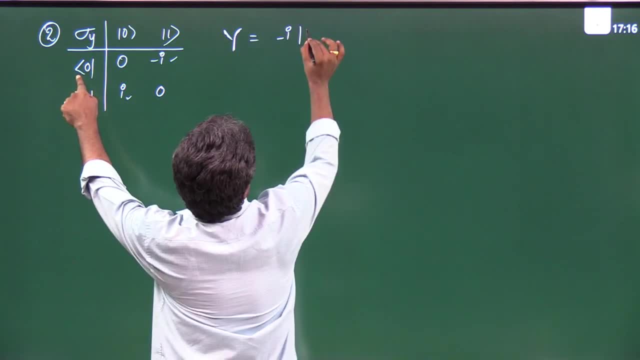 y okay, so here we have non-zero, non-zero. that's why minus iota, that's why minus iota, that's why minus iota: ket become sorry, ket become sorry. ket become sorry, bra become ket, bra become ket, bra become ket. and the ket become bra like this and the ket become bra like this. 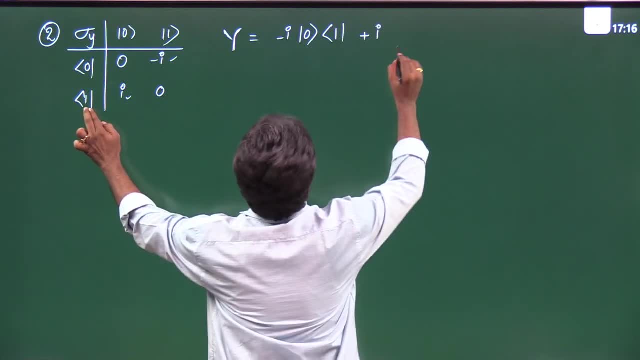 and the ket become bra like this: and a plus iota and a plus iota and a plus iota. write this bra vector as a ket vector. write this bra vector as a ket vector. write this bra vector as a ket vector. write the corresponding ket vector as a. write the corresponding ket vector as a. 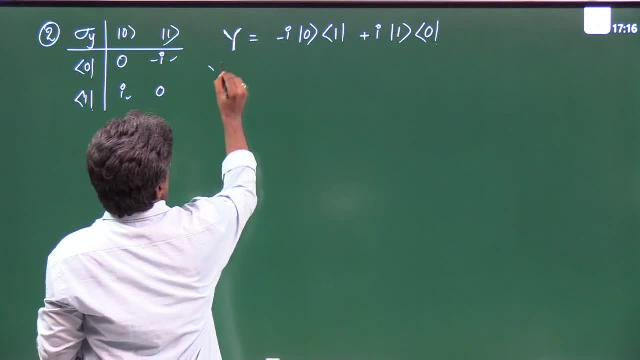 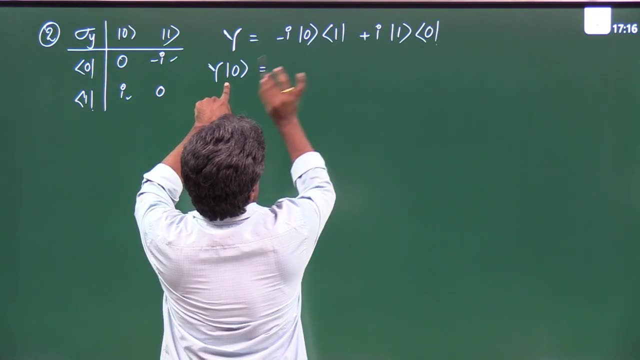 write the corresponding ket vector as a bra vector. that's it, bra vector. that's it bra vector. that's it now, now. now, y operates on zero, y operates on zero, y operates on zero. so i hope you understand, so, i hope you understand, so i hope you understand this is the bra one- into ket: zero, zero. 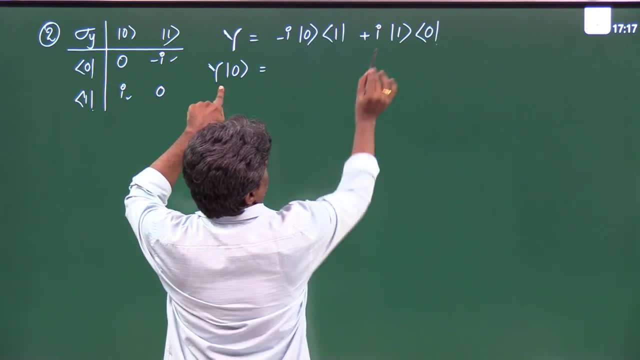 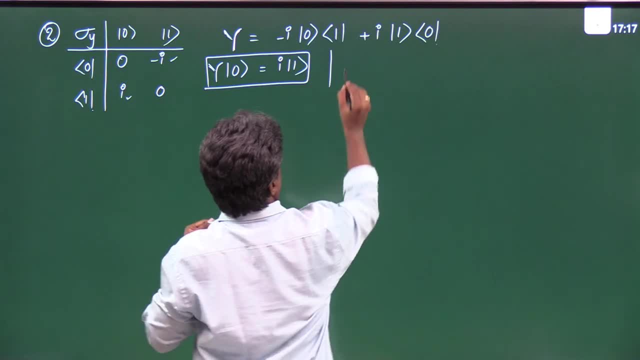 with the iota one did you observe? with the iota one, did you observe? i have not written completely directly. i have not written completely directly. i have not written completely directly. i'm writing because we already discussed. i'm writing because we already discussed. i'm writing because we already discussed, still not understanding. 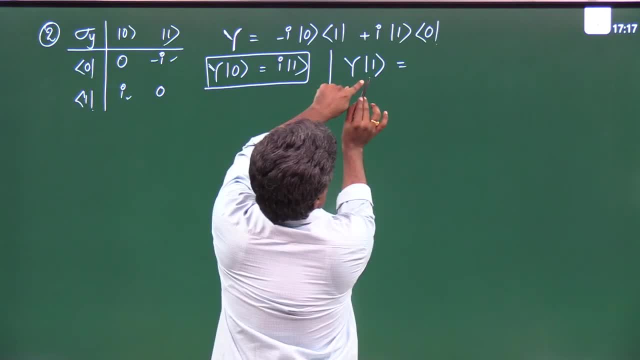 still not understanding. still not understanding. then y operates on one, then y operates on one, then y operates on one. so this is a ket one multiplied with. so this is a ket one multiplied with. so this is a ket one multiplied with bra one. bra one, ket one is one. 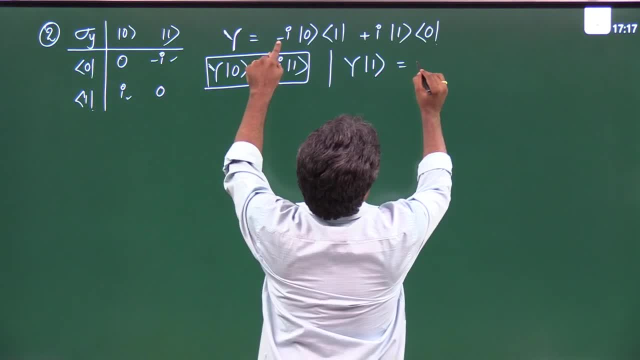 bra one. bra one. ket one is one bra one bra one. ket one is one bra zero. ket one is zero. that's why you're bra zero. ket one is zero, that's why you're bra zero. ket one is zero. that's why you're left with. 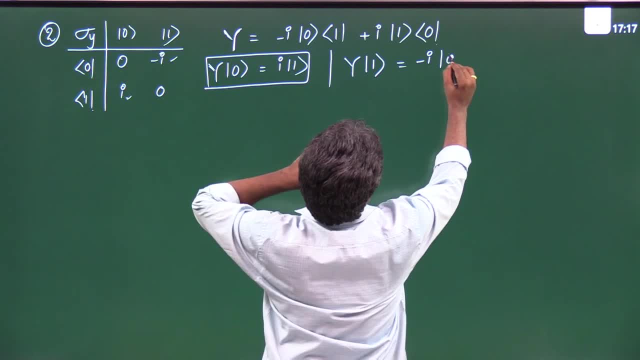 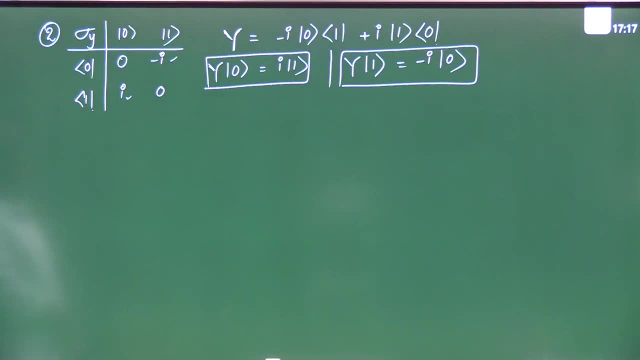 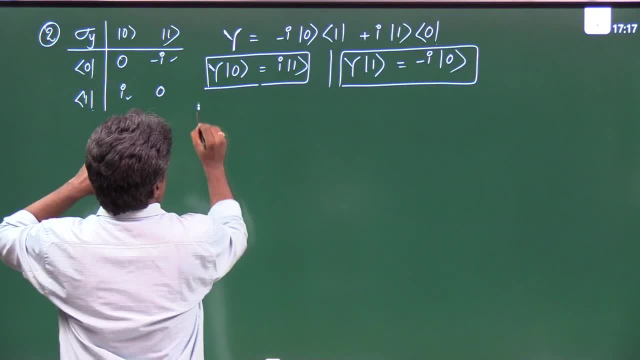 you have zero. how to represent this quantum gate in the notation? this is the quantum gate in the notation. this is the quantum gate in the notation. this is the initial state, initial state, initial state, and here we have quantum gate y and what, and here we have quantum gate y and what. 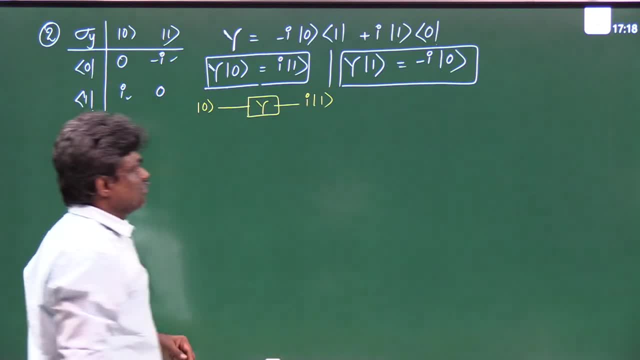 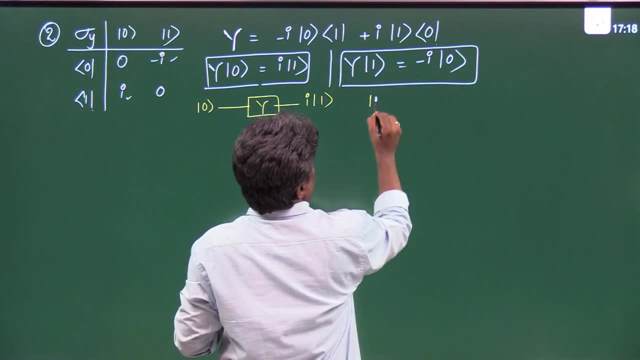 and here we have quantum gate y. and what is its operation? is its operation? is its operation? i iota 1, that means a zero state. i iota 1, that means a zero state. i iota 1, that means a zero state. ket 0 become i into ket 1. similarly, 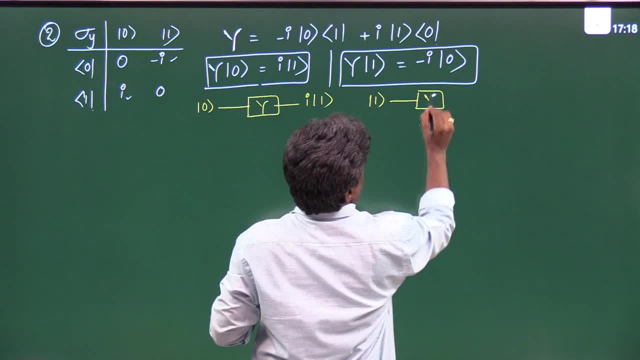 ket 0 become i into ket 1. similarly, ket 0 become i into ket 1. similarly ket 1- initial state. we have this y ket 1 initial state. we have this y ket 1 initial state. we have this: y gate, that is, gate, that is. 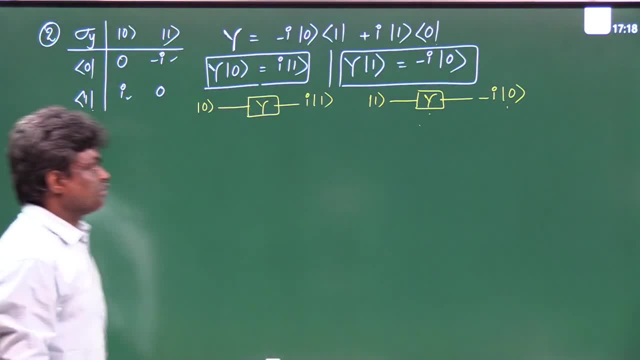 gate. that is minus iota, minus iota, zero. similarly can you write that zero. similarly can you write that zero. similarly can you write that: z matrix sigma j make it fast. z matrix sigma j, make it fast. z matrix sigma j, make it fast. so one zero, zero minus one. 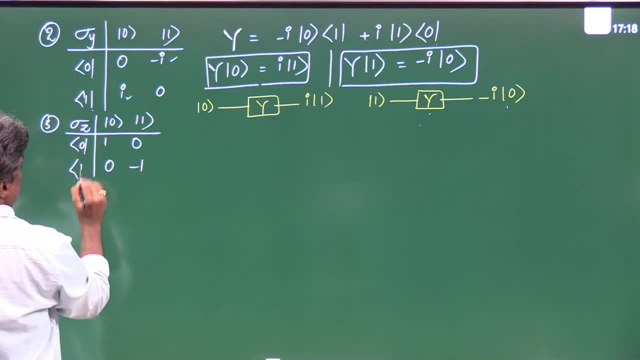 so one zero zero minus one. so one zero zero minus one ket zero ket one ket zero. sorry bra zero ket zero. ket one ket zero. sorry bra zero ket zero. ket one ket zero. sorry bra zero. bra one bra one bra one. so here z is equal to. 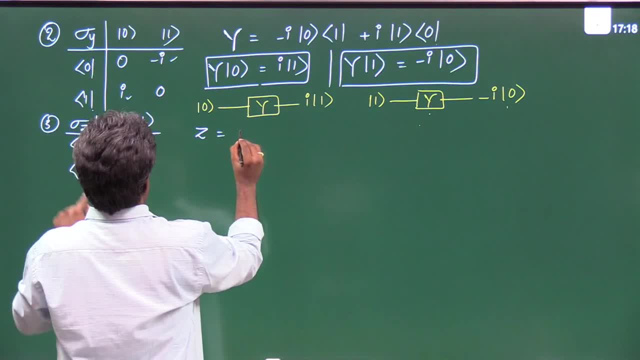 so here z is equal to, so here z is equal to. this is a non-zero and this is a non-zero. this is a non-zero and this is a non-zero, this is a non-zero and this is a non-zero. that's why. that's why. 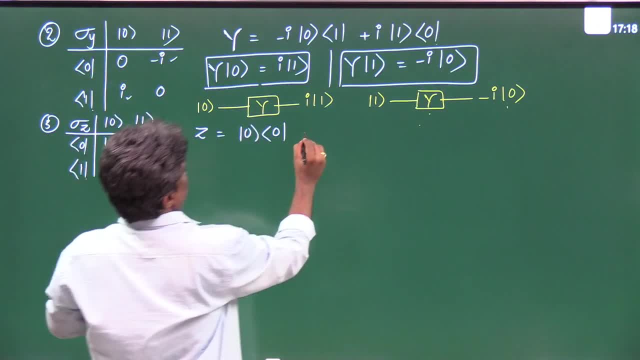 that's why bra zero, bra zero, bra zero, ket zero. here it is a minus ket zero. here it is a minus ket zero. here it is a minus minus. you have to take minus, also minus. you have to take minus, also minus. you have to take minus also, because this is the element minus one. 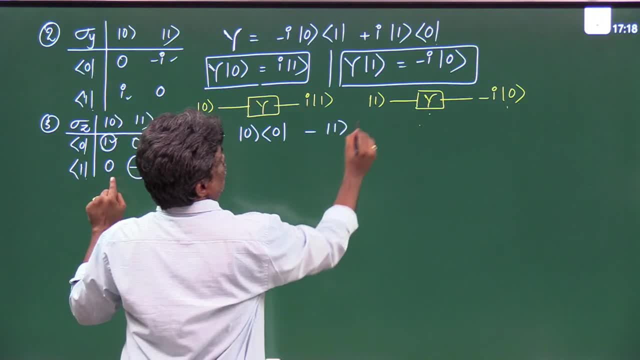 because this is the element minus one, because this is the element minus one. this is the element one, this is the element one, this is the element one. so bra one, so bra one, so bra one, ket one. i hope you are doing. ket one, i hope you are doing. 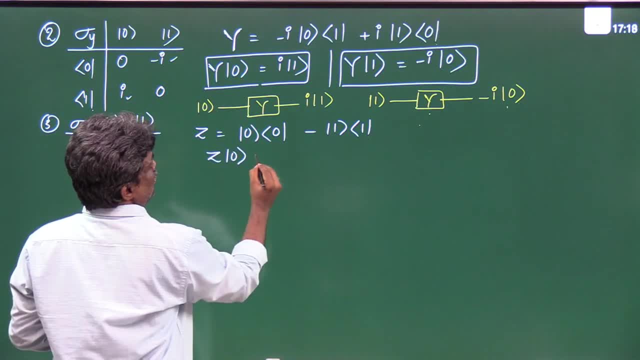 ket one. i hope you are doing so now. let us see the operation z. so now, let us see the operation z. so now let us see the operation z. operates on zero, operates on zero, operates on zero. so z means this entire thing you have to. so z means this entire thing you have to. 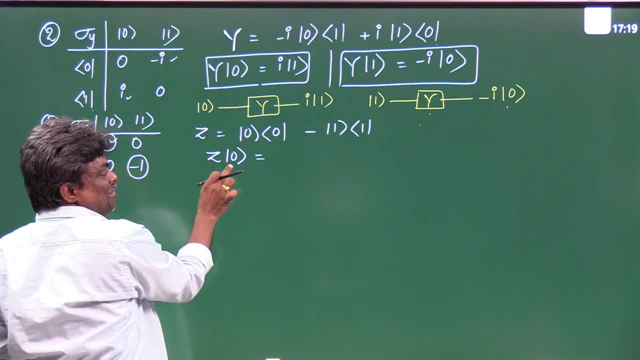 so z means this entire thing you have to write. once you have written this write. once you have written this write, once you have written this, you are multiplying with the ket zero. you are multiplying with the ket zero. you are multiplying with the ket zero. this is the first one multiplied with. 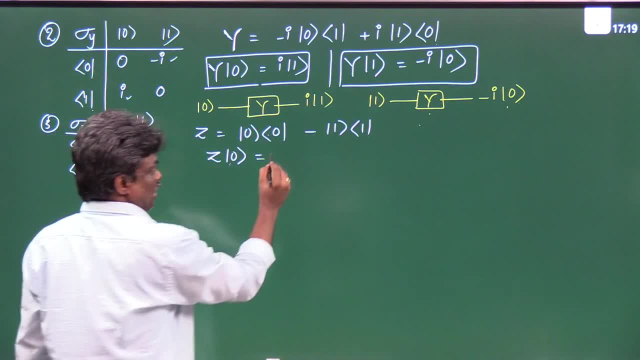 this is the first one multiplied with. this is the first one multiplied with: the ket zero, bra zero. the ket zero, bra zero. the ket zero, bra zero, ket zero. how much one? that's why zero, ket zero. how much one that's why zero, ket zero. how much one that's why zero? no change. 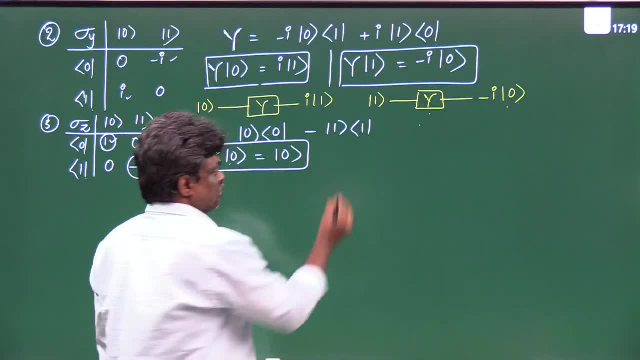 no change, no change. next one, sir. what happened to second one? next one, sir. what happened to second one? next one, sir. what happened to second one? second one is zero. second one is zero. second one is zero. now z operates on one. are you observing? now z operates on one. are you observing? 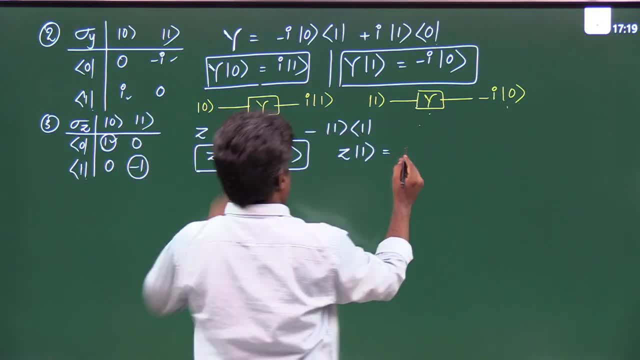 now, z operates on one. are you observing? z operates on one. you can write this: z operates on one. you can write this: z operates on one. you can write this entire thing. if you are not entire thing, if you are not entire thing, if you are not understanding what i am saying, is you? 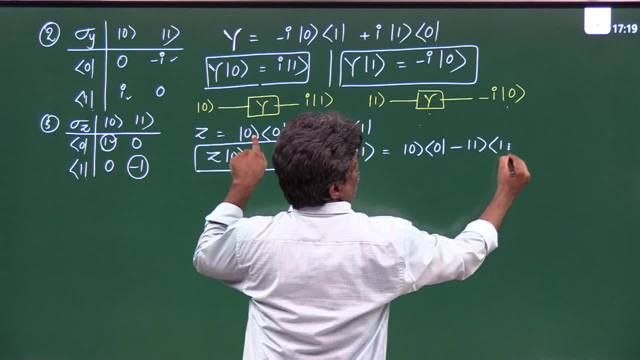 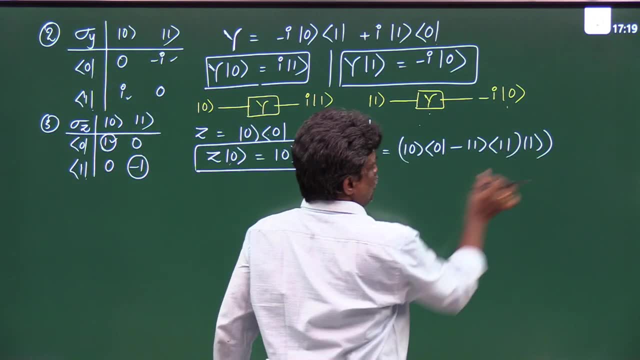 understanding what i am saying? is you understanding what i am saying? is you please write this? don't compromise, just write that into one. don't compromise, just write that into one. don't compromise, just write that into one. you know now. you know now. you know now. so this product is equal to one and this 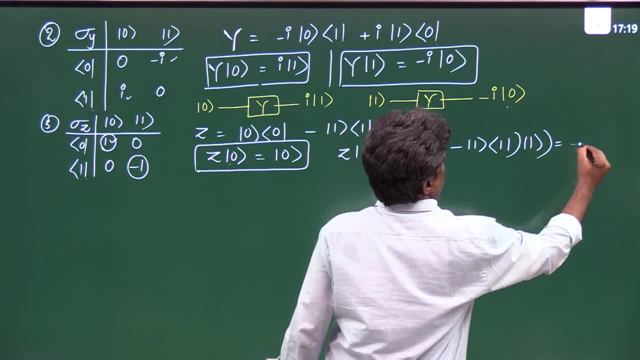 so this product is equal to one. and this, so this product is equal to one. and this into this is a zero. into this is a zero. into this is a zero. so this is equal to minus ket one. so this is equal to minus ket one. so this is equal to minus ket one. so 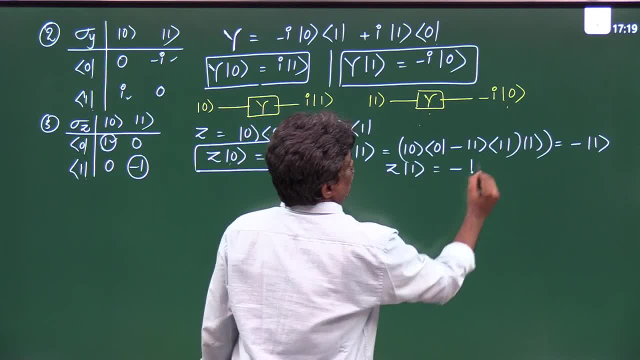 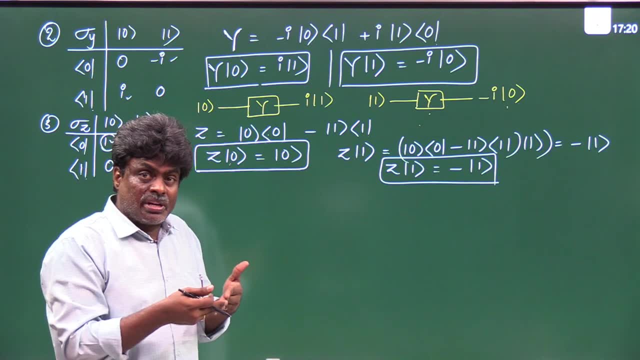 so. so here z operates on one, we got minus one. here z operates on one, we got minus one, here z operates on one, we got minus one. so what happened, sir, whenever pauli z? so what happened, sir, whenever pauli z? so what happened, sir, whenever pauli z gate operates on zero state? you are 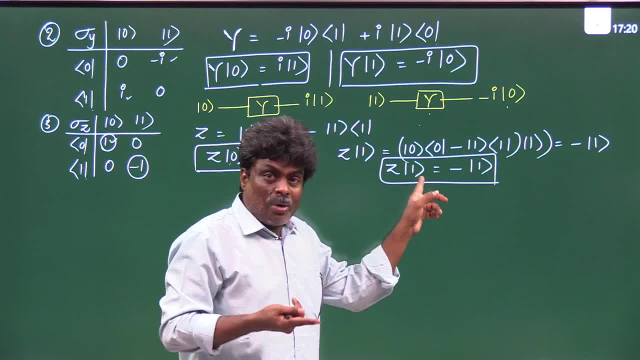 gate operates on zero state, you are gate operates on zero state. you are getting the same state, no change. getting the same state, no change. getting the same state, no change, but whenever it is operating on one state, but whenever it is operating on one state, but whenever it is operating on one state, we are getting some phase change. 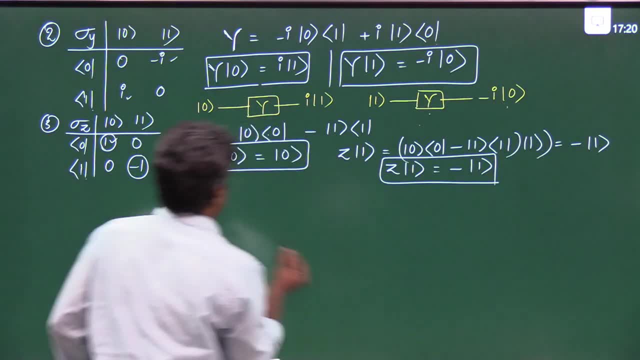 we are getting some phase change. we are getting some phase change. some phase change okay. some phase change okay. some phase change, okay. so, so, so, notation: this is the z gate notation notation. this is the z gate notation notation: this is the z gate notation, quantum z gate. 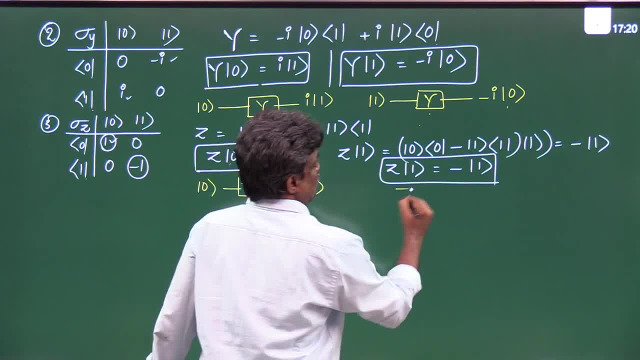 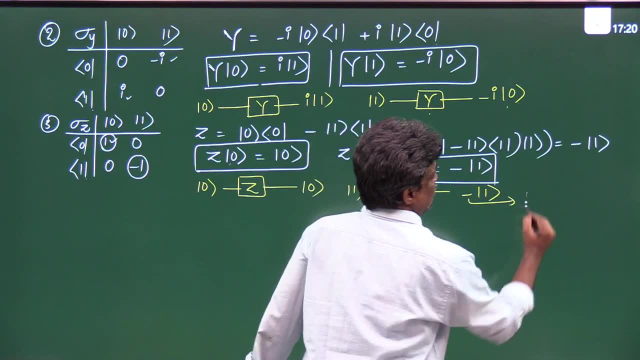 quantum z gate, quantum z gate. so zero, no change. but so zero, no change. but so zero, no change. but whenever it operates on, whenever it operates on, whenever it operates on one, you will get the phase change one, you will get the phase change one, you will get the phase change minus. 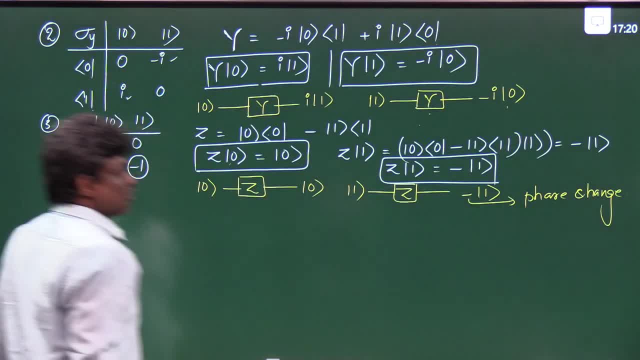 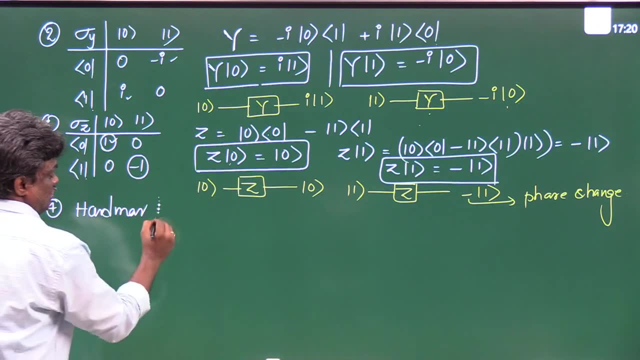 that's good. and the next, the most, that's good. and the next the most, that's good. and the next, the most important thing: the fourth, one important thing. the fourth, one important thing. the fourth one: head mod gate. head mod gate- yes, ready. i hope you have completed this. 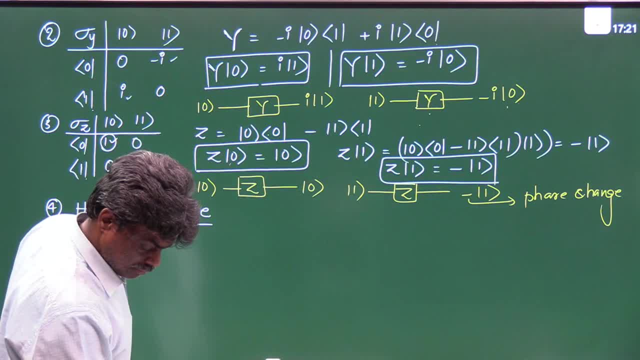 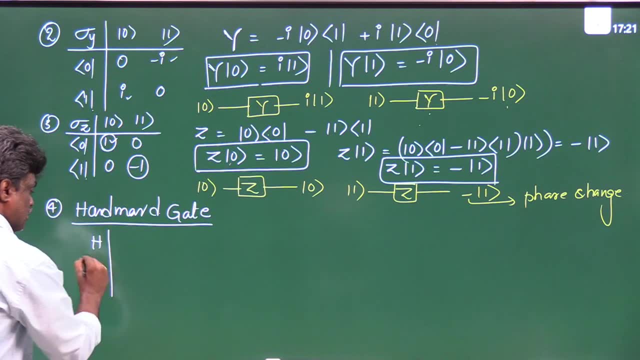 yes, ready, i hope you have completed this. yes, ready, i hope you have completed this. shall i wait are completed. So please write this outer product form for head mod gate H. So here we have 1, this is also 1, 1, minus 1, this is ket 0, ket 1, bra 0, bra 1.. 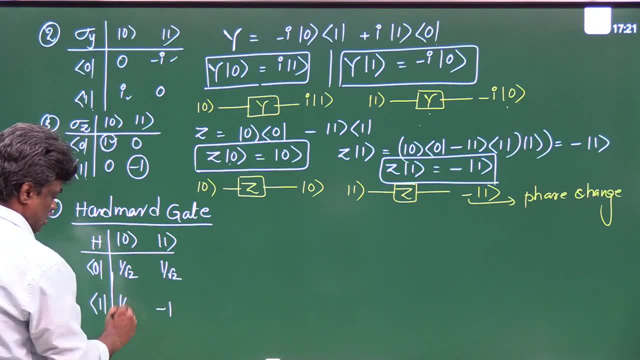 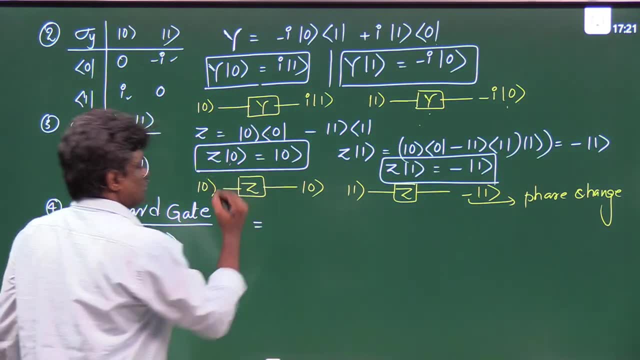 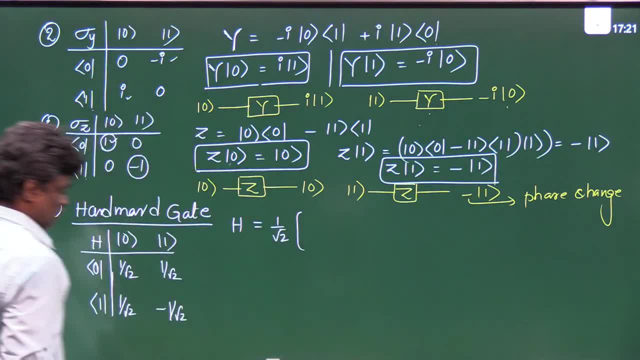 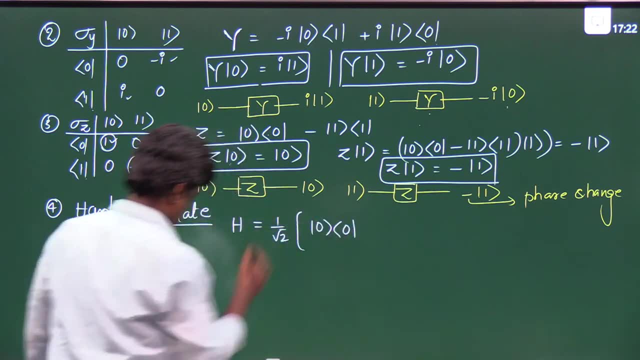 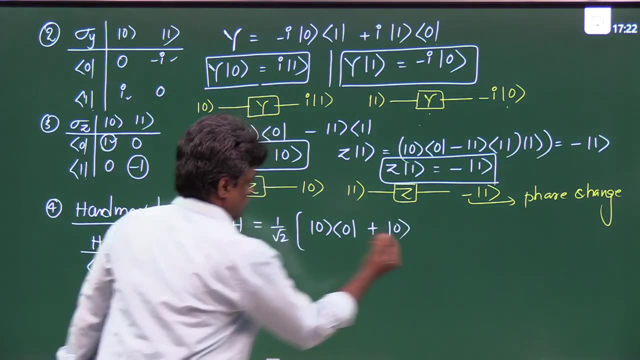 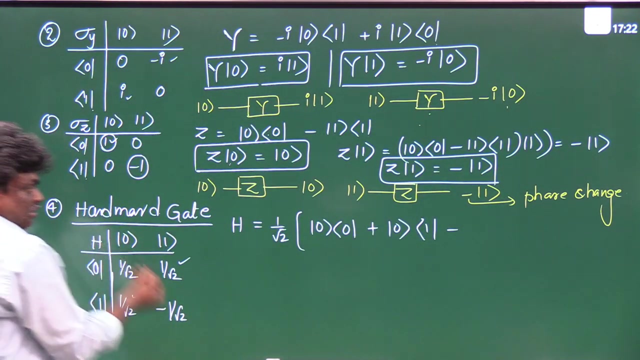 So I am taking 1 by root, 2 common. So this will become ket, this will become bra: 0, 0.. Next, I am taking again plus This element. I am taking: this become ket and this become bra. Next, I am taking this element. this is also plus. 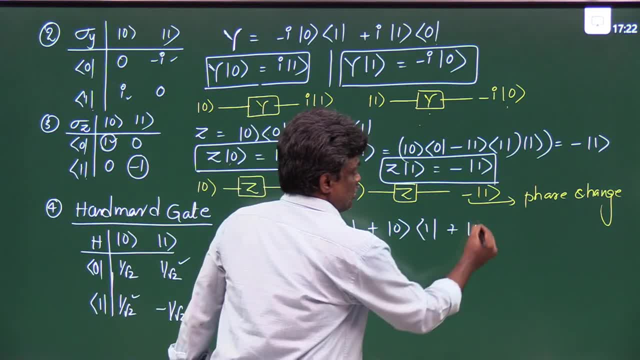 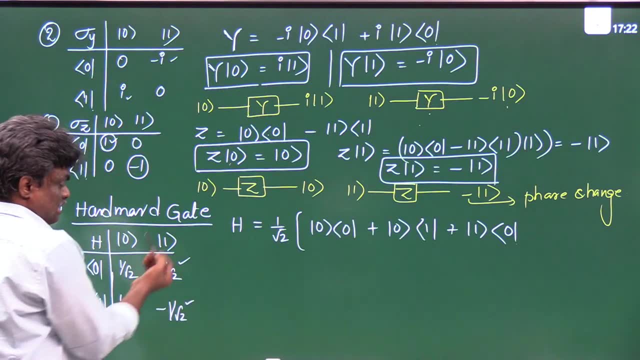 Here, the corresponding bra vector will become ket vector and the corresponding ket vector become bra vector. and the last and final, this is the minus, and this is nothing but 1, 1.. Now, please try yourself, because you will get interest. please do it. 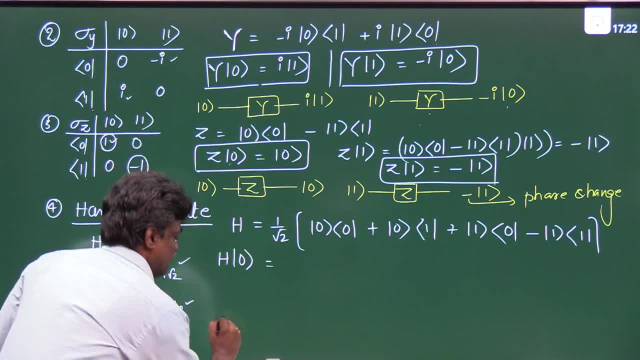 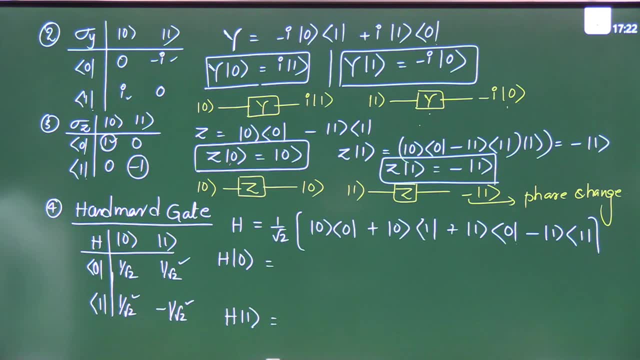 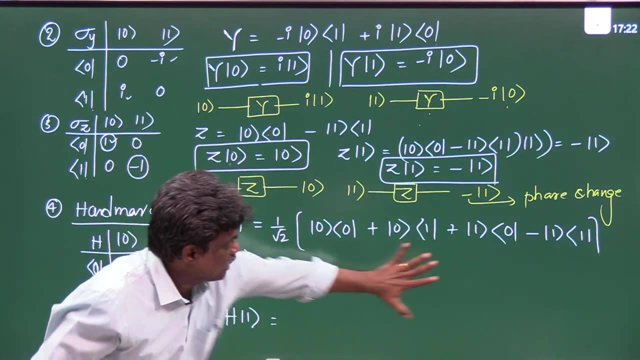 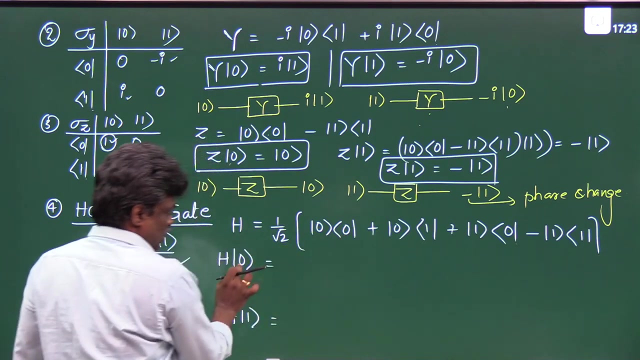 Now, H operates on 0, tell me what you are getting. H operates on 1, what you are getting, please do it. See whatever you have done here, the same thing, please do it. So you have to multiply with the ket vector 0, bra 1, ket 0, sorry. bra 0, ket 0, bra. 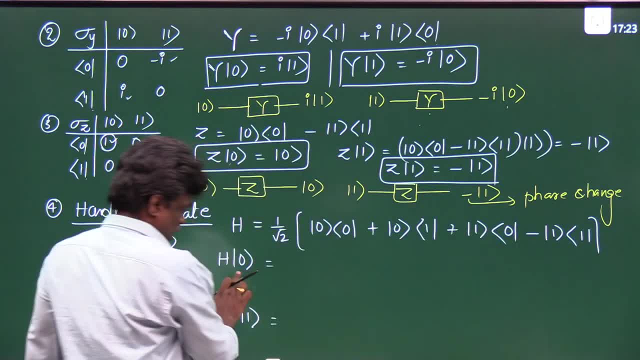 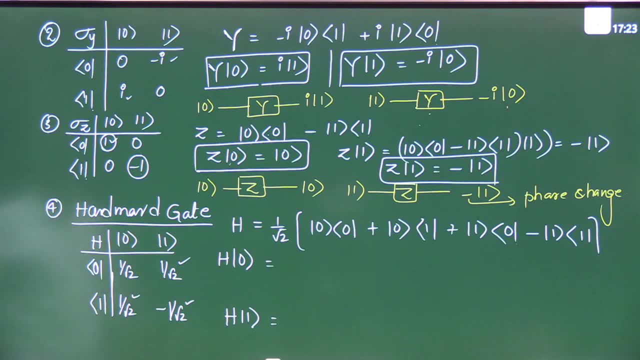 1, ket 0.. Whatever 0, leave it, and whatever the non-zero, please take it. Write yourself: Now you are writing this Hadamard gate operation: when Hadamard gate is operating on 0, state what you are getting. and Hadamard gate operates on 1, what you are getting. please do it. 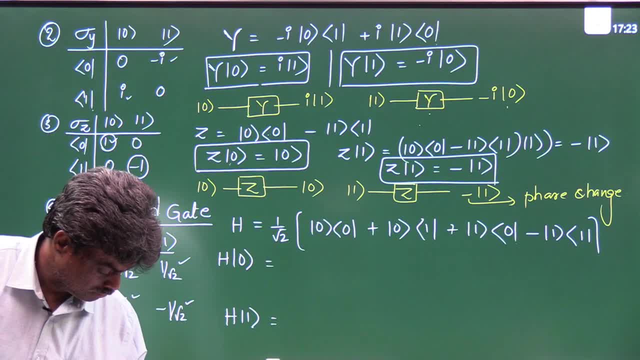 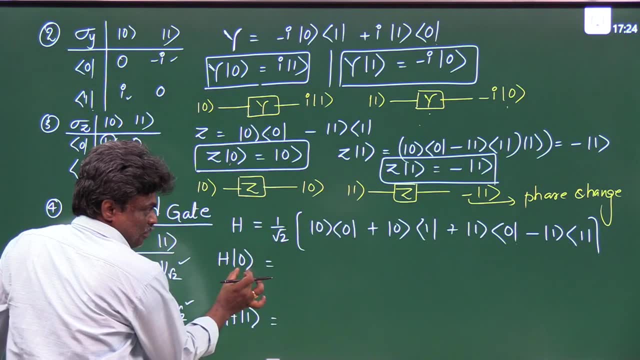 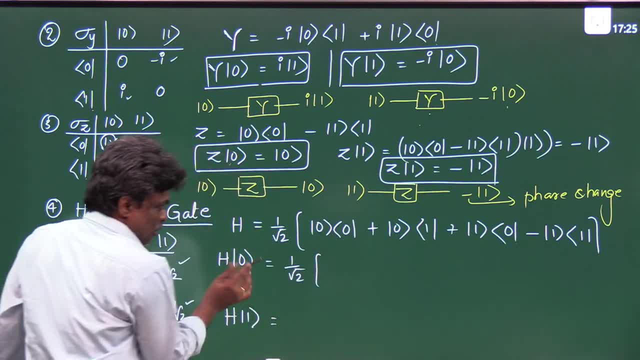 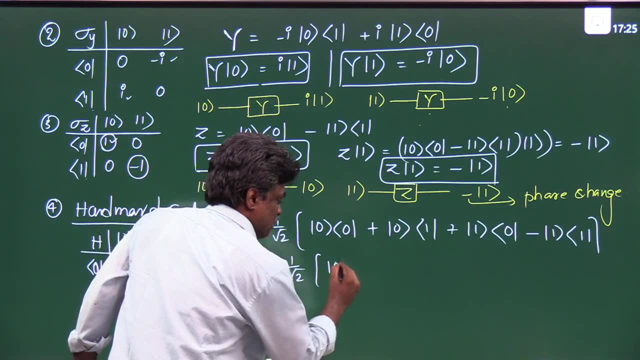 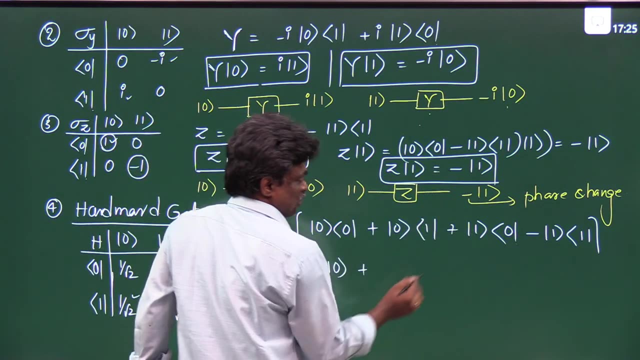 So 1 by root 2, first term. Are you observing? take this, take this ket 0, and write here: So this is equal to 1, we left with 0.. Plus, take this ket 0 and multiply here 0.. 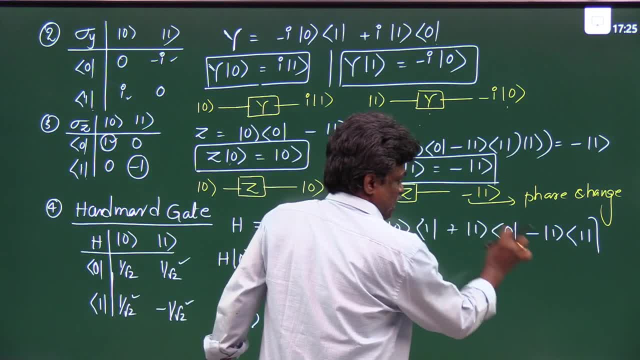 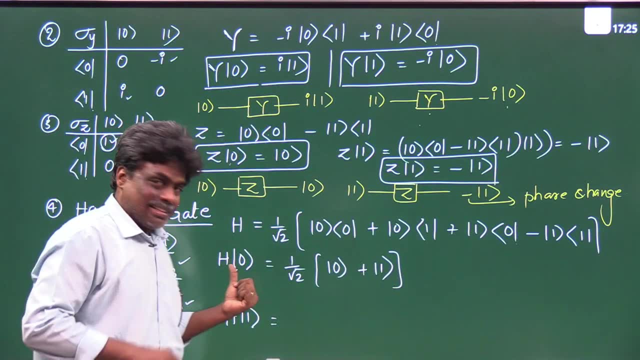 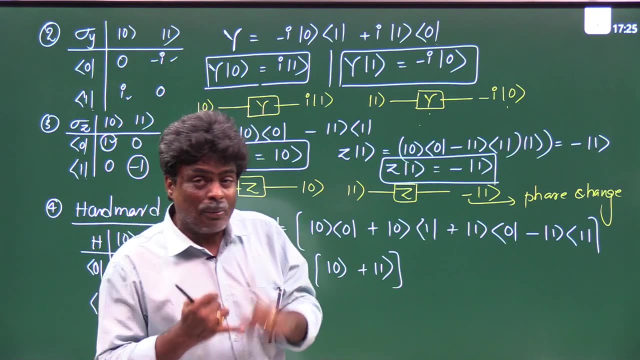 Next, Take this 0. And multiply here. play here here one, so the remaining is one. oh, that's good, we got the Hadamard gate. this is a very important which creates the superposition. state earlier that Pauli gates, what they have given, they have given a single qubits. but the 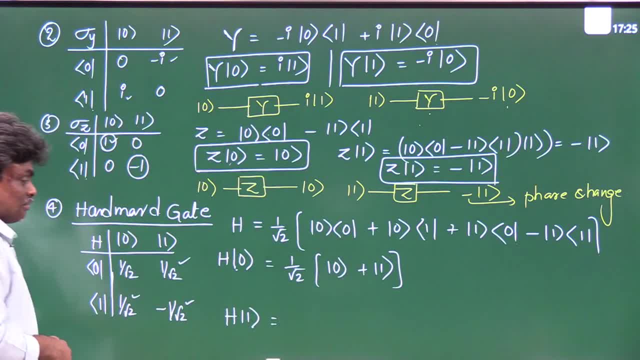 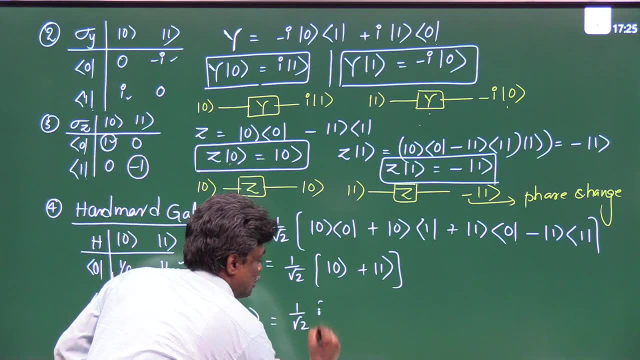 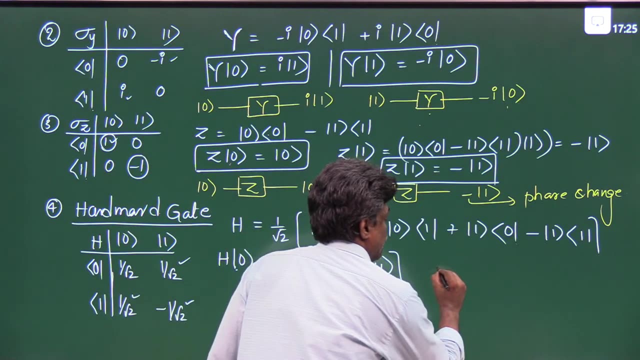 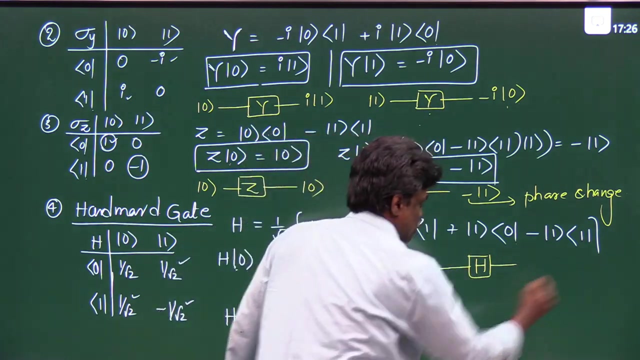 Hadamard gate is given the superposition. have you done the second one? so this is equal to 1 by root 2. I think you have see. you got this very nice, excellent. now please write this: gate operation: quantum gate notation. this is the quantum gate notation: input is 0, output right input is 1 and Hadamard gate is. 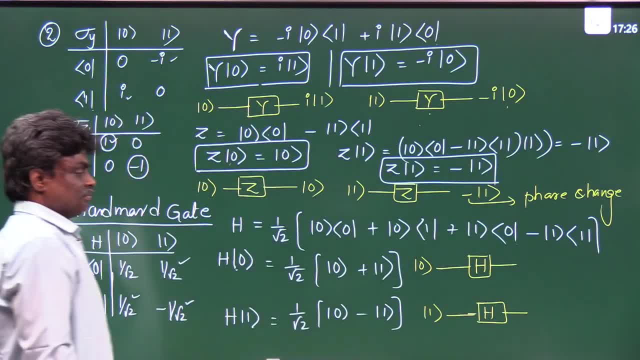 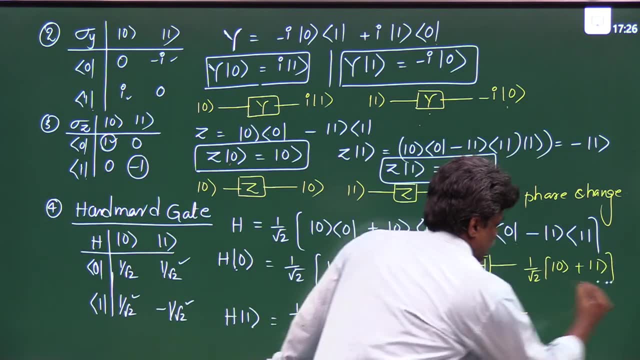 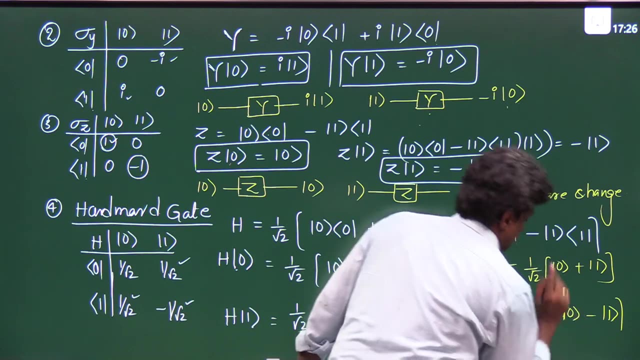 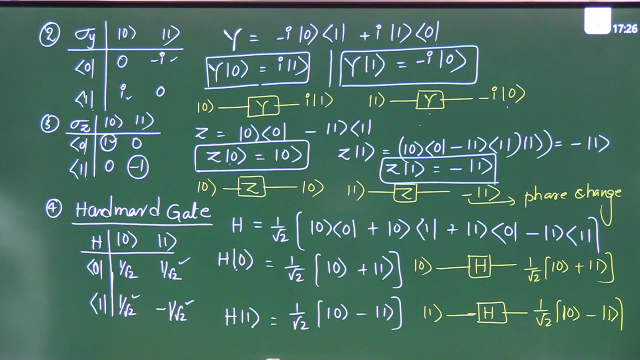 operated. what is the output? so this input is 1 by root, 2 plus 1 and this output: sorry output. if you copy, no use, because whatever I am explaining this algebra, you know as a quantum mechanics student, try yourself. then only there is some use and some interesting thing. 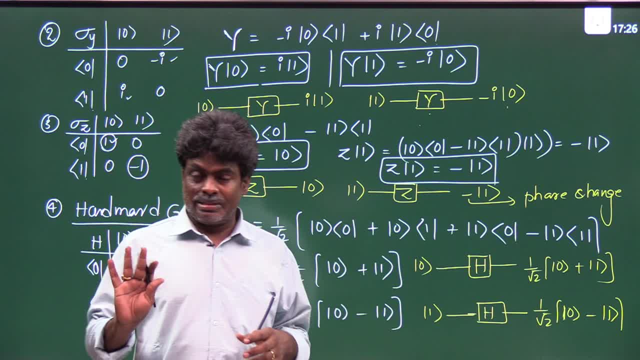 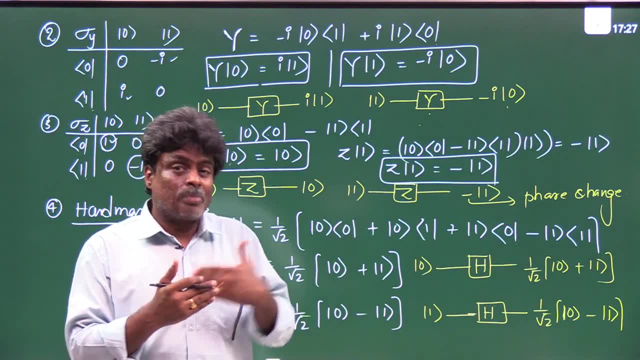 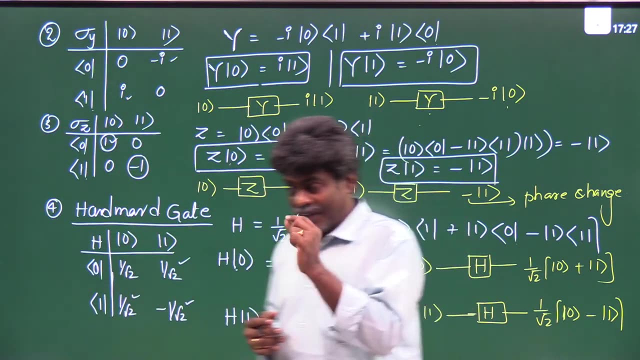 about this Hadamard gate, what Hadamard gate is doing here. that Hadamard gate is always creating the linear combination of that, our superposition state. I repeat, superposition state. okay, so there will be one more state called entangled, entangled state. that is also superposition state, but some difference. 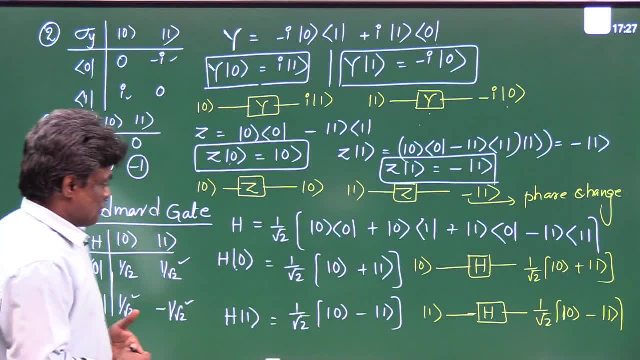 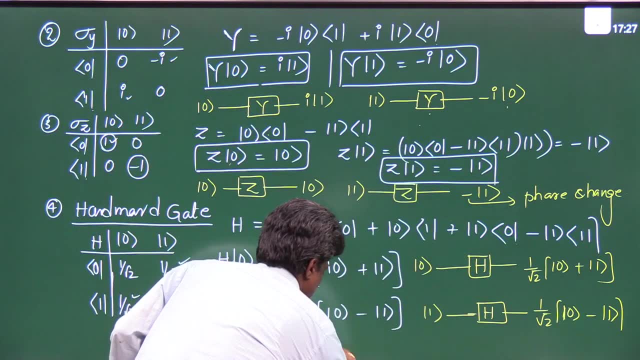 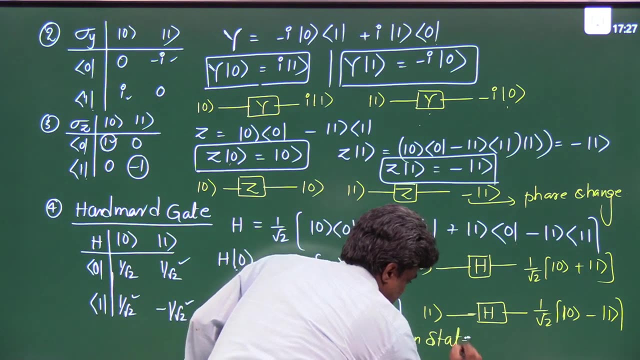 is there that we will discuss slowly. so this is also a superposition state. so Hadamard gate will give you the superposition state. superposition state ready. is it completed? are you understanding? if you are not understanding, it's okay. no need to, I won't mind, don't worry, because I don't know whether you are following or. 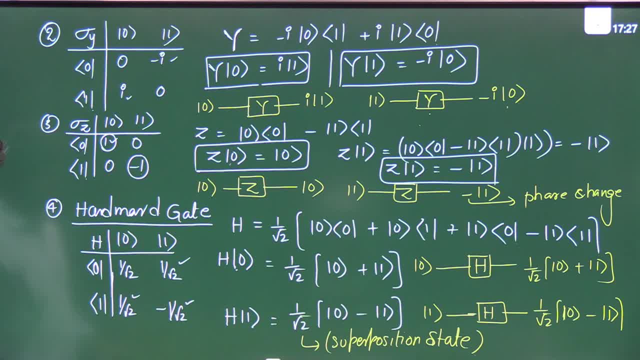 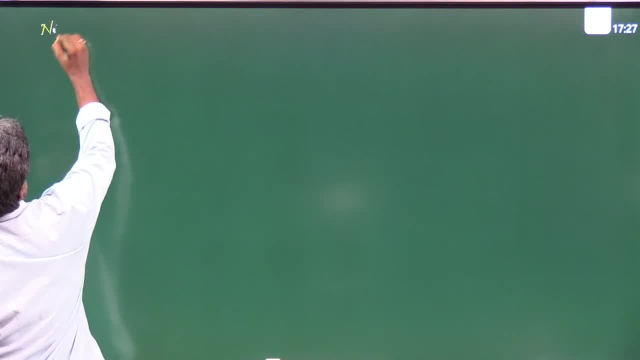 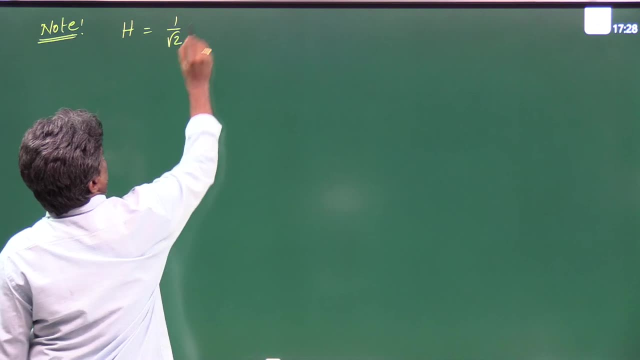 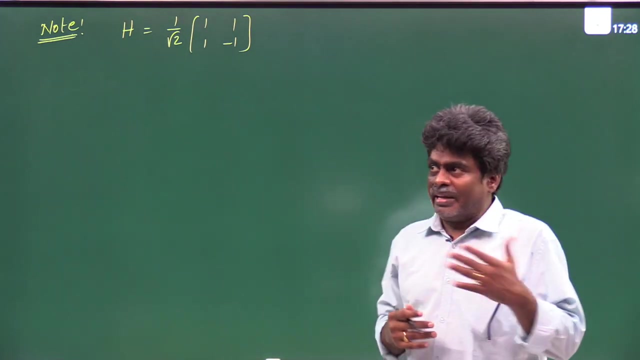 not ready, yeah, so here some more most important point here: everybody, listen, here we got Hadamard. gate H is equal to 1 by root, 2, 1, 1, 1 minus 1. listen, I don't know if you are reading any textbook. I think only one very standard book is. 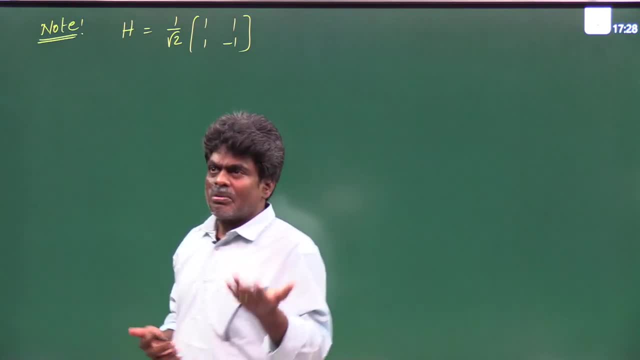 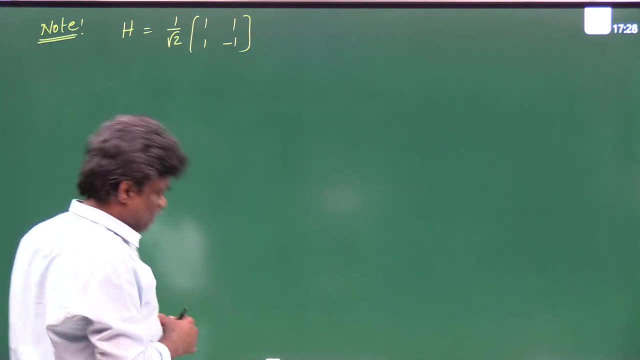 there. I think maybe you are reading that book only. maybe some of you have done some projects during your MSC. okay, so about this Hadamard gate? what they have given this Hadamard gate is a square root of, not gate, I don't know how many. 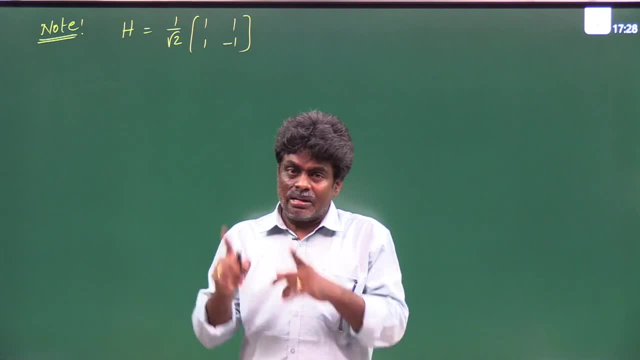 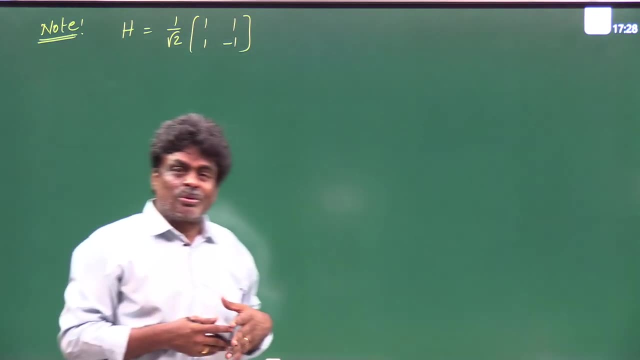 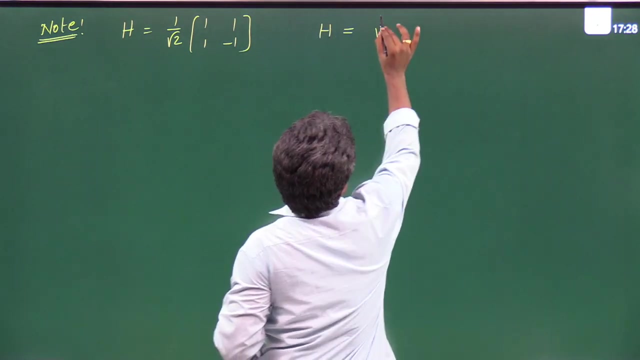 of you heard this word. Hadamard gate is nothing but the root of not gate. that means a square root of not gate. why? why it is called square root of not gate. let us discuss. are you ready? yeah, so this Hadamard gate is also called as a. 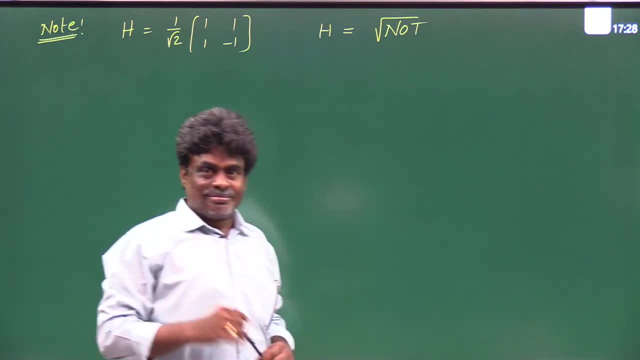 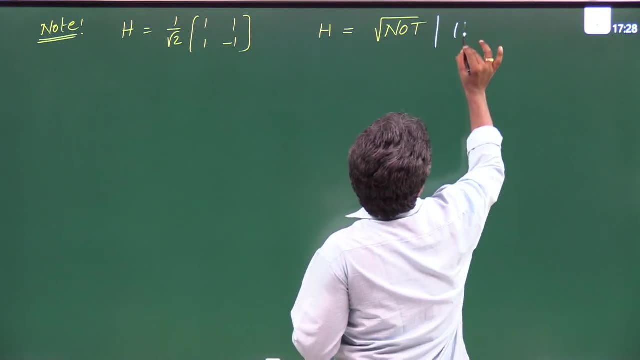 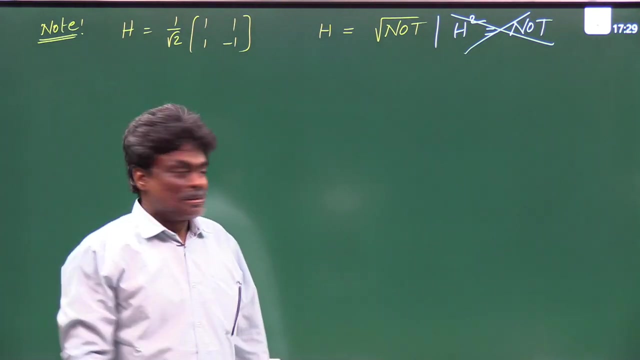 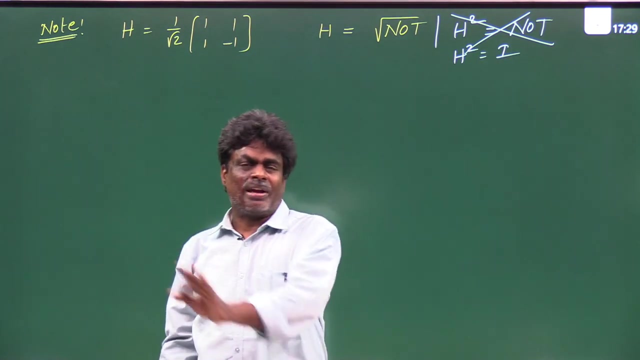 square root of, not gate. and it is called square root of not gate. and don't be confused here, sir. if I apply square on both sides, that means H square, will I get not gate? absolutely wrong, because you know already, H square is equal to identity. it simply it is called as a square root of, not gate. why it is. 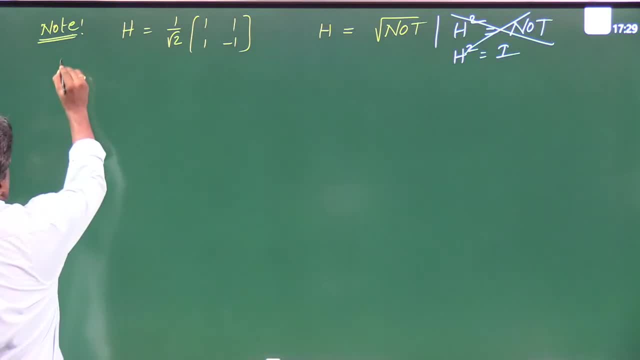 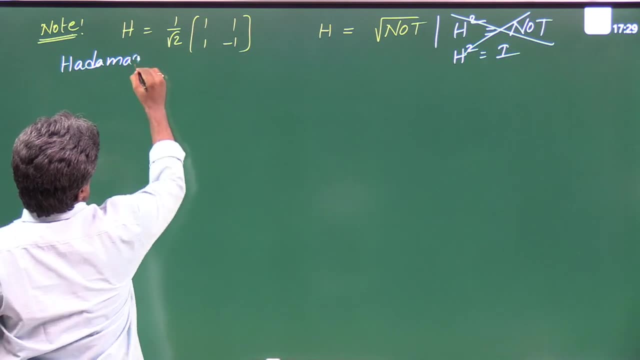 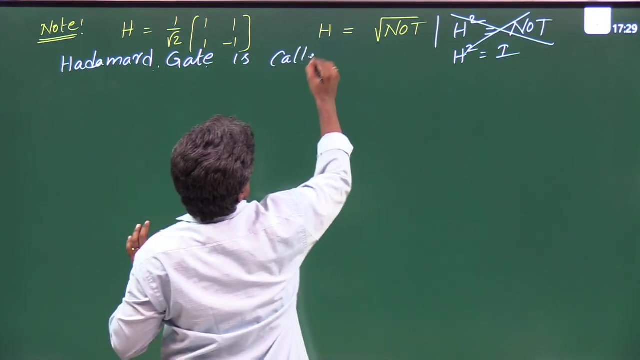 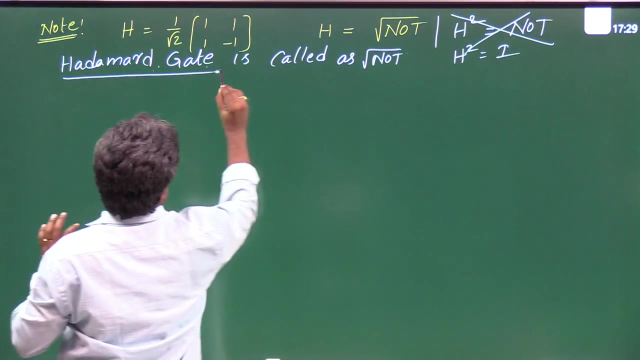 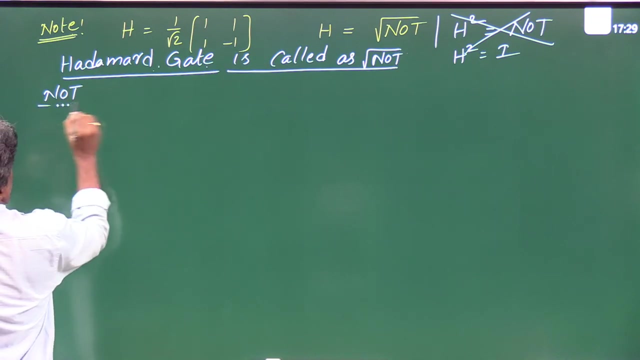 called a square root of not gate. ready? so Hadamard gate, I think. okay, Hadamard gate is called as square root of not gate. why so, listen? so first of all, let us take one more time the not gate. what the not gate is doing already you know. 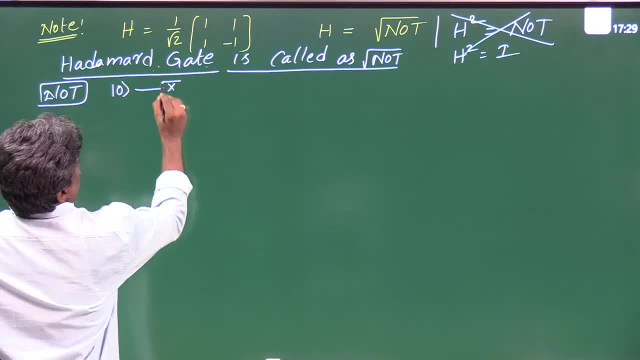 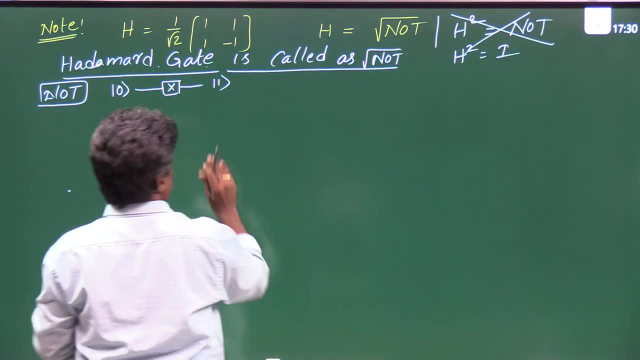 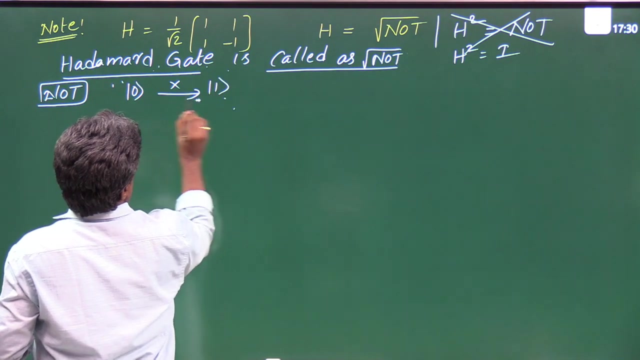 it flip this 0 to 1 and as well as 1 to 0. that is vice versa, am i right? i will write like this: 0, this x gate 1 and this 1 to 0, so this is a flipping between 0 and 1.. 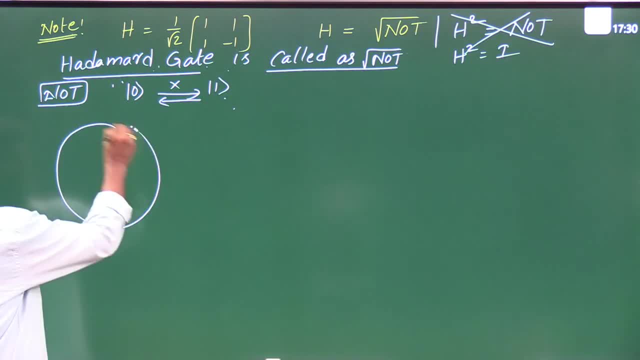 now i would like to take this block sphere. i told you this is a very important role. it will play very important role. okay, so i'm taking this. everybody listen. so this is my initial state. so that is a ket: 0- north pole and if you apply x, gate what it is. 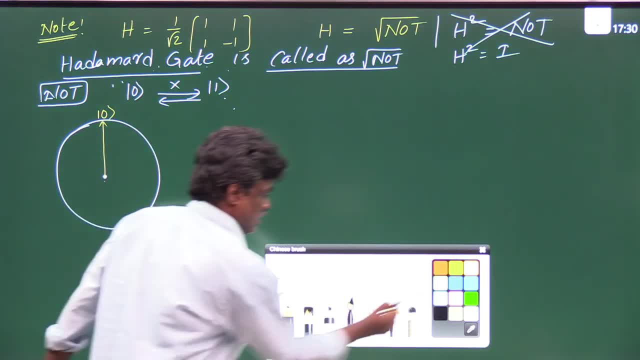 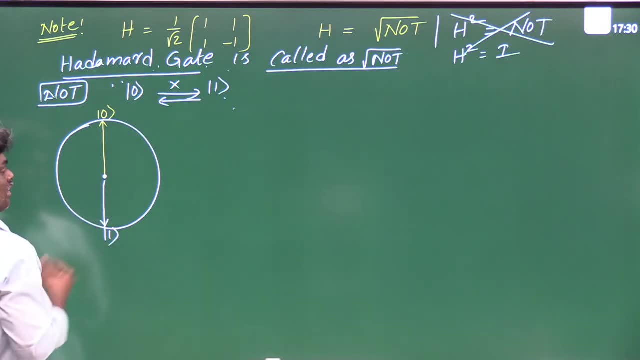 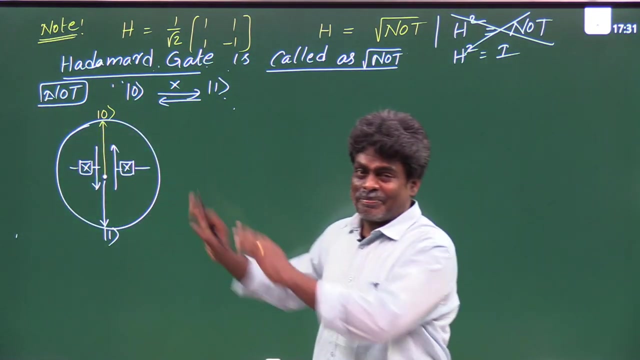 doing. it is, it is converting or it is becoming this one state and vice versa. this is zero become one, okay. similarly, one become zero. so i will write like this: i think now you understand this is the x gate operation. that's good. so i represented like this. now, if you see carefully, what is this? 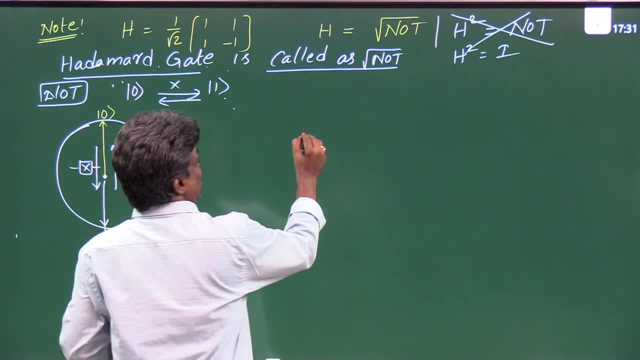 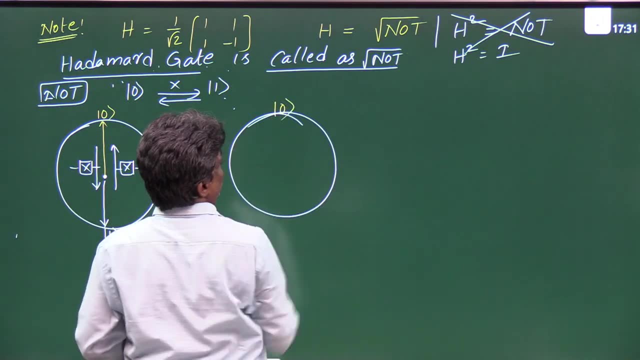 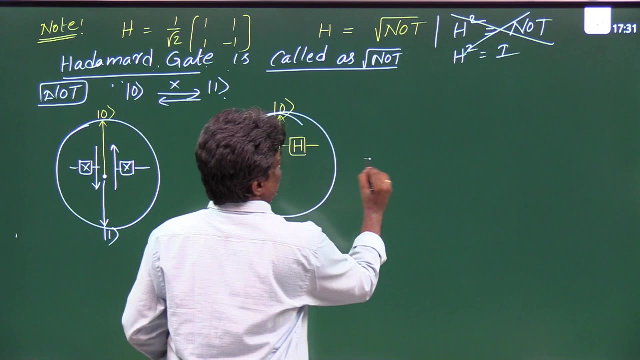 Hadamard gate is doing ready. so here we have, this is the block sphere, and initial state is zero. now, this is your initial state. now you apply the Hadamard gate here. so what it is doing, you know this is the again block sphere. okay, so see carefully. 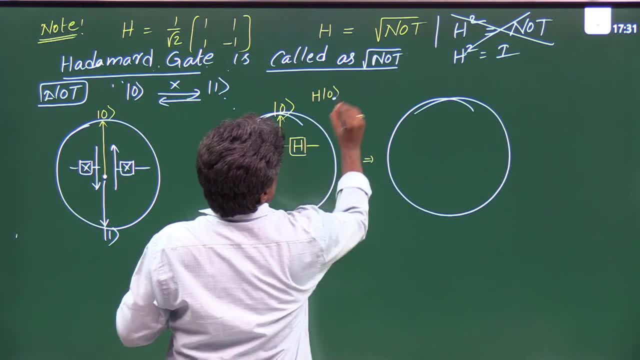 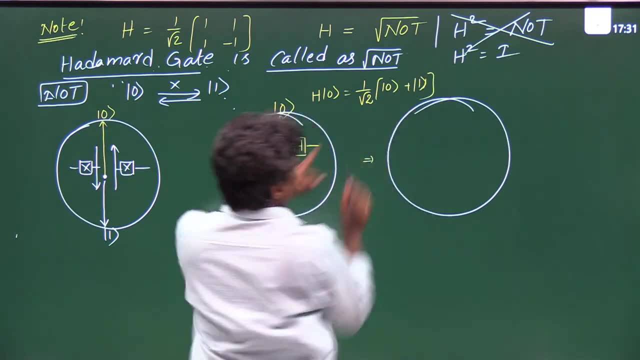 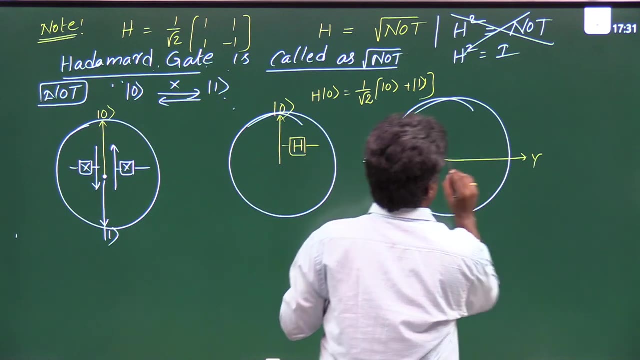 whenever Hadamard gate operates on zero. i think you know the result: it is a linear combination of zero and one. what is the meaning of this? what is this state represent? this state represent now: this is the y-axis and this is the z-axis, and this is: 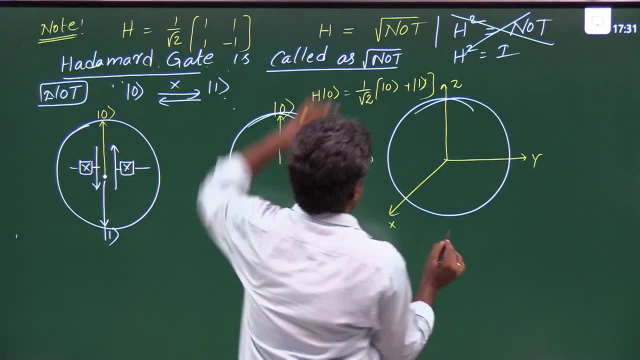 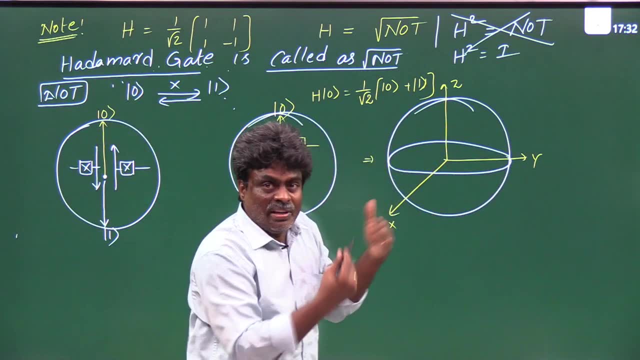 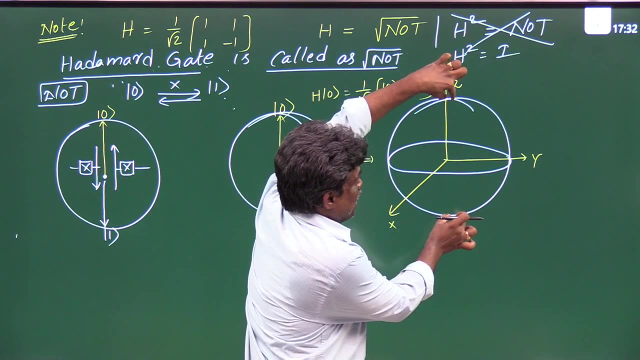 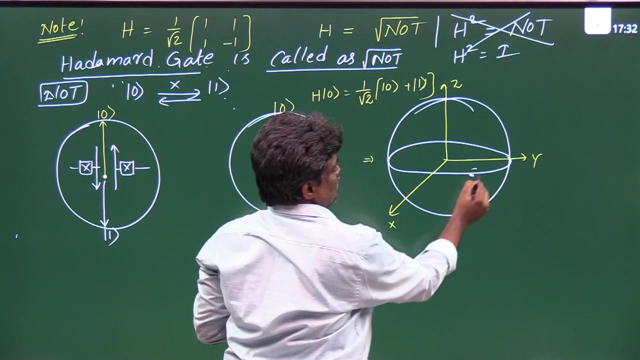 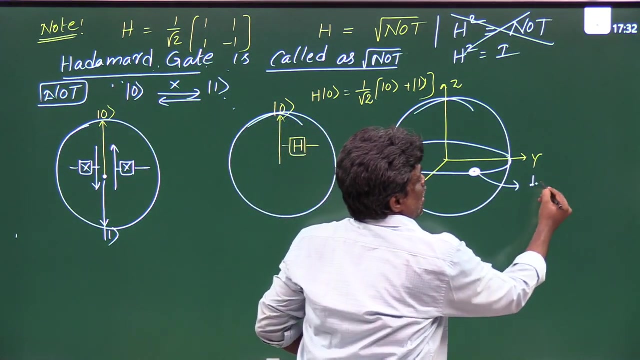 x-axis. actually, this is nothing but a state which is halfway between, halfway between this: 0and 1, i repeat, this is the zero and this is the one, and this state is halfway between zero and one, somewhere here, let us suppose. so this is the plane. okay, here, somewhere in this plane. so this is 1 by root, 2 ket 0 plus ket 1. 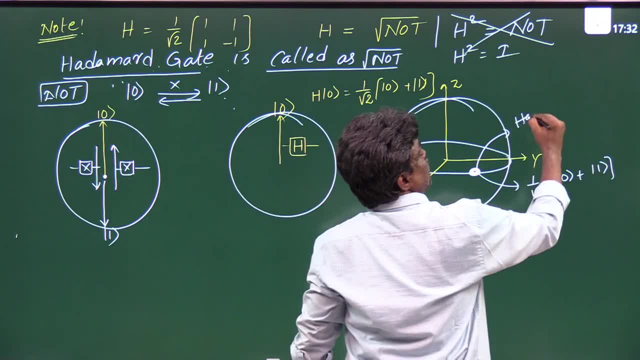 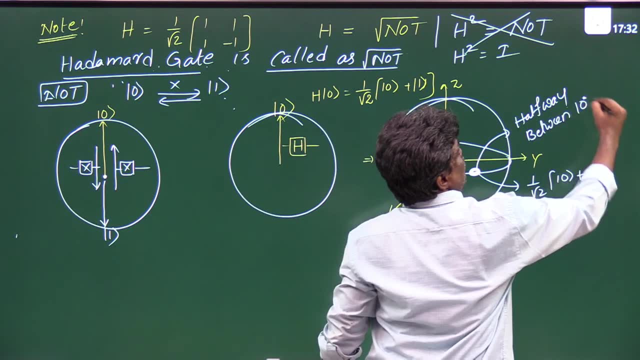 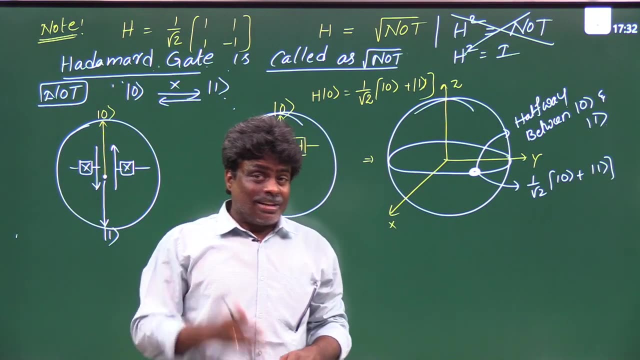 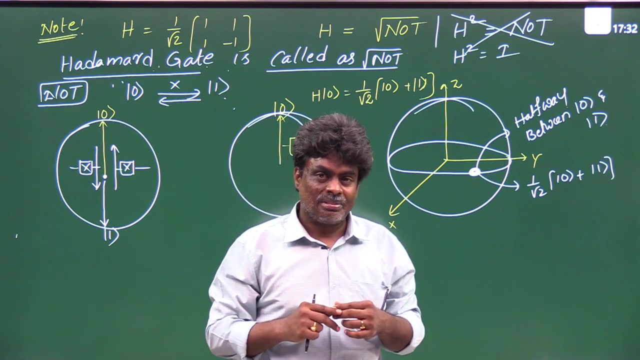 so this point is nothing, but simply it's somewhere halfway or midway between between 0 and 1. that's why it is called square root of naught. the naught gate is completely, completely transforming north pole to south pole, south pole to north pole, but the Hadamard gate is doing what it is doing, that zero state is. 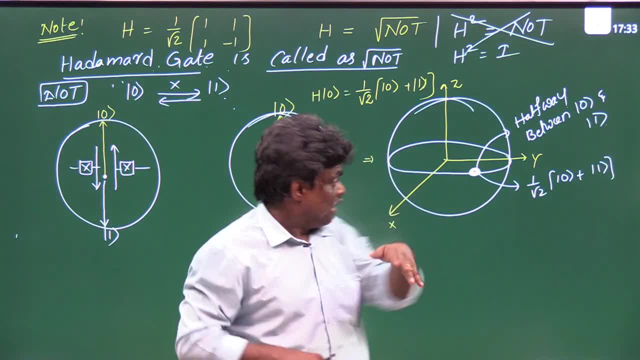 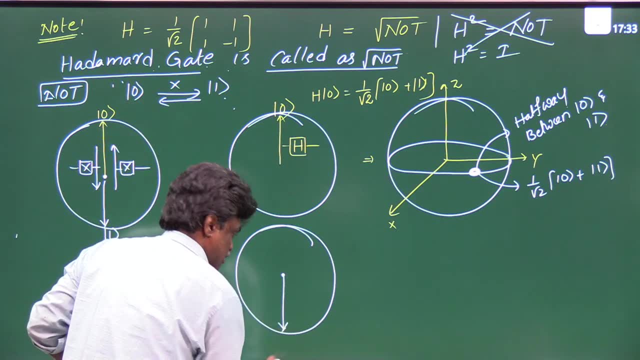 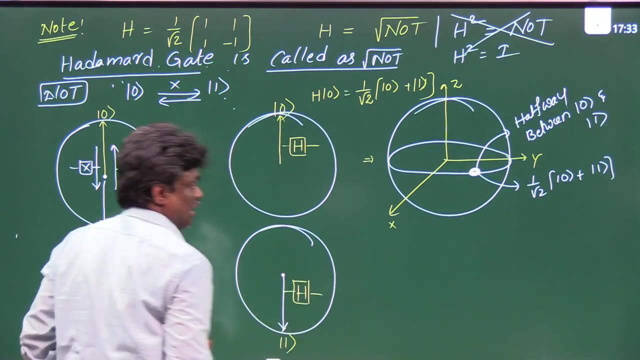 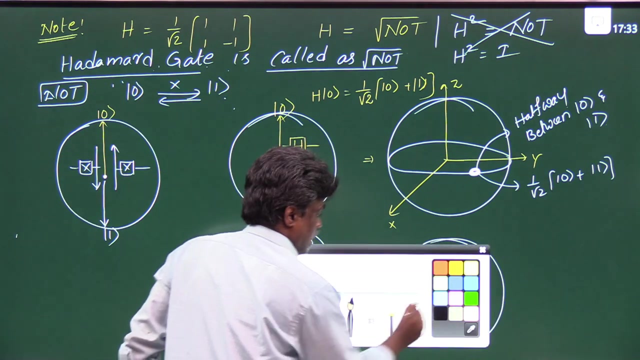 converted to halfway between 0 and 1 and similarly 1. also, if you take this, this is the initial state, so i'm taking this is a 1. now i applied the Hadamard gate on this, okay. so then again, i'm taking this block sphere, okay. so i hope you are understanding. 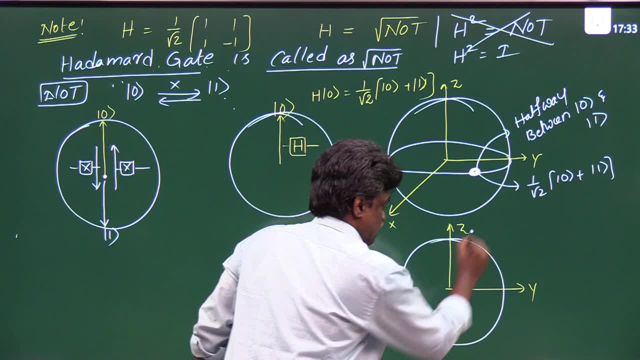 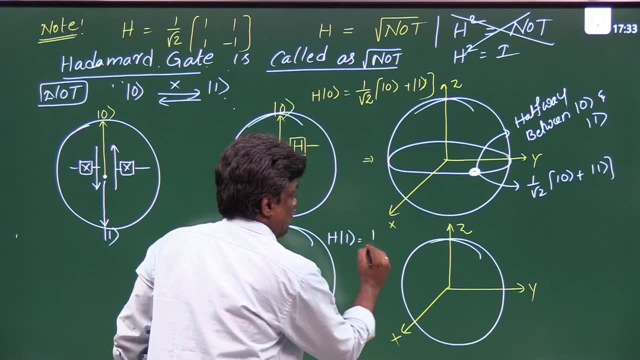 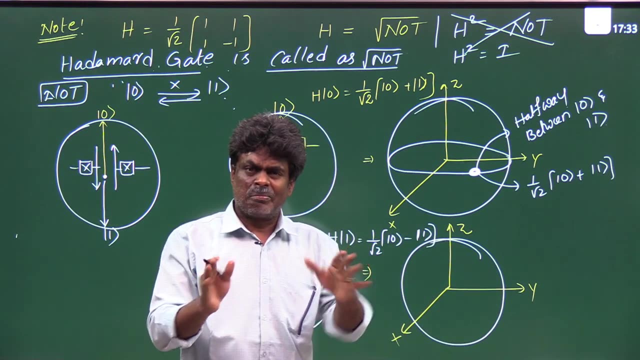 this is a y and this is a z and this is x. so earlier what i said- here you got h- operates on 1, 1 by root, 2, 0 minus 1. this is also somewhere halfway between that 0 and 1. if you take this block sphere. again, i'm taking this block sphere. okay, so then again, i'm taking this block. 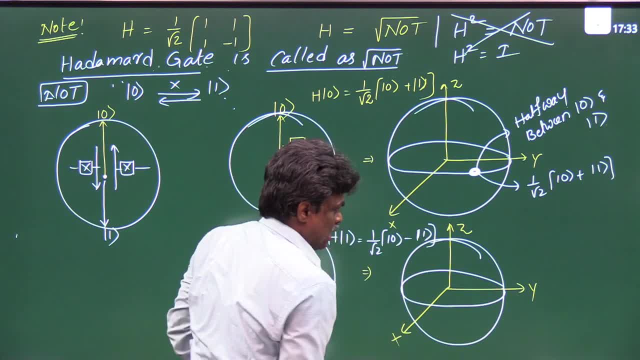 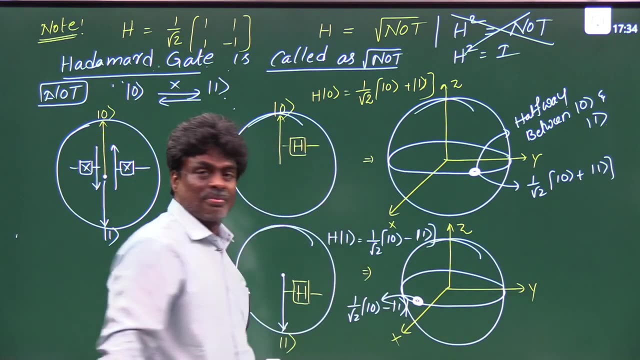 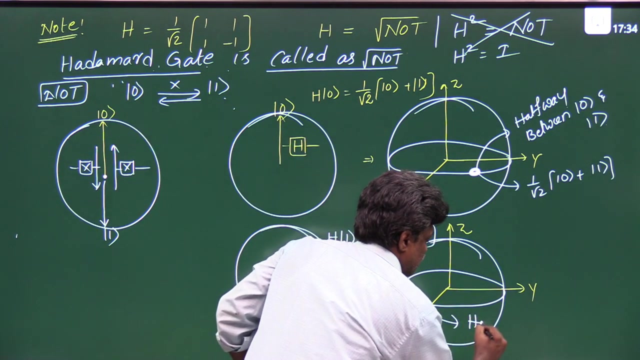 you take this plane, which is in between 0 and 1, somewhere here, let us suppose somewhere here or here, whatever it may be somewhere here. so this is 1 by root, 2, 0. if you want exactly, you can identify. it's not an issue, that's it. so this is also somewhere halfway between. this is a halfway. 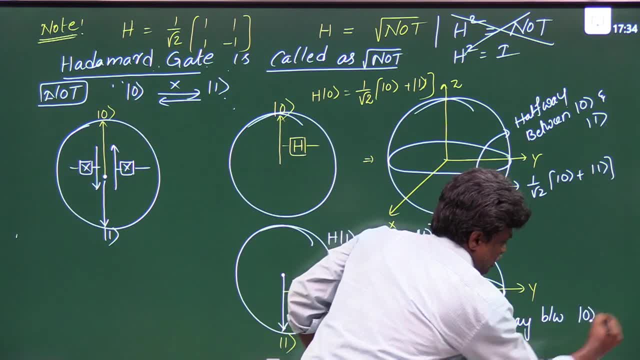 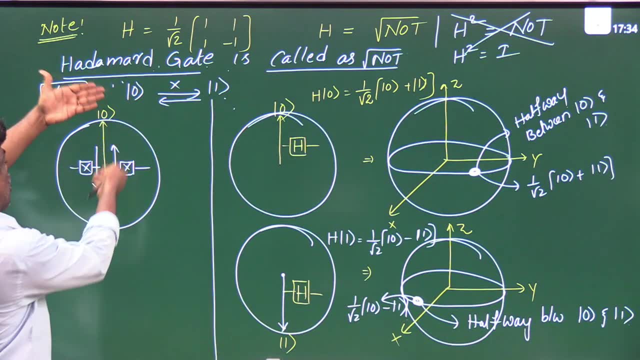 between ket 0 and 1. so this is a half way between ket 0 and 1. so this is a half way between ket 0 and 1 and a ket 1, so the north gate is completely transforming north pole to south pole, south. 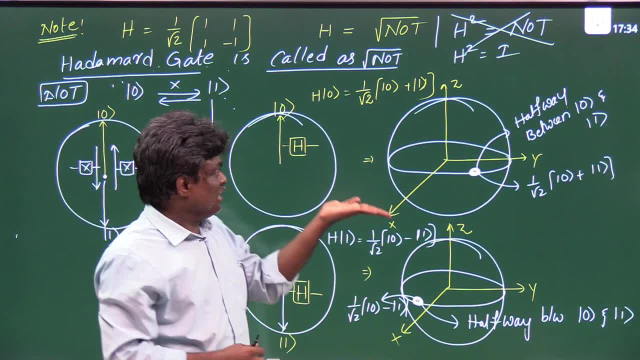 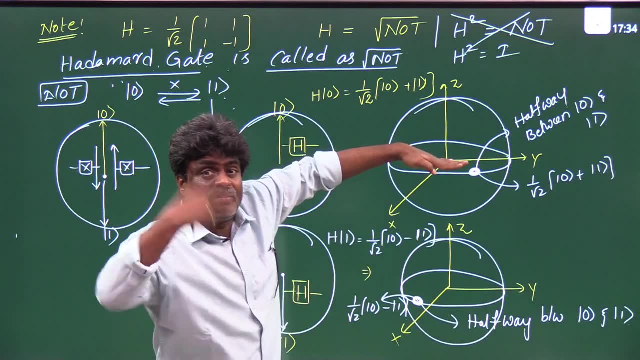 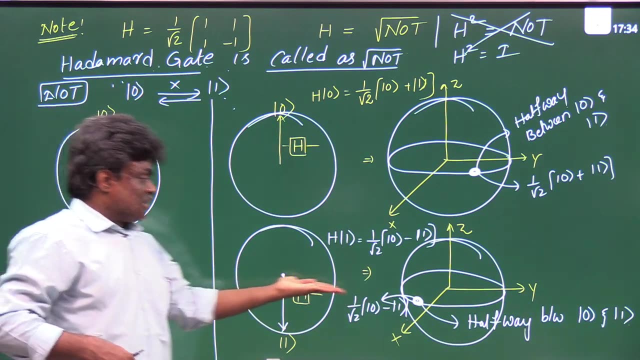 pole to north pole but the Hadamard gate. what it is doing it is taking a 0 state and converting a state in between, exactly midway between 0 and 1. similarly, it is taking one state and it is converting to some other state which is in between, halfway between that 0 and 1. 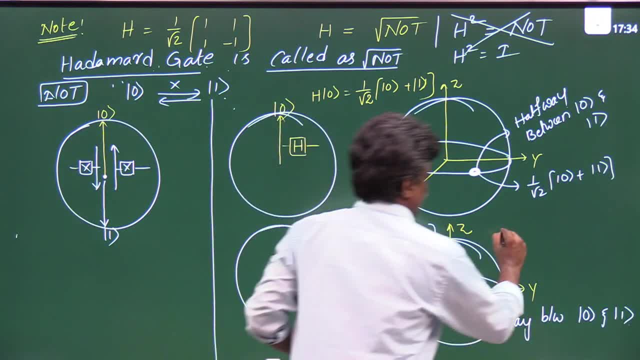 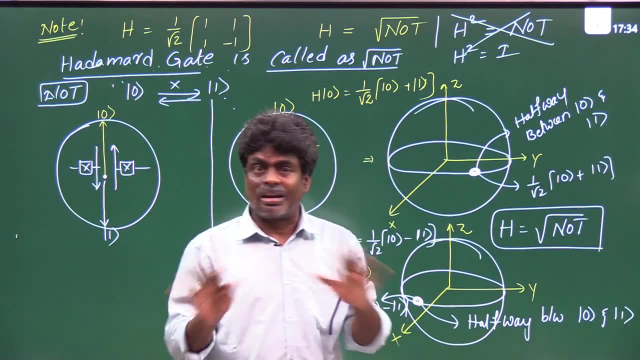 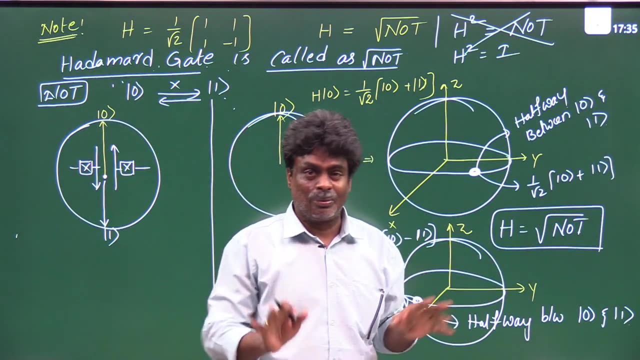 that's why this Hadamard gate is called the square root of north gate. this is the reason and don't ever try to get. take the north gate and apply square root. will you get the Hadamard gate? no, why they call it as a square root of north gate based on this operation. so here it is. 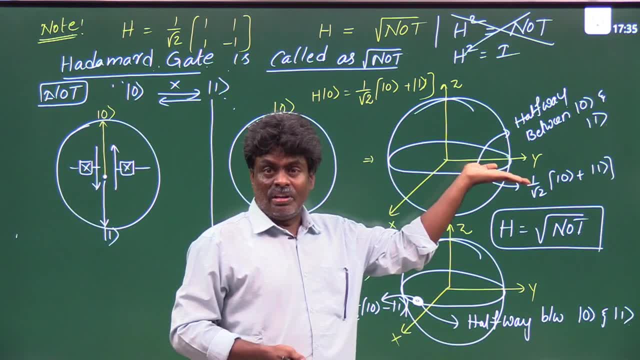 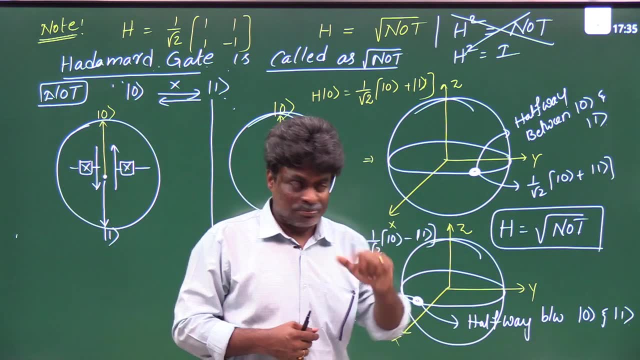 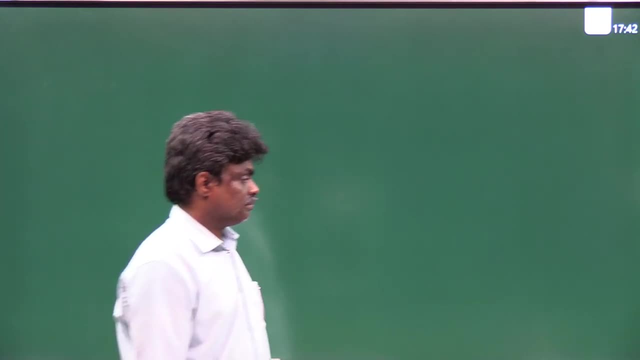 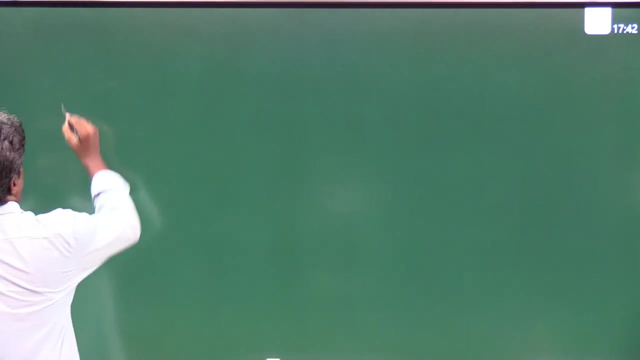 completely transforming here. somewhere midway between it is transforming, so that's why the- this is also called as square root of, not gate. Got it Right Now? listen Here. we understand. what is this? Hadamard gate operation. Okay, once again. 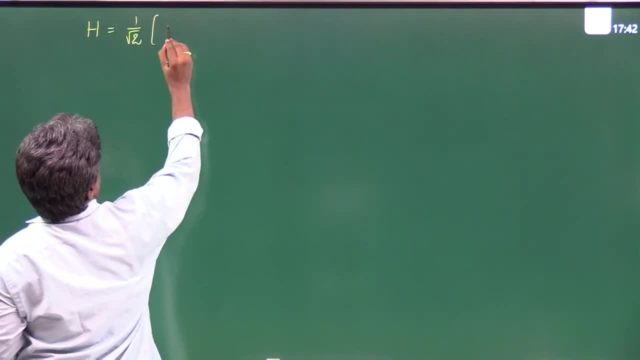 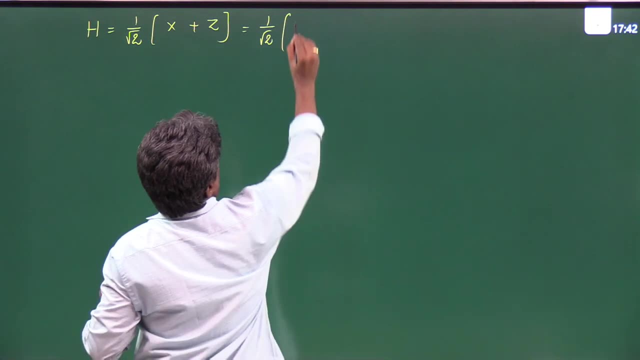 Hadamard gate is a simply combination of two gates. One is a poly x, another is a poly z, So which is nothing but 1 by root, 2, 1, 1, 1, minus 1.. That's good. And what is this operation? 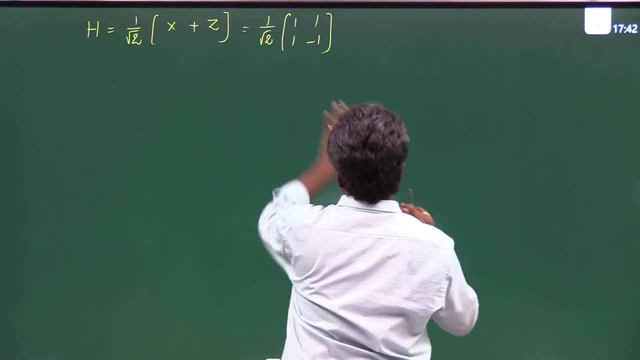 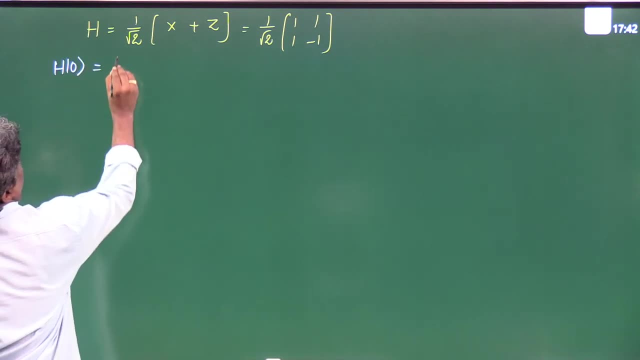 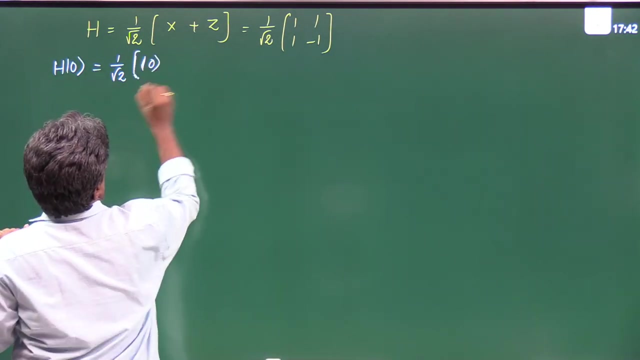 H operates on 0.. Listen carefully, Okay, I will write here. So Hadamard gate operates on 0.. What you are getting: 1 by root, 2, ket 0.. Ket 0 plus ket 1.. I hope you got it. 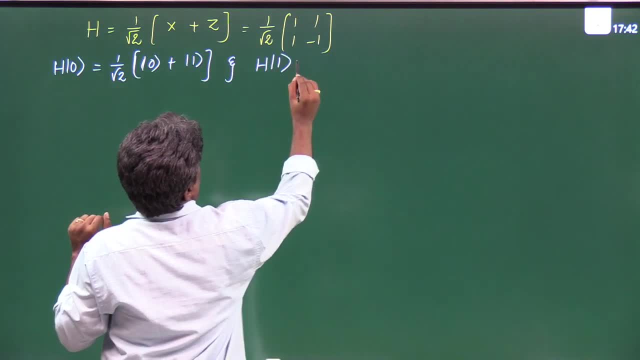 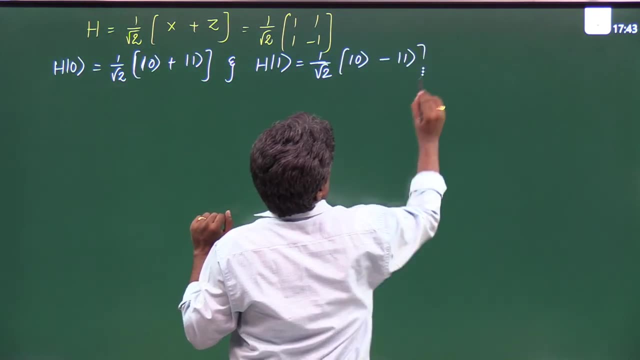 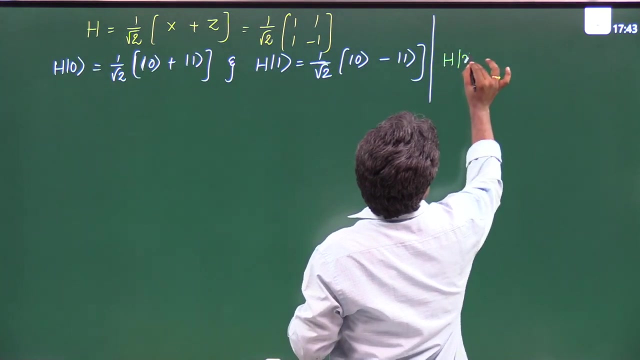 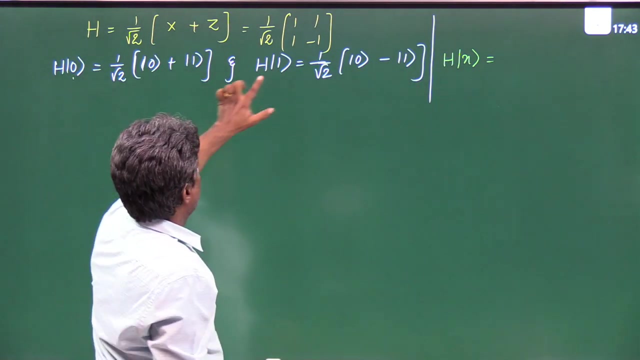 And Hadamard gate operates on 1.. We got 1 by root, 2. A superposition state. we got 0 minus 1.. Now, more generally, we can express this as the Hadamard gate operates on x. The Hadamard gate operates on x. See whether it is operating on 0 or whether it is operating on 1,. 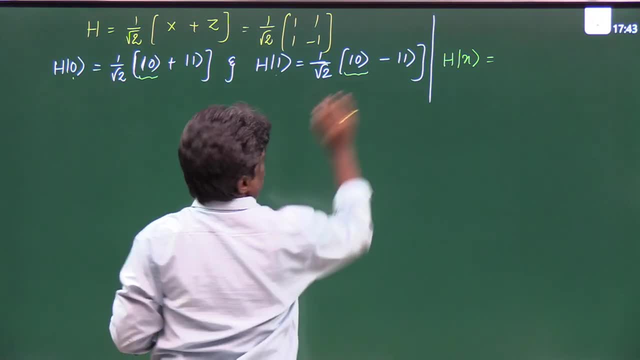 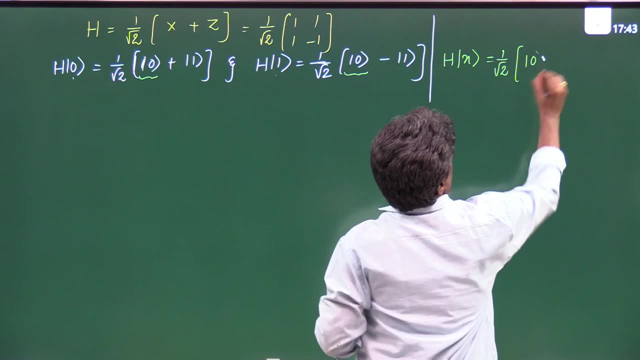 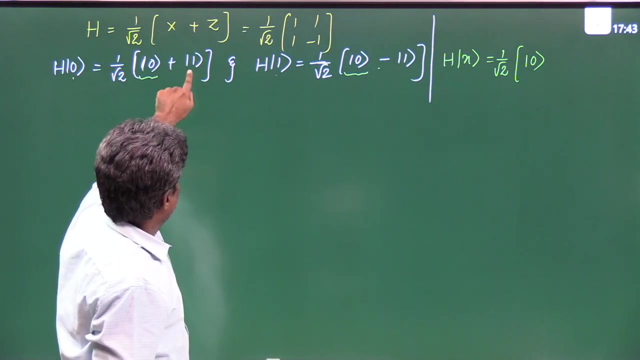 there is no change in the first. There is no change in the first one. That's why 1 by root, 2, ket: 0 as it is. If it is 1, here you are getting minus. If it is 1, here you are getting minus. 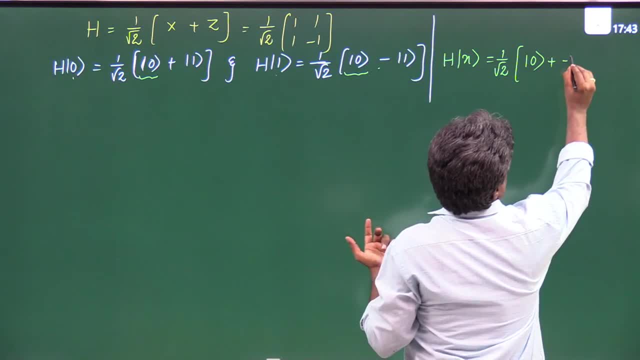 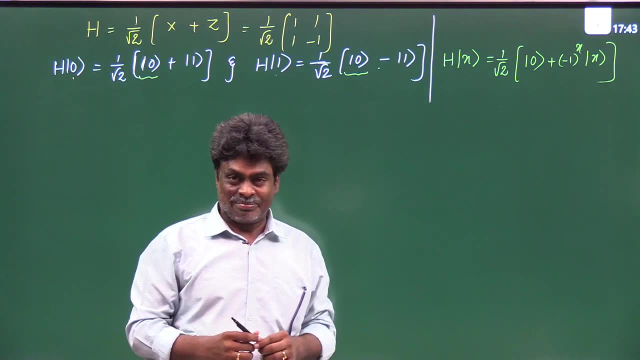 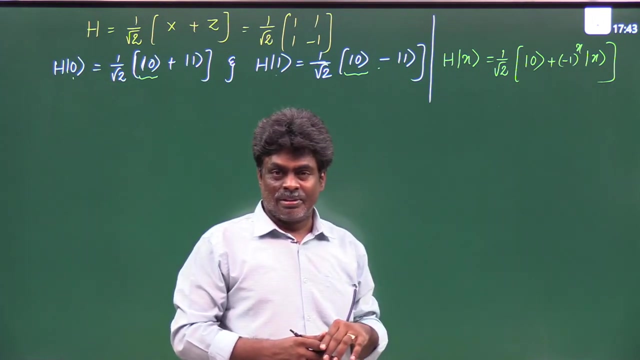 That's why I will write more generally: Plus minus 1 whole power x into ket x. This is just a general representation, A single representation. No need to write two times like this. Let us write like this, Okay. So now the point is: this is very crucial, very interesting. 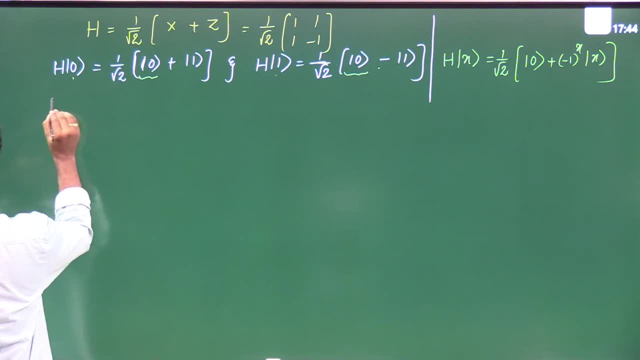 Listen Now I am operating Hadamard gates like this. Take a small task Now. I have taken Again here. input is 0.. I am operating Hadamard gate- Okay, Something I will get. And again I have taken one more input And the second Hadamard gate I have taken. 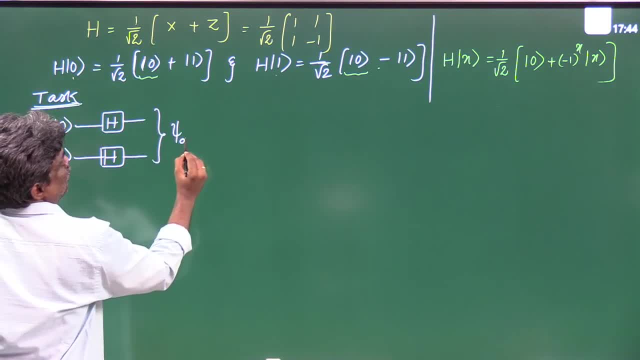 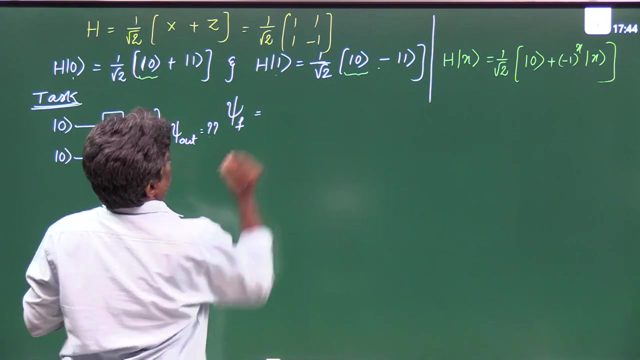 Now, what will be the output? What will be the output Ready? So today, just listen, I will explain why we are writing like this. Maybe tomorrow I will explain. So the psi final are output, Output. whatever it may be, Psi final is equal to Ready. It's very simple. This Hadamard gate is operating on 0.. 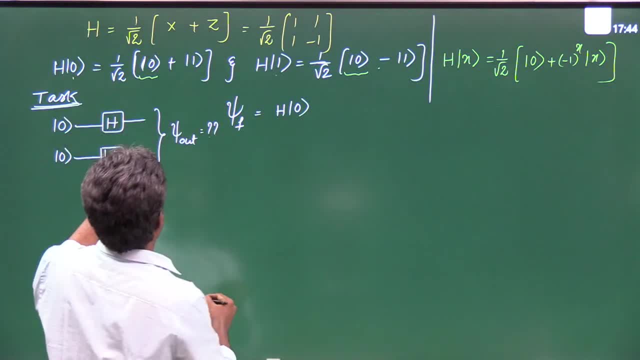 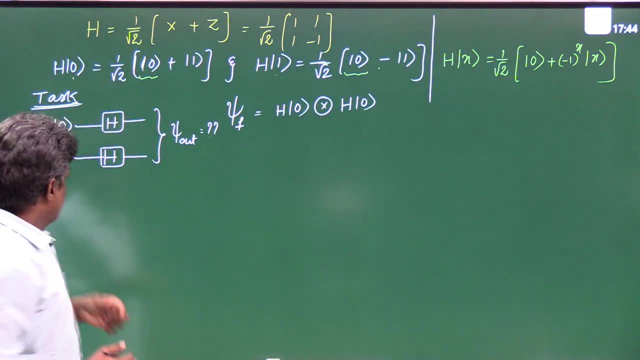 That's why Hadamard operates on 0. And this Hadamard operates on 0. And we have to take the tensor product. That's it. So if I have 3, you will get one more tensor product. So if I have 4, you will get one more tensor product. 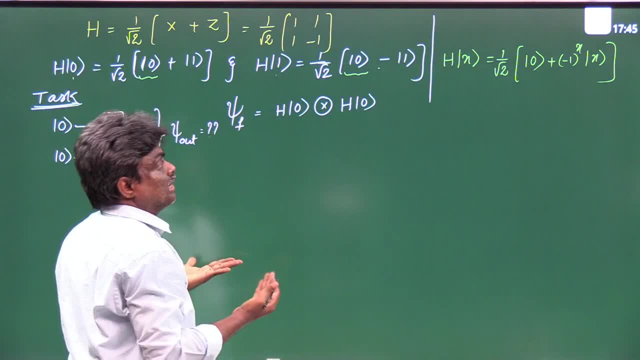 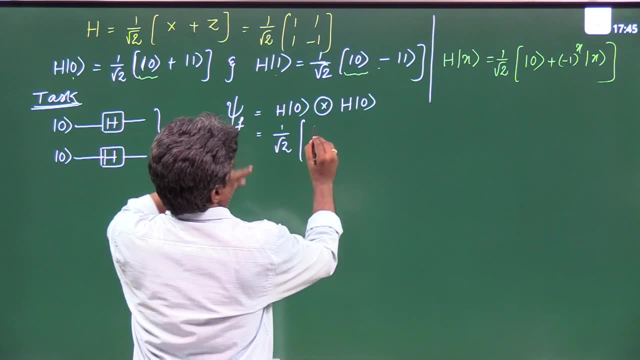 Let us do for two things, Because if you take many, you will get confusion. Let us do this. I hope you know 1 by root. 2. Already, you know this. Shall I write this as What is this One minute? 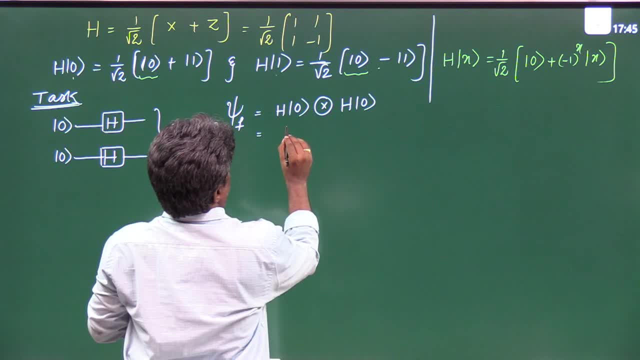 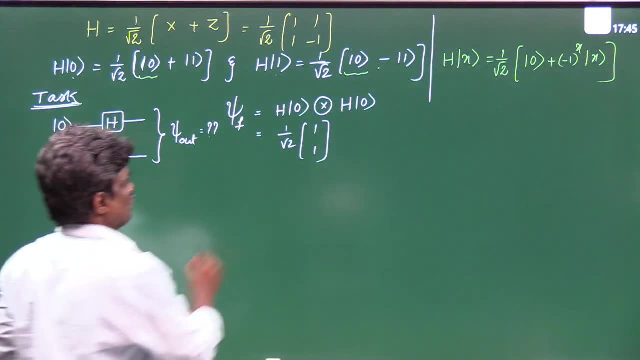 Yeah, So Hadamard gate operates on 0.. What you will get: 1 by root, 2. I think 1, 1.. Am I right? Please check? Yeah, That's it, Because this can be written as what. 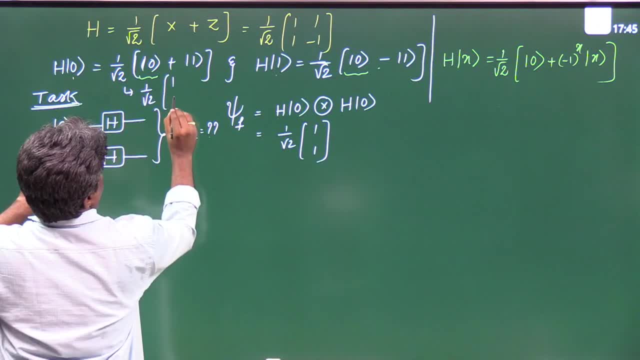 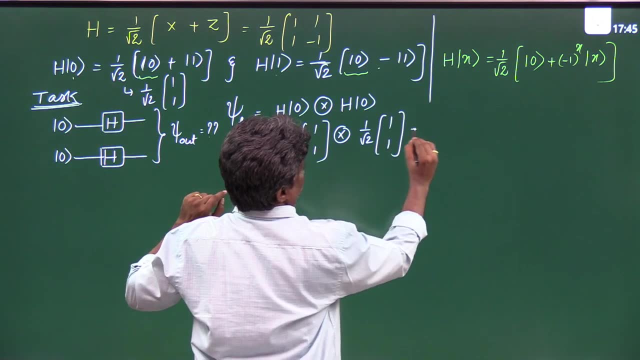 This can be written as 1 by root, 2. In the matrix form: 1, 1.. So tensor product: 1 by root, 2. This is also 1, 1.. Carefully observe Please. Very important, Very important. 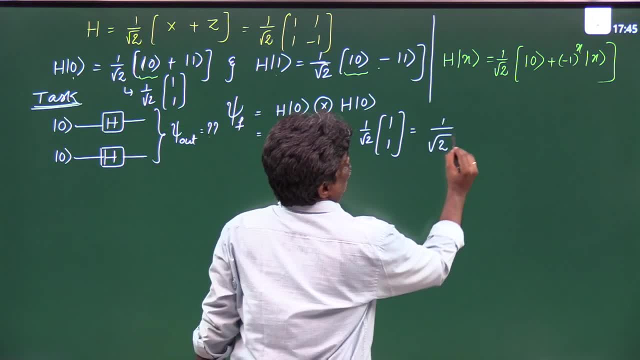 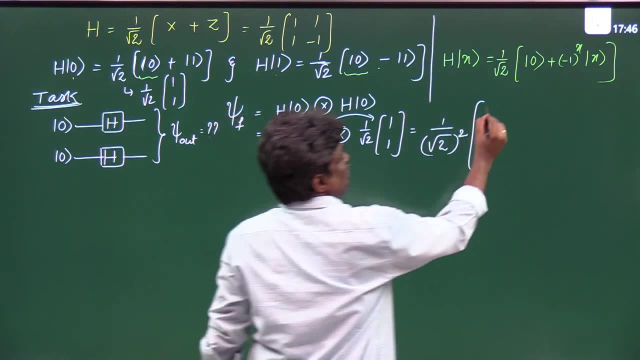 So tensor product, No need to get tension Or root 2 whole square. Take this 1 and multiply with the entire matrix, That is 1, 1.. Take this 1 and multiply with the entire matrix: 1, 1.. 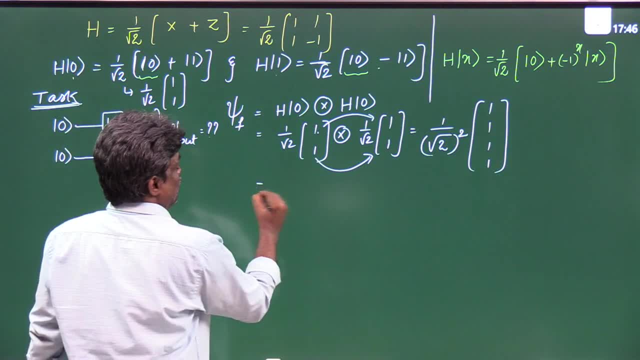 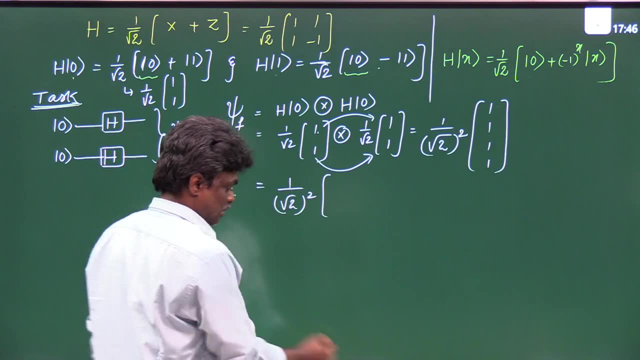 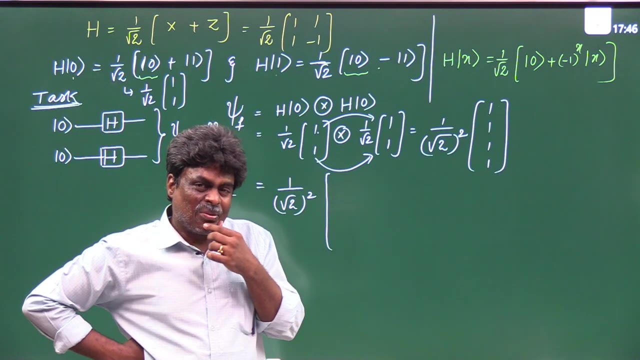 See the beauty. Now, here we got the final state: 1 by root, 2 whole square Into Everybody. please, Please, listen carefully. Here I have 1, 1, 1, 1 like this: What is this? 1, 1, 1?? 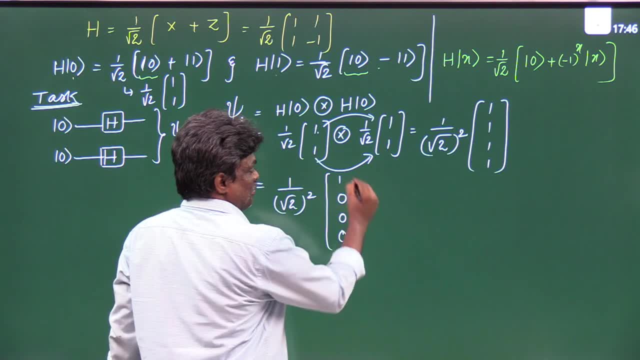 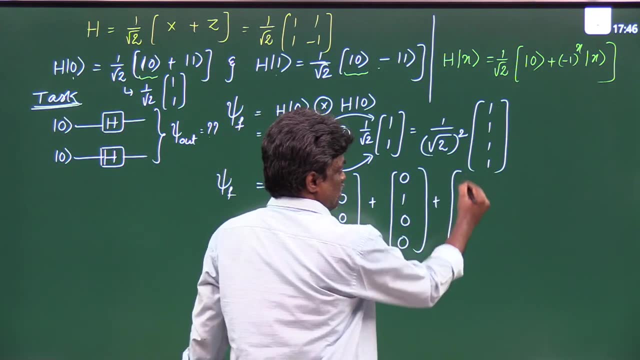 If you observe carefully, I can write this: 1, 0, 0.. Plus I can write this as 0, 1, 0, 0.. Plus 0, 0, 1, 0.. 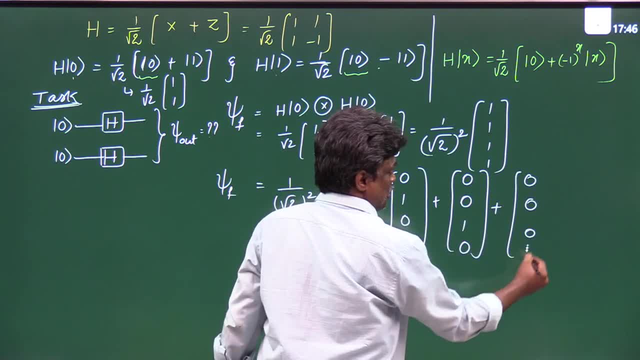 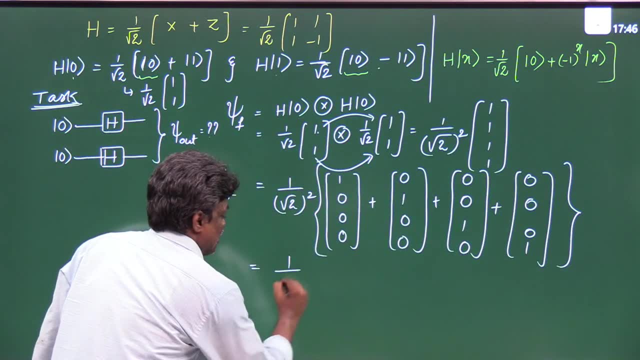 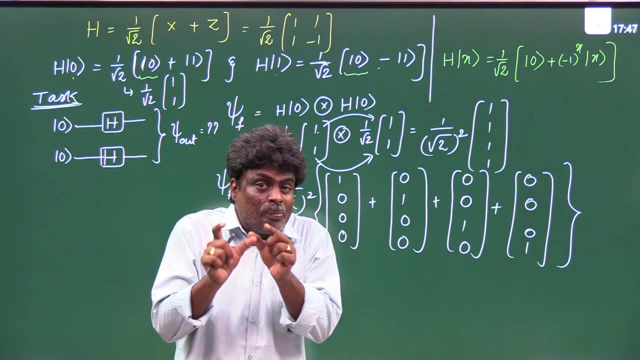 Plus 0, 0, 0, 1.. Wait a minute. So here we can write it as 1 by root, 2 whole square. Can you please tell me? I already explained this. 2 qubit states. 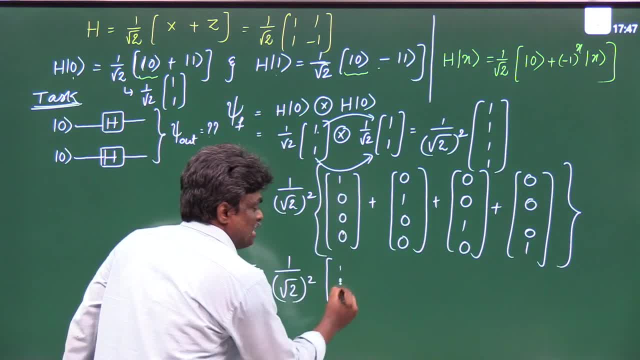 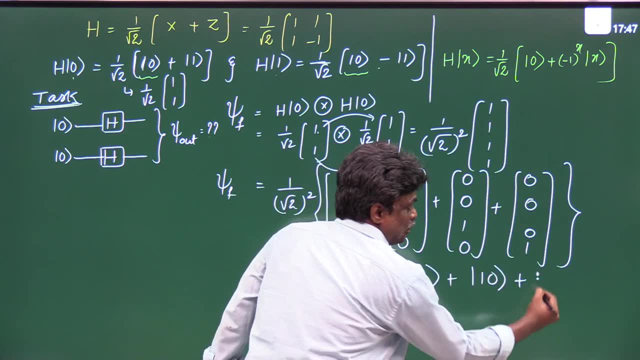 2 qubit base states This: first one is 0, 0.. Second one is 0, 1.. Third one is 1, 0. And fourth one is 0, 1.. I hope you got it. 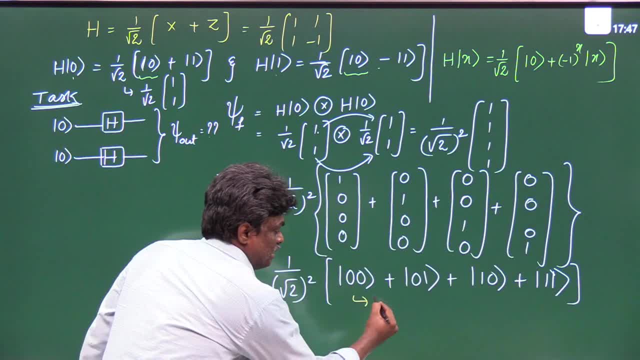 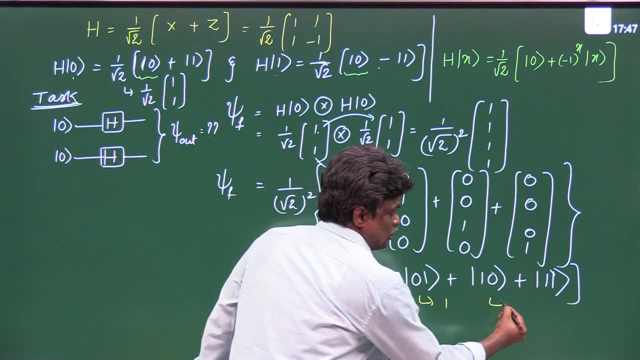 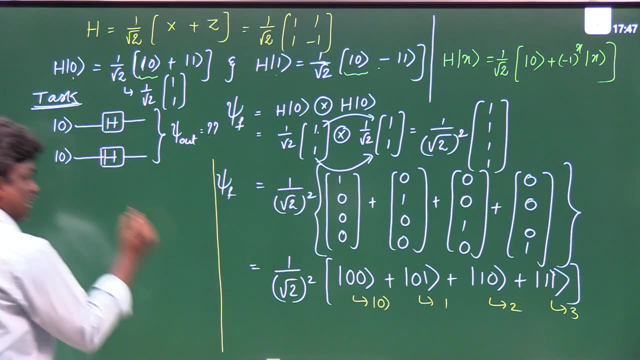 And once again, Let me write the binary notation 0.. Okay, But I have written ket, And here this is a 1. And this is a 2. And this is a 3.. So, Finally, Whenever you have this, 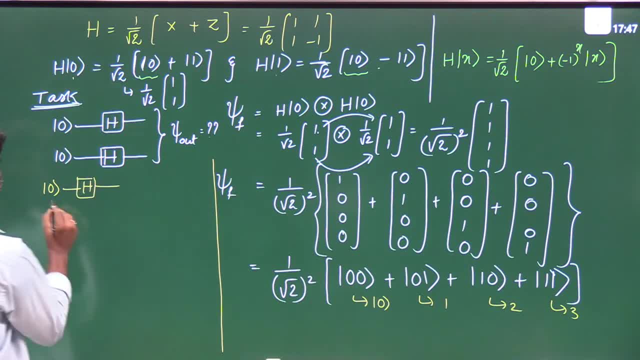 You operate the Hadamard gate on a 2. 2, 0 states. 2, 0.. 2, 0 states. Carefully, observe What is the final output. We got 1 by root, 2 whole square. 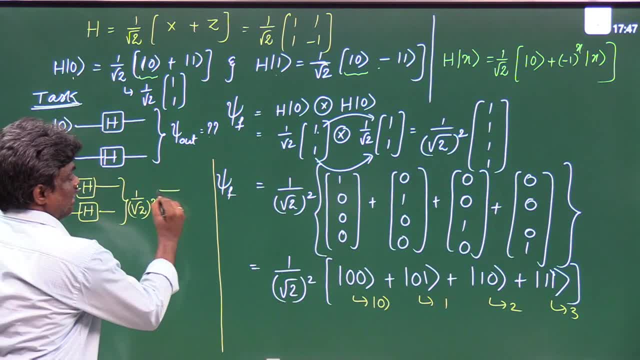 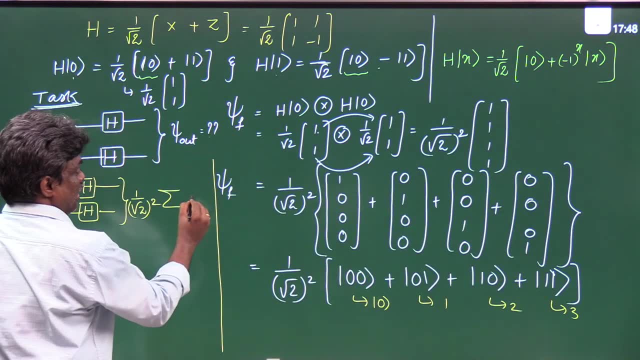 Are you observing? 1 by root, 2, whole square Linear combination of 0, 1, 2, 3.. Repeat 0, 1, 2, 3.. That's why I'm taking some j. 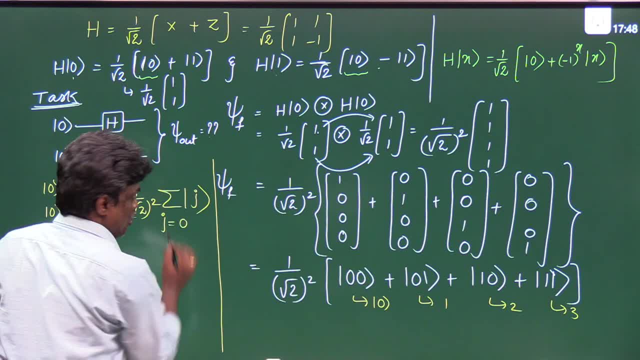 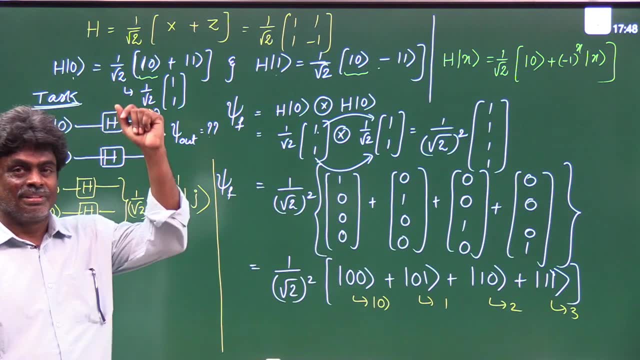 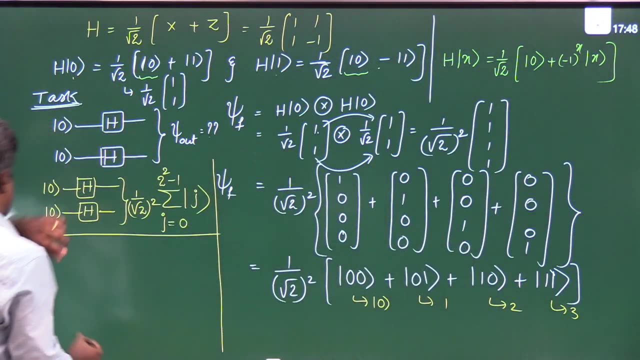 That j value takes from where 0,, 2, 3.. That's why I can write it as a 2 square minus 1.. What is this? Wait a minute. Let me write more generally. So If I take 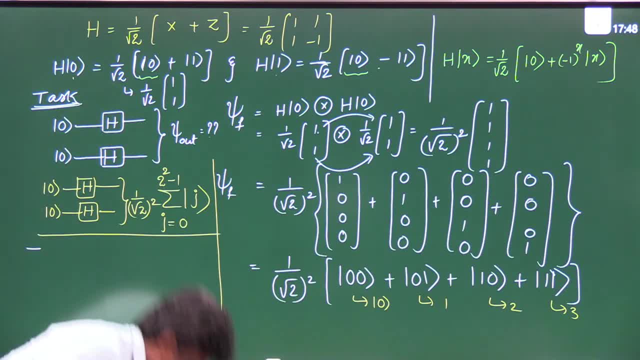 Like this, That is. That is, I have taken 0.. Hadamard And again 0. So n inputs I am taking, So like this, n times operated, Then what will be the output according to this? 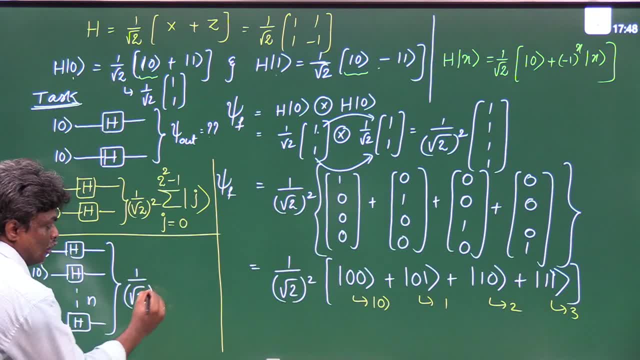 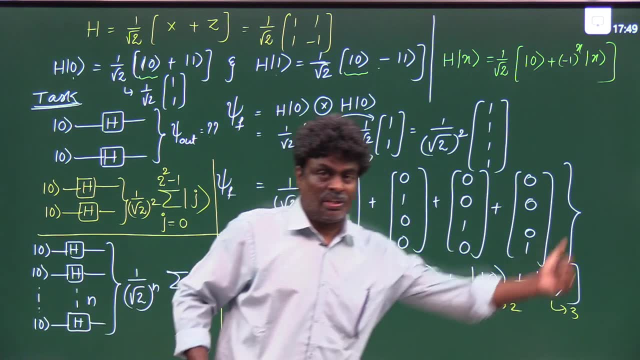 Could you please tell me 1 by root, 2, whole power n Sigma j That j stands for: 0,, 1,, 2,, 3,, 4,, 5,, 6,, 7,, 8.. 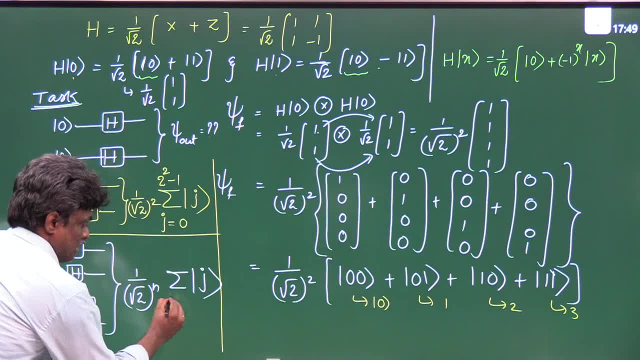 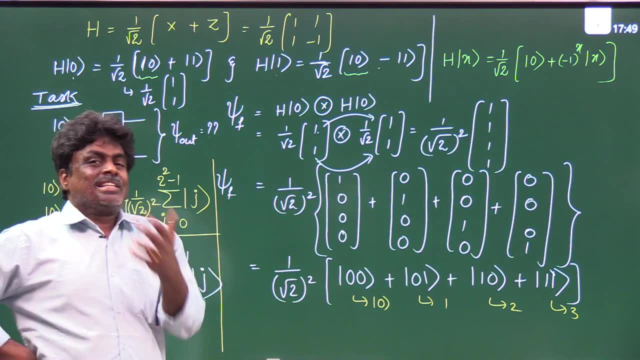 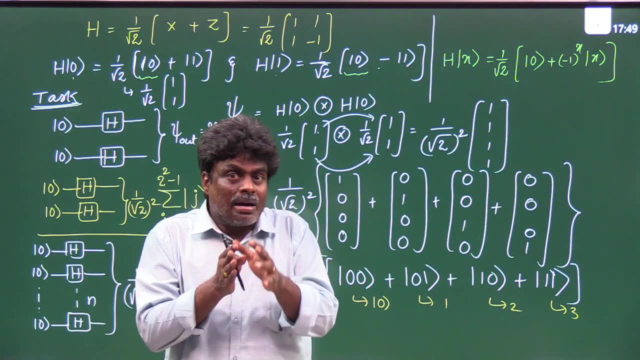 Something like that. So j That, j, That, j That j takes values from 0 to 2, power n minus 1.. Sir, what is this? You please tell me. what is this? Here you are observing Whenever you operate a Hadamard gate two times? 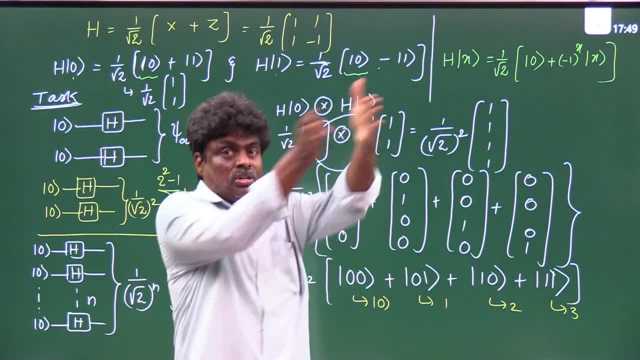 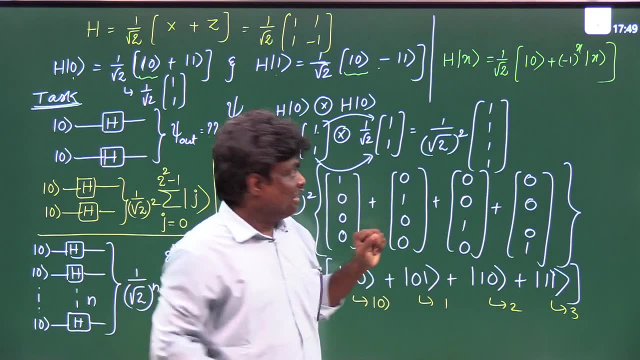 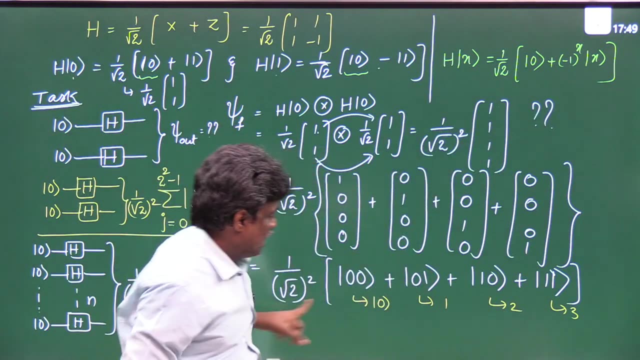 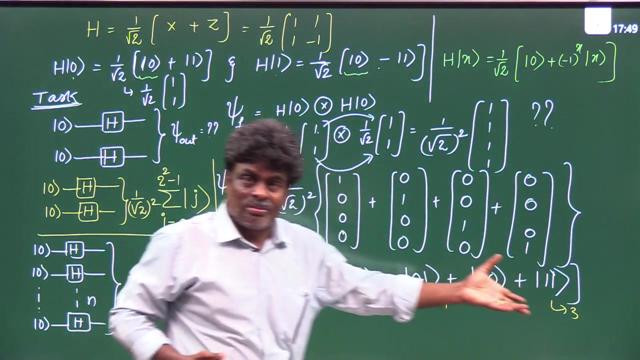 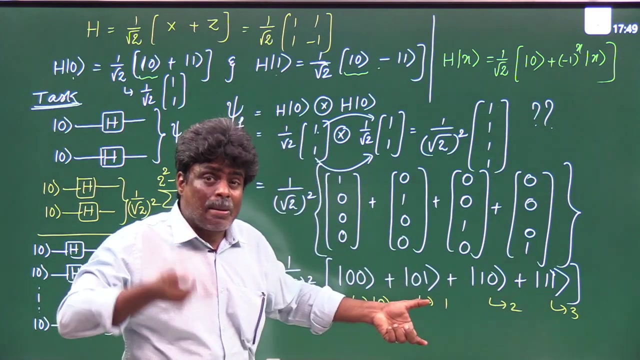 That means, sir, not two times Hadamard. Two Hadamard gates operates on two inputs, zero states. You got the final output as 1, 1, 1.. Now, what is this represent? actually, If you split it, finally, what you get? this is a linear combination of, and this is a linear combination of are simply array of all the numbers lying between. I repeat, this is simply an array of all the numbers lying between 0 and 3.. 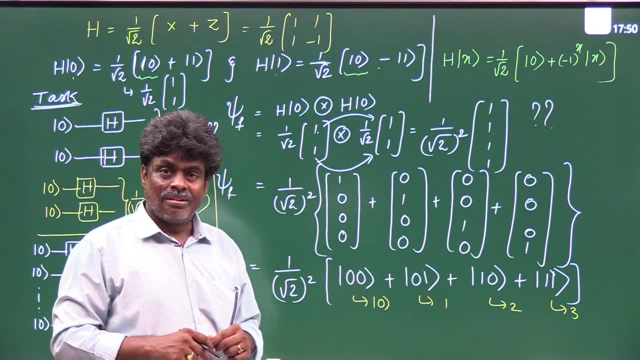 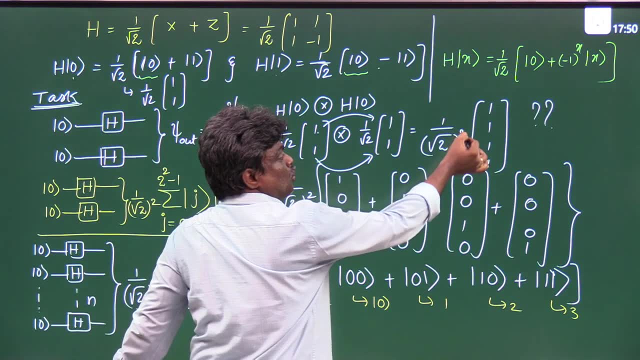 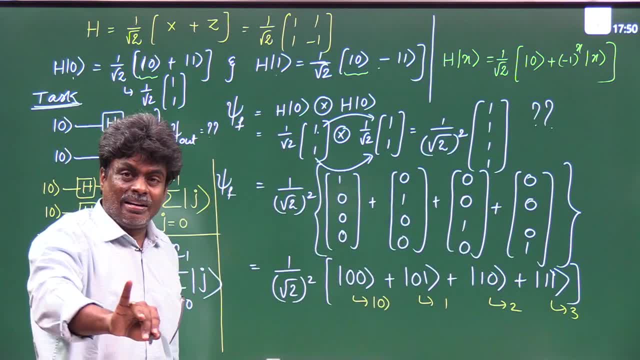 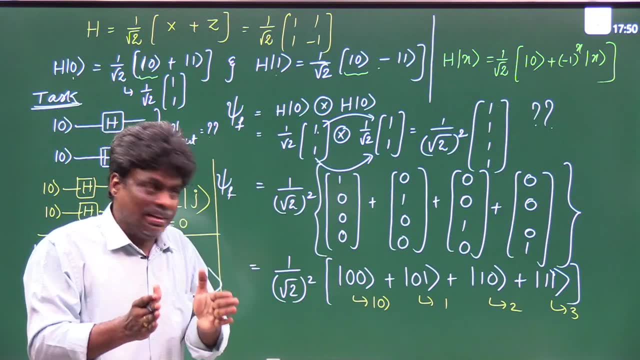 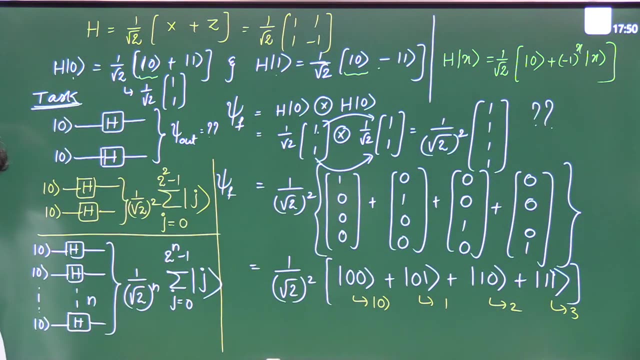 Like this. That is nothing, but It's a random number. It represent a random number Which lying between 0 and 2 power n minus 1.. 0 and 2 power n minus 1.. I don't know how many of you understand this. 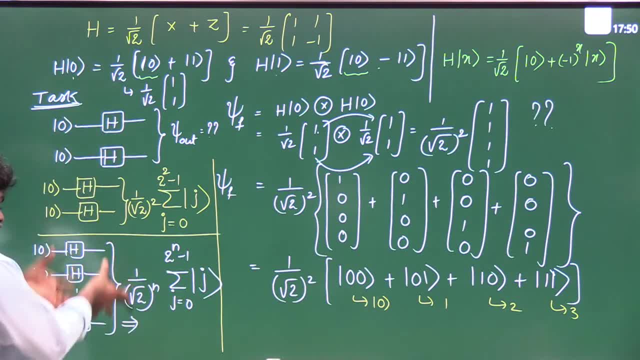 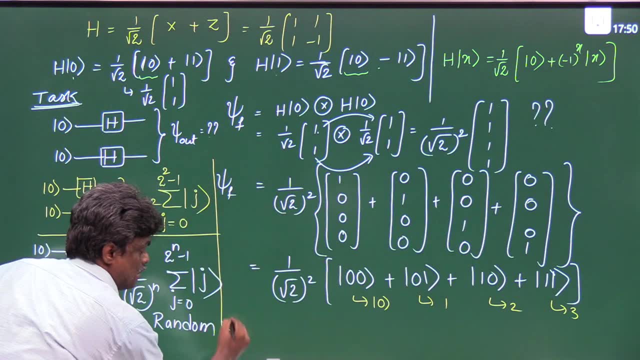 So this where they will use? I mean, what is the significance of this? This represent A random number in binary notation, random number lying between, lying between. here I have taken n operations. that's why 0 to 2 power n minus 1.. 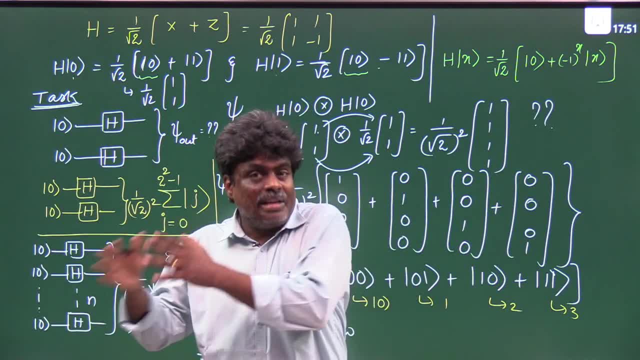 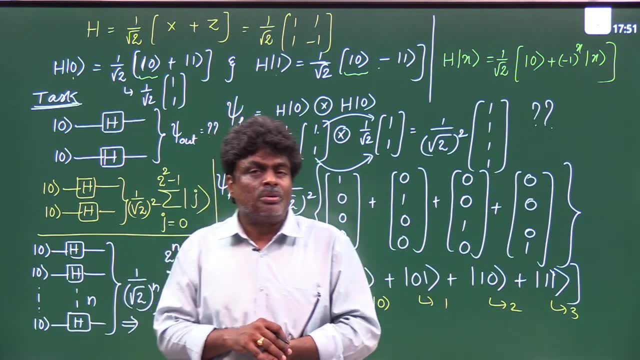 So what is this random number? When you are applying, then you will understand While you are studying the Grover's algorithm. definitely, we have to use this Because in the Grover's Algorithm what you will do Just like, we call it as finding a needle in the haystack. 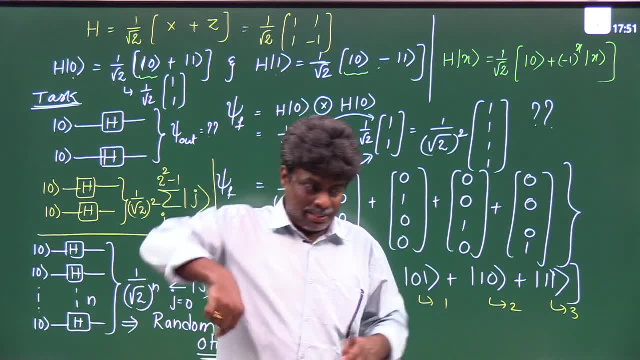 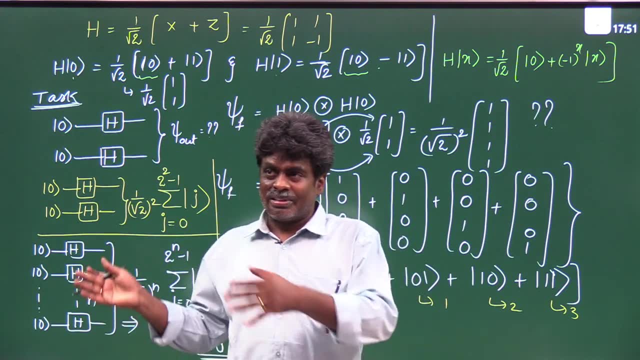 That means, for example, you lost one needle in the haystack. Haystack means in Telugu- I know, in English I don't know what you call Telugu- we call it, as some, that grass, that we will tie that, all the grass, something like that. 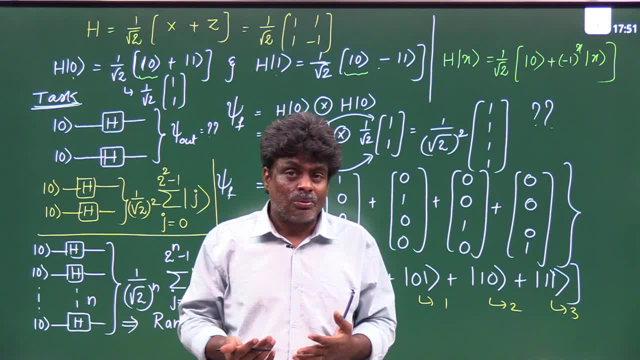 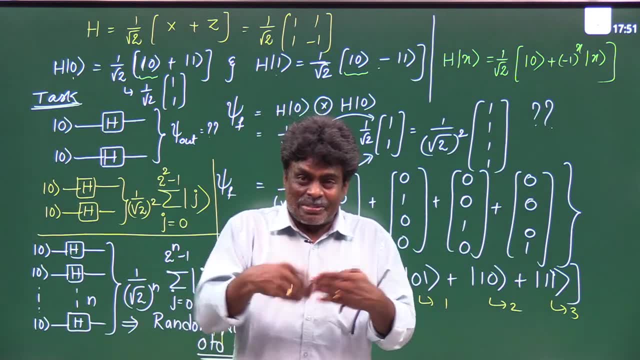 For example, you lost a needle in that, What you will do, Will you search for needle. Don't say I will put a magnet or something like that. Don't say I will put a magnet or something like that. So will you try to find the needle. 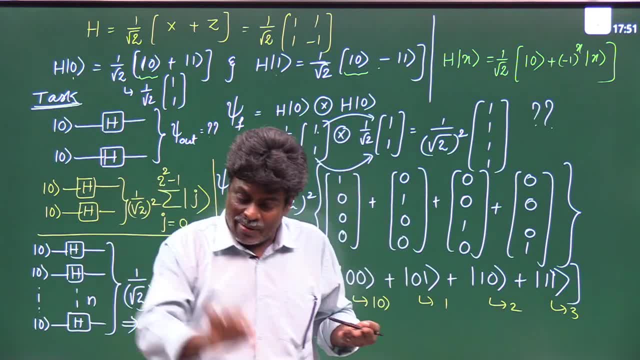 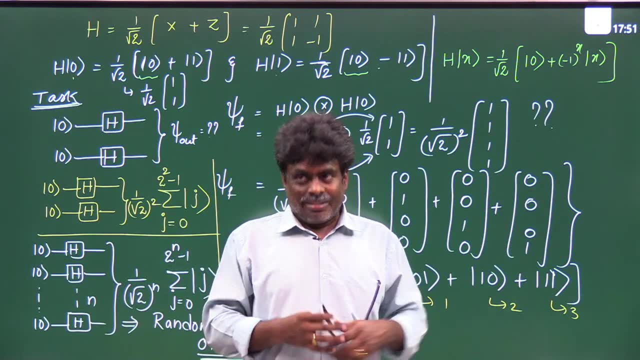 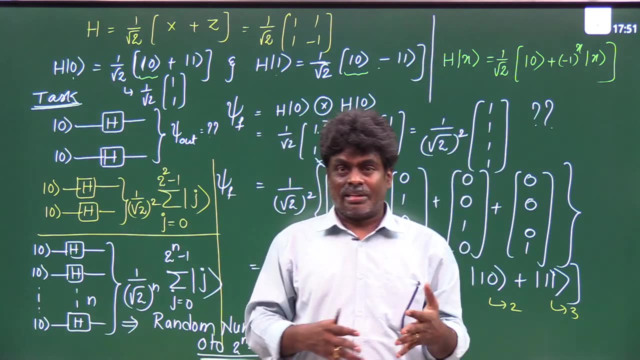 No, We will try to separate the one by one piece, like this. Then only we can find the needle Common sense. That means for example: you have some phone numbers. Some phone numbers are there In all over India. some phone numbers are there. 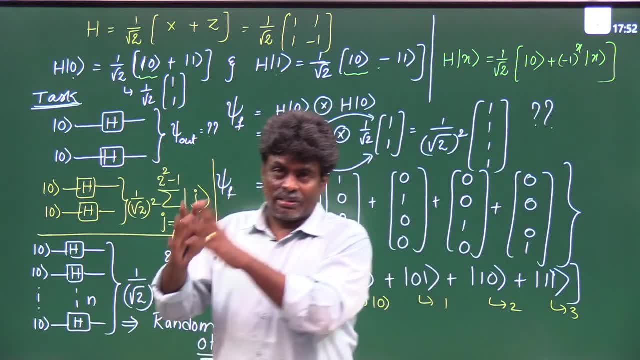 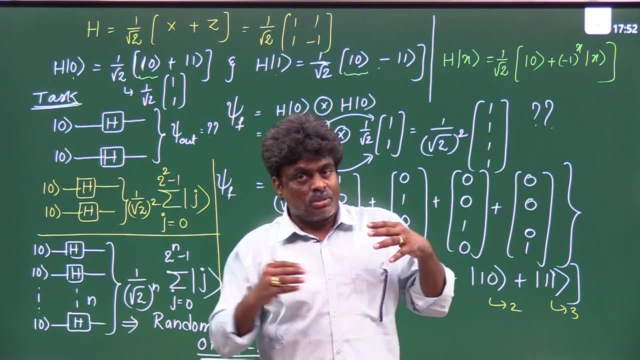 You want to know the phone number of Mr X. What you will do? You will write a program First. you will write, you will store all the phone numbers in an array, Generally programming. the basic idea is like this: 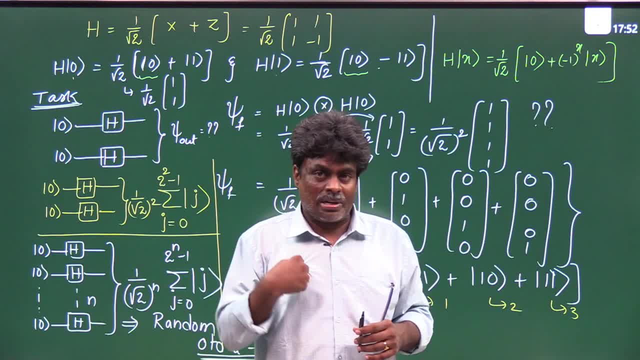 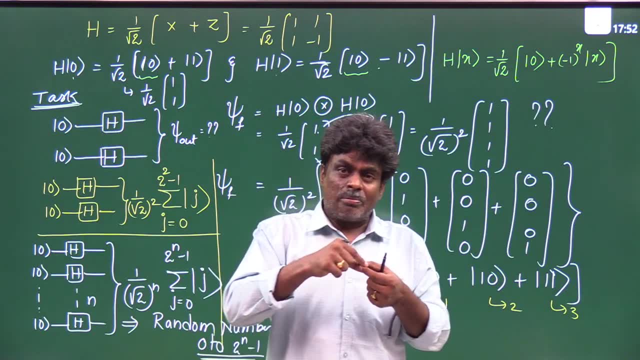 And you will give input as your phone number- unknown person phone number- And then you will search operation, Then this phone number will match with each and everything And finally it will give you the output. Mr Nageshwar Rao. 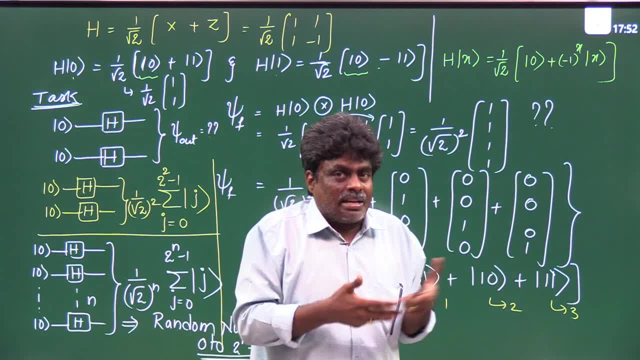 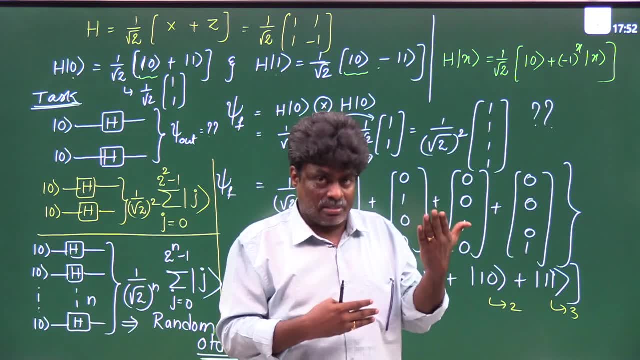 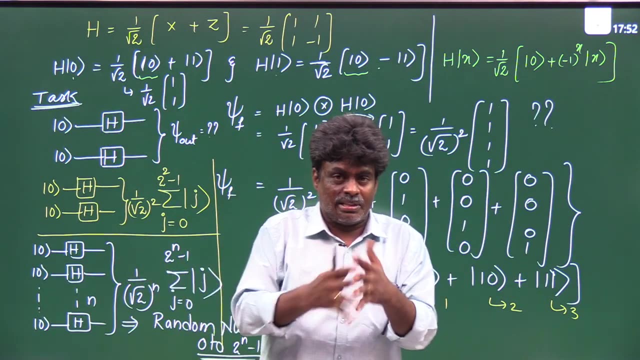 So this is what classical computer will do. I repeat, whenever you want to search for a phone number of- I mean name of- a person. if you have a phone number, you want to find his name. It's not like a robo-movie. the Rajnikanth say the phone number. 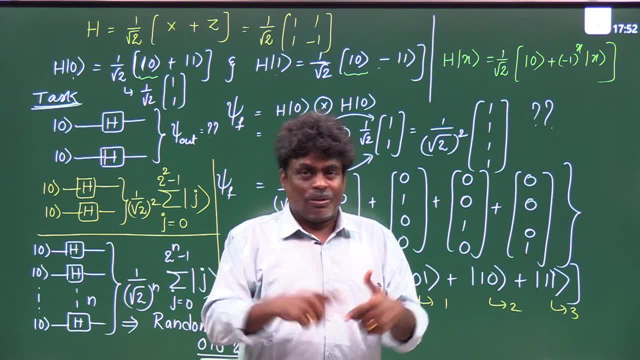 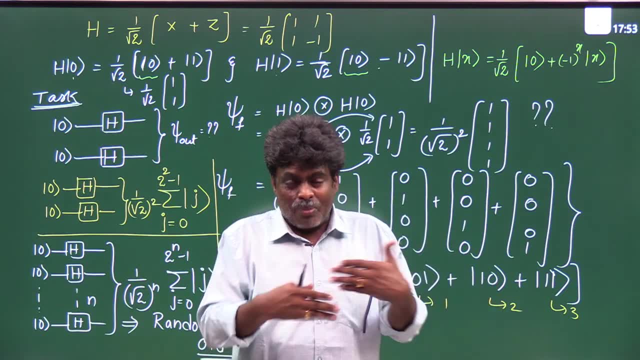 It's not like that. We have to search Now the computer also, classical computer also. it's just like a manual search only, But it will do fast. So what is the process actually? You will give all the phone numbers, data in an array. 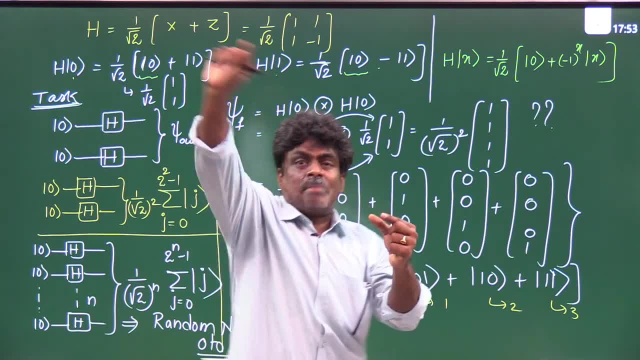 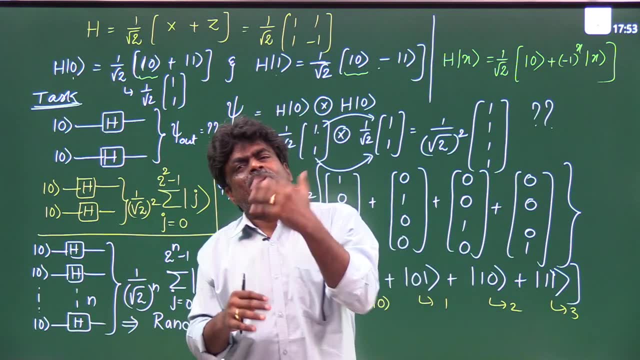 And you will give this input And it will search whether this is matching or not. matching or not matching or not. It will check one by one, one by one. For example, you have 10,000 phone numbers, 10,000 people, data. 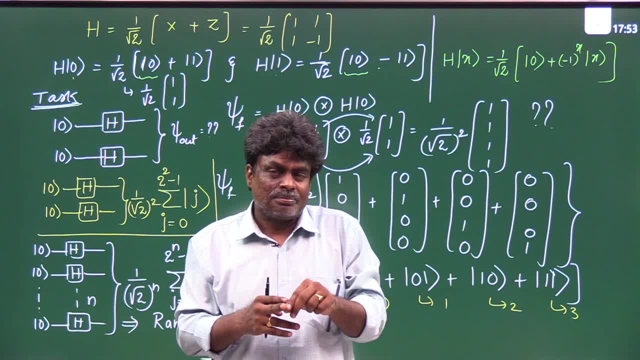 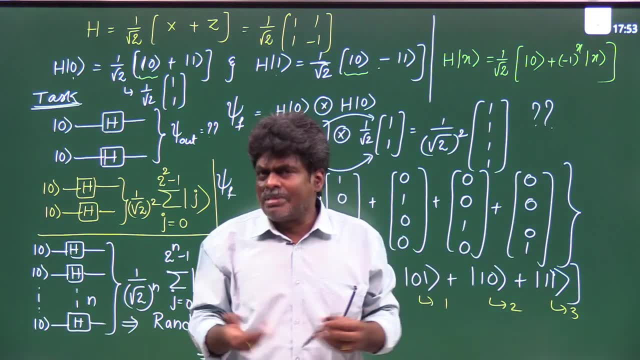 Now you are searching for Nageshwar Rao, Nageshwar Rao phone number. Then classical computer will do how many iterations, how many operations it will do. The common sense will tell you. Maybe first attempt you may get. 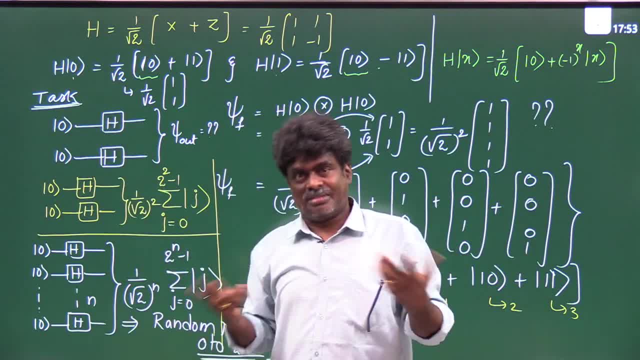 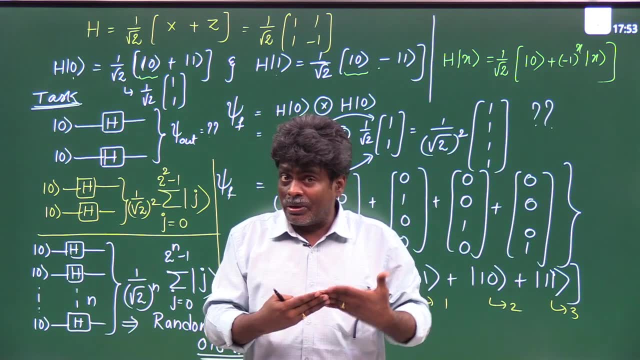 Yes, Or last attempt you may get Yes. That's why, on average, it has to do. I hope you understand what I am saying. The classical computer maybe first attempt we get, we don't know- Or last attempt, probability. 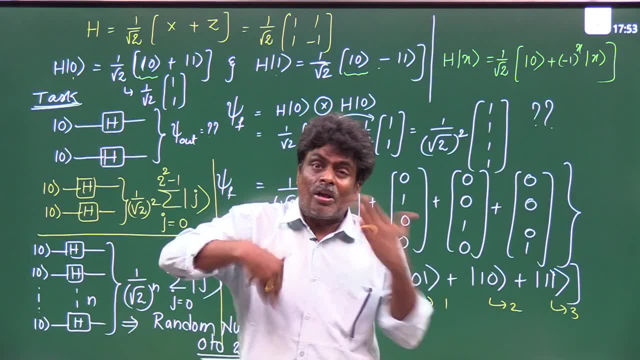 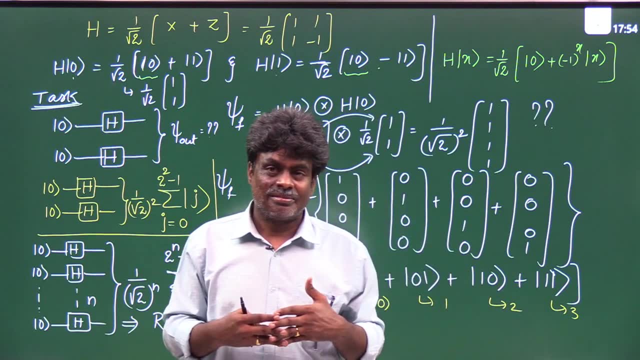 Last attempt, we also get On an average how many operations it has to do. Half of that, That is a 10,000 by 2. That is a 5,000.. But what? What is the algorithm is saying? 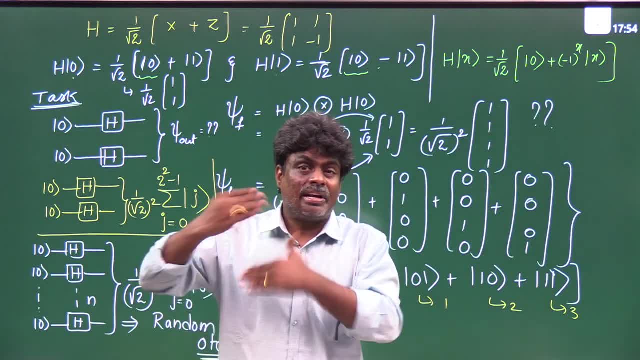 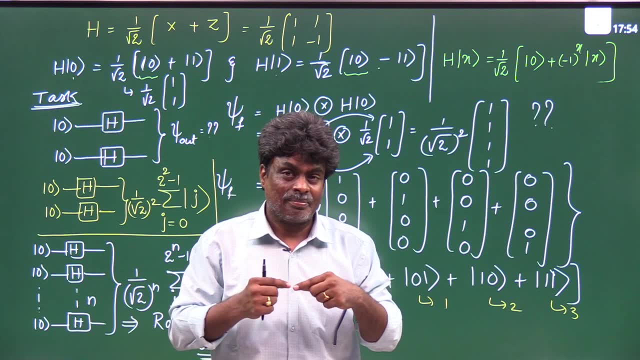 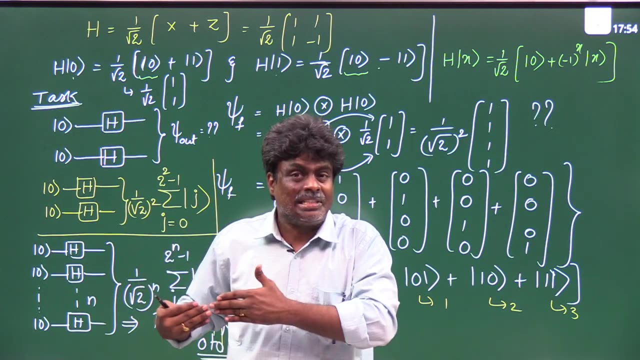 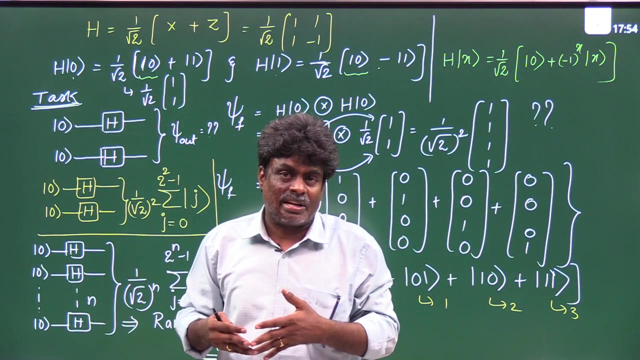 The classical computer is doing 5,000 iterations for finding a phone number out of 10,000 phone numbers. I hope you are understanding. The classical computer will do or perform 5,000 average operations or 5,000 iterations average for finding a phone number or search a phone number out of 10,000 phone numbers. data: 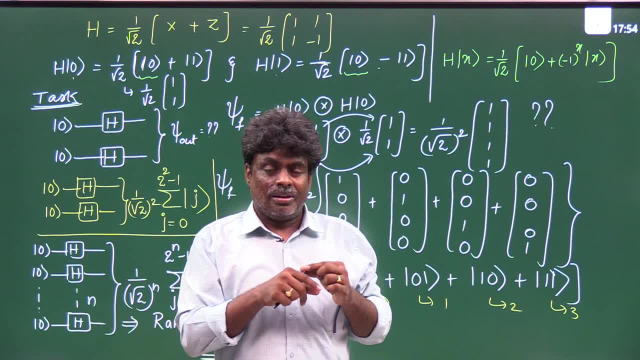 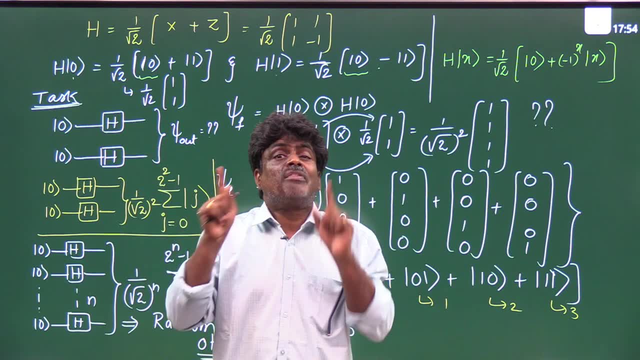 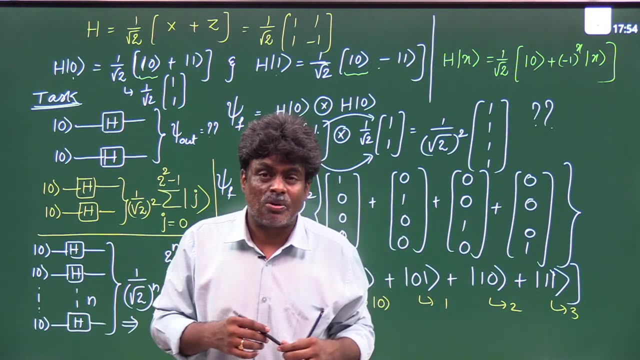 But what Grover's algorithm is saying? Yes, If you construct, if you build a quantum computer, it will perform only square root of 10,000.. Square root of 10,000, how much? Square root of 10,000, how much. 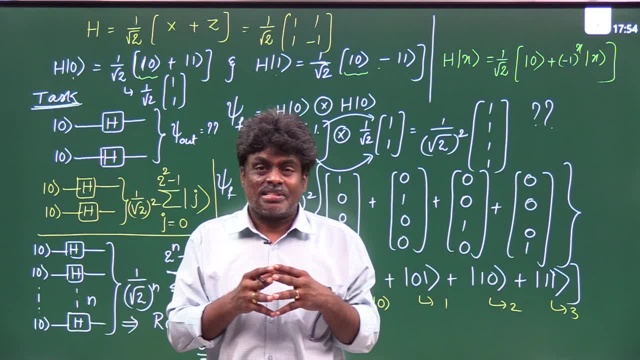 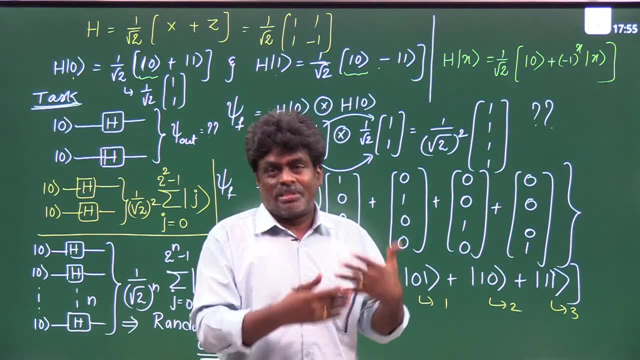 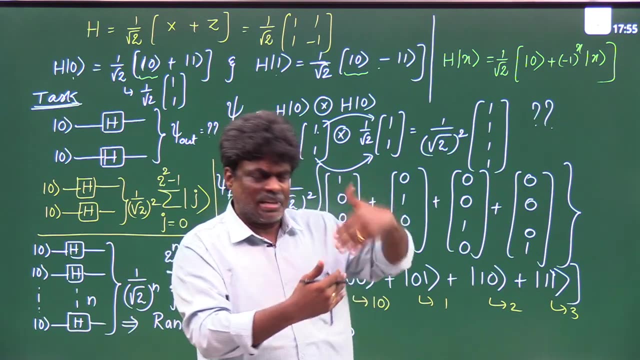 Okay, So that square root of 10,000 operations, That means how less it is. So that is a process. I mean that is a speed or whatever it may be. That is the nature of quantum Quantum. what do you say? quantum iteration or quantum process, whatever it may be. 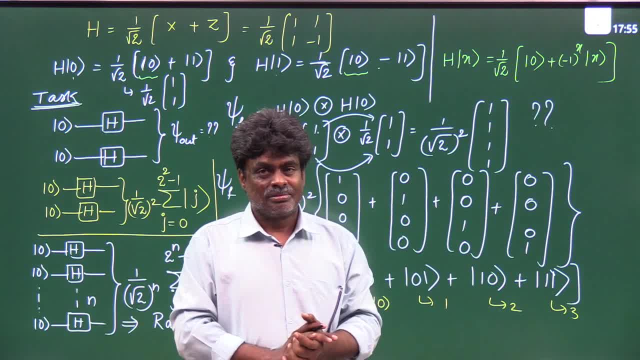 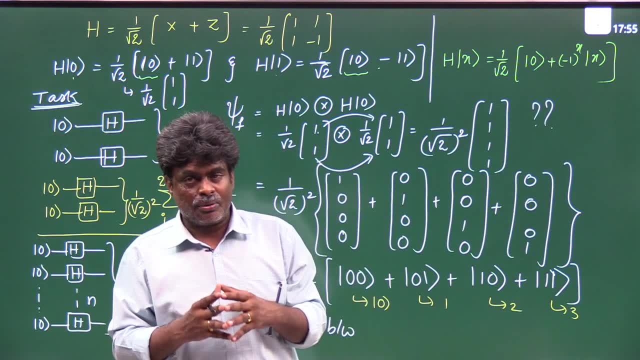 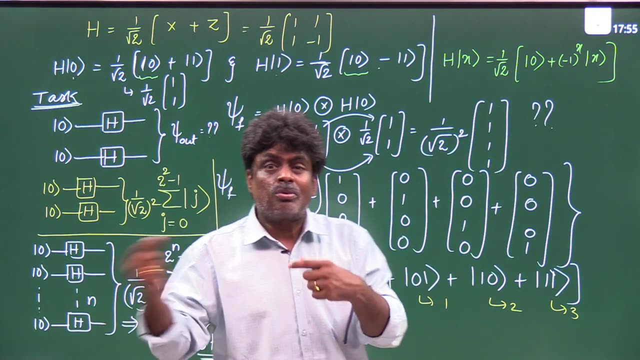 That is the difference between classical and quantum. So it will perform only under root n. Under root n operations That we will discuss more clearly. No problem, Grover's algorithm, we will discuss. So anyhow, in that Grover's algorithm I told you we have to store something or we have to give some random number. 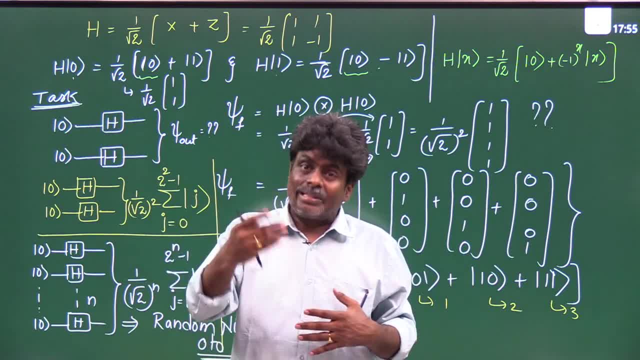 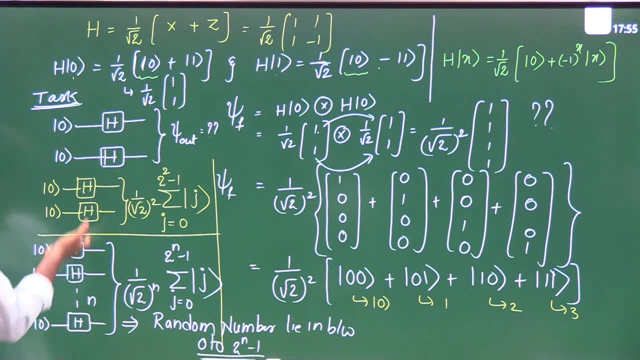 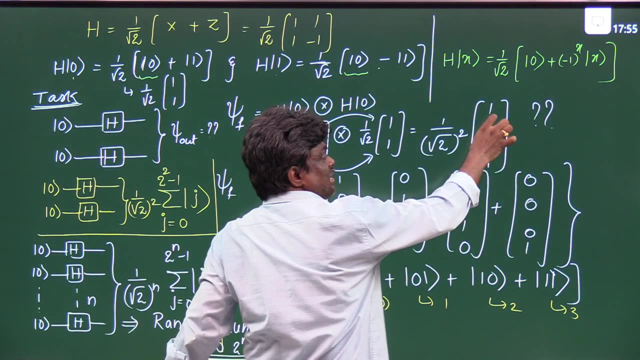 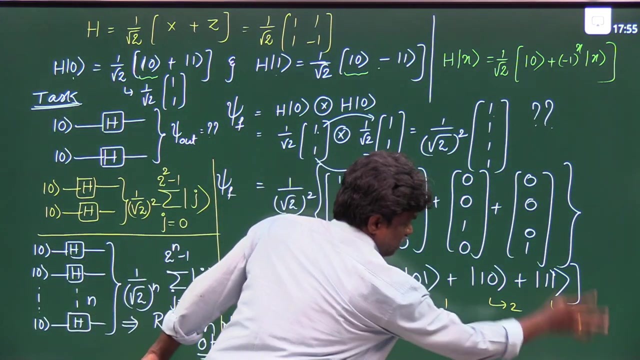 We have to give some random number To get the random number. we will use this concept, That is, if you operate these Hadamard gates n, Hadamard gates on n, 0 bits, Whatever the state, you are getting, this represent a random number lying between lying, between lying between 0 and 2, power n minus 1..